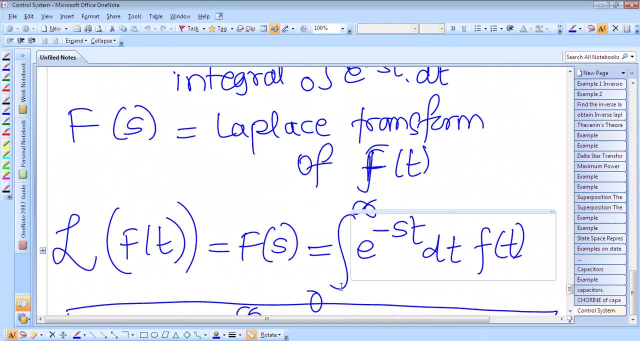 And therefore f of s is the Laplace transform of the function f of t And therefore, finally, we have to obtain the Laplace transform of: f of t is nothing but f of s. 0 to infinity, e, raised to power minus S, t, dt, into f of t. 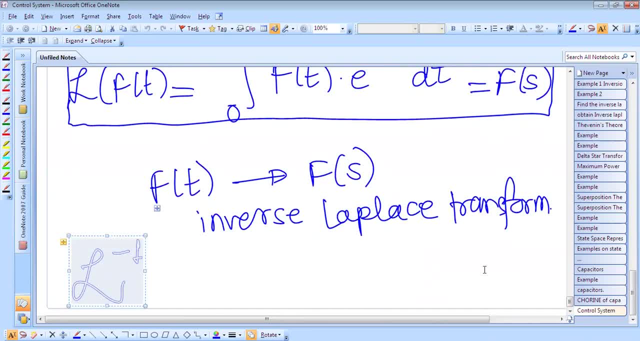 And we have got this Okay. So this is the f of t, So this inverse Laplace transform. Okay, So the reverse process of finding the time function f of t From the Laplace transform f of s is called as the inverse Laplace transform. 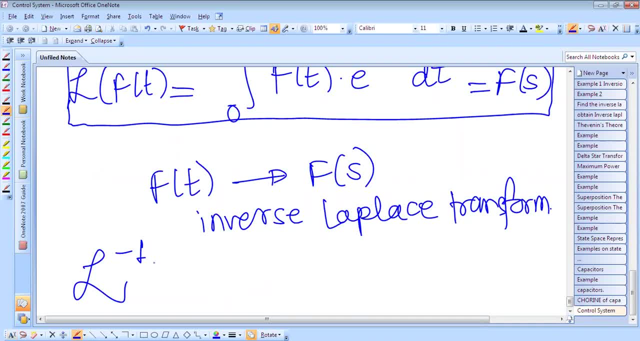 Therefore the operational symbol is used: L raised to power minus 1.. And this is f, of s is equal to f, of t is equal to 1 over 2 pi j. We have already seen this in signals and system. Okay, How to find the Laplace transform. 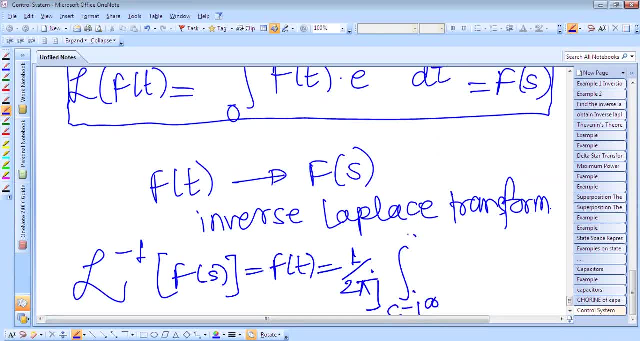 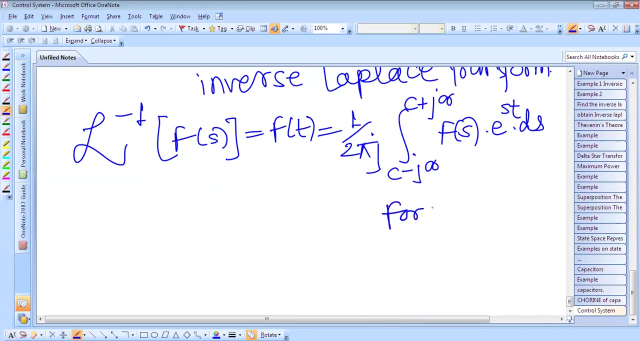 We will not go into the detail. So c minus c minus j infinity to c plus j infinity, And this f of s into e, raised to power S t into ds. So this is the inverse Laplace transform And this is for the t is greater than 0.. 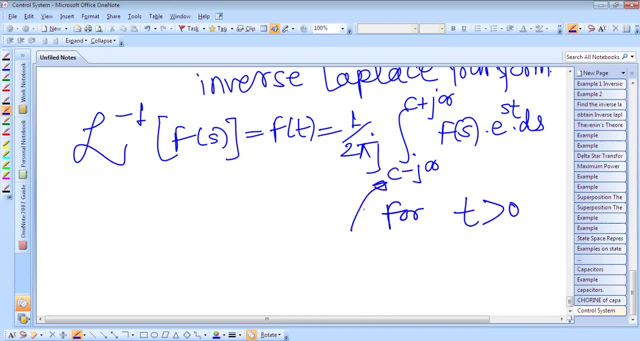 So where this c, this c is nothing but the abscissa of convergence, And it is a real constant. c is the abscissa of convergence and it is a real constant, And it is chosen larger than the real part of the singular points of f, of s. 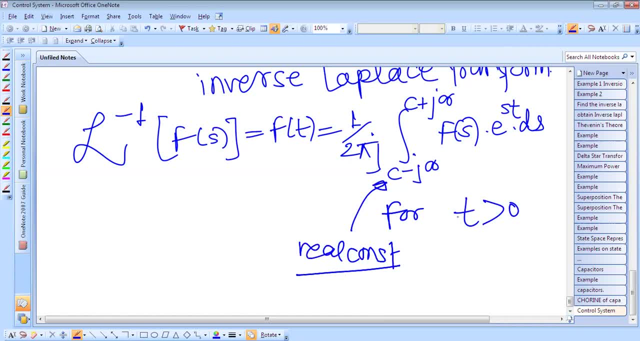 And thus the path of integration is parallel to the j omega axis. So this path of integral, this is parallel to the j omega axis. That means imaginary axis, And it is displayed by the amount c. Okay, This is the. c is the real part from it. 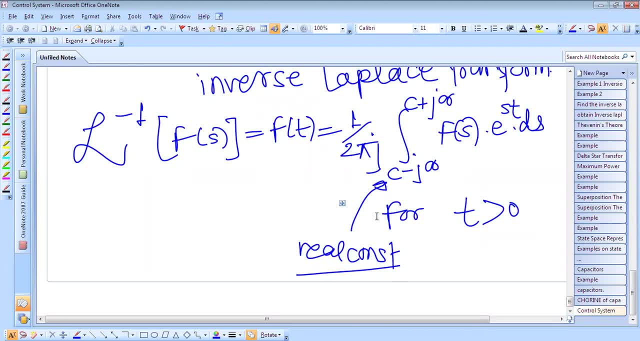 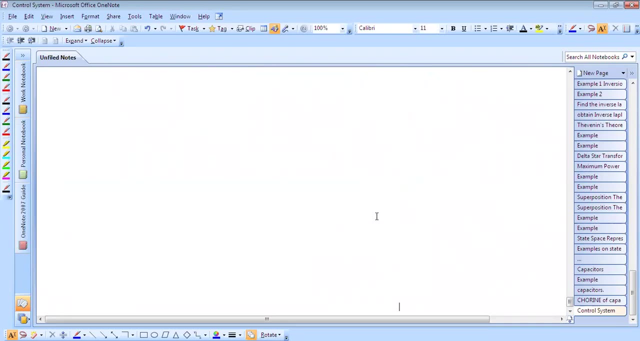 Therefore, the path of integration is the right of all singular points. Okay, So next we will discuss the mathematical modeling of the dynamic system. This is the very basic step for the analysis of the control system. This is the very basic step for the analysis of the control system. 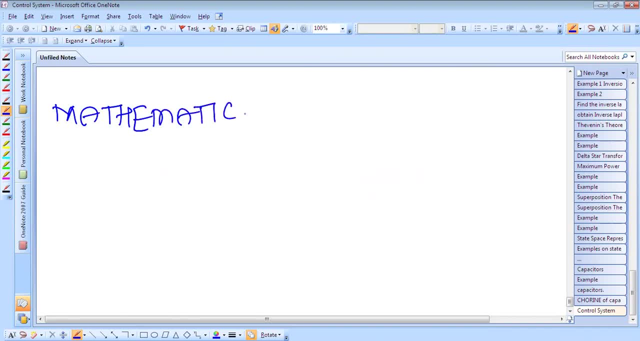 Okay, This is the very basic step for the analysis of the control system. So this is the very basic step. So now we will discuss the analysis of the control system. for the analysis of control system: ok, what do we in this method, here, in studying, 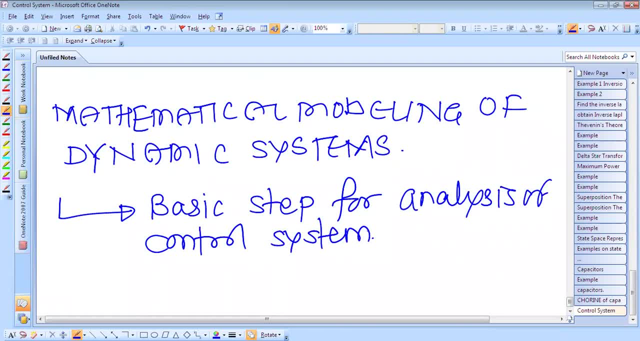 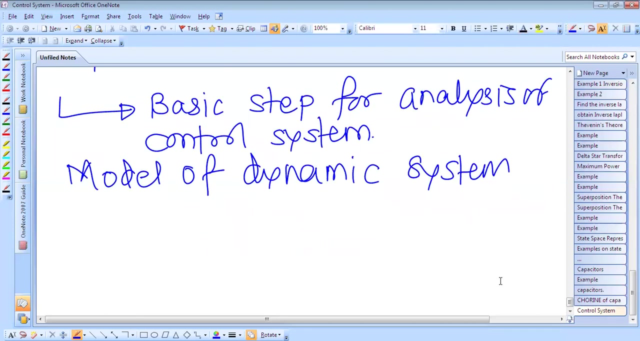 the control system, the. we have to develop the model of dynamic system. we have to develop the model of the dynamic system, model of dynamic system and once you develop this model of dynamic system and we have to analyze the dynamic characteristics, ok, model of dynamic system and analyze dynamic characteristics. 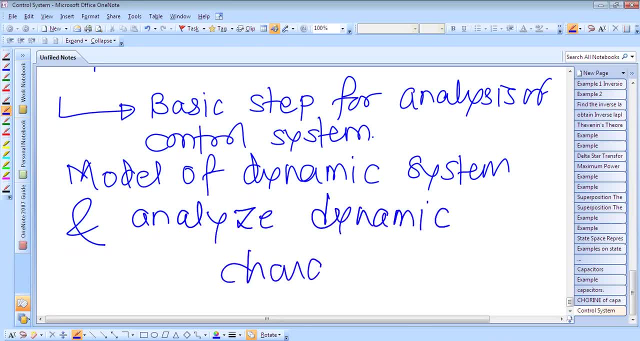 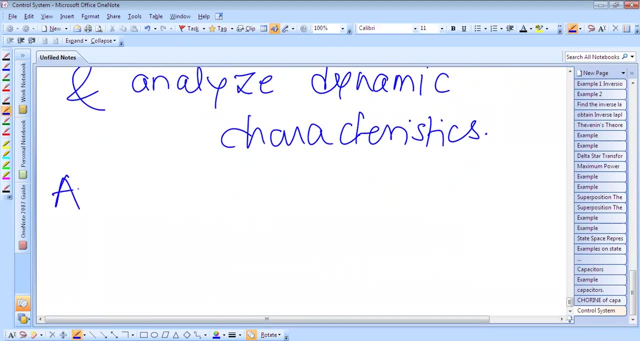 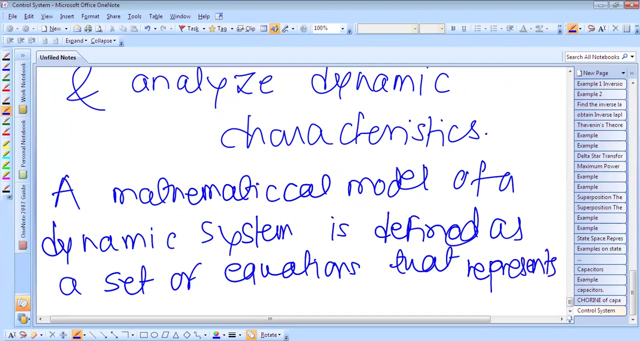 ok, we have to analyze dynamic characteristics of the dynamic system. so mathematical model of the dynamic system is defined as a set of equation. what is mathematical model? see, a mathematical model of a dynamic system is defined as a set of equations that represents dynamics of the system. is defined as a set of equations that represents dynamics of the system. 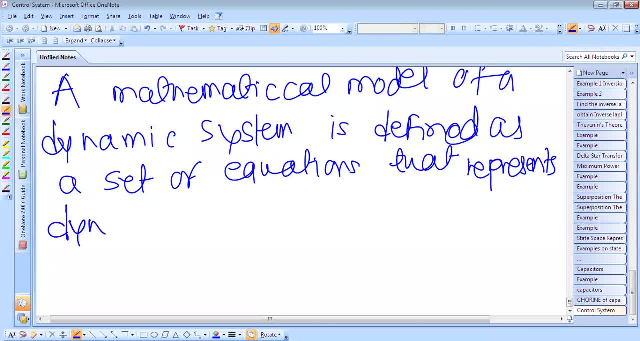 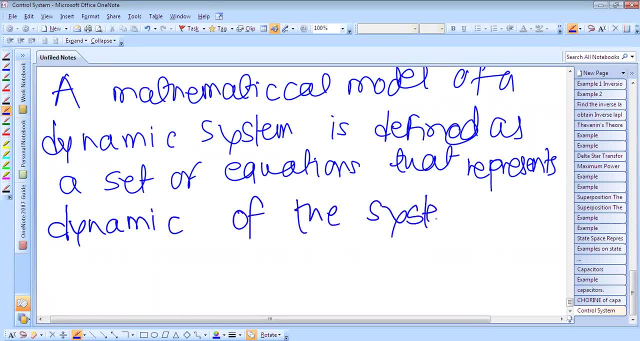 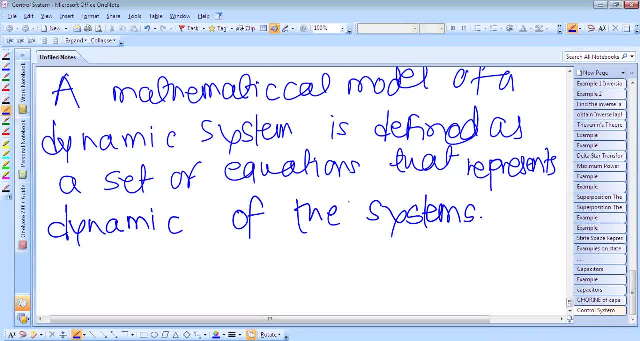 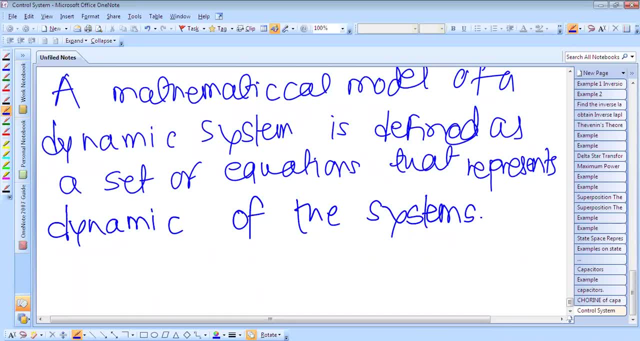 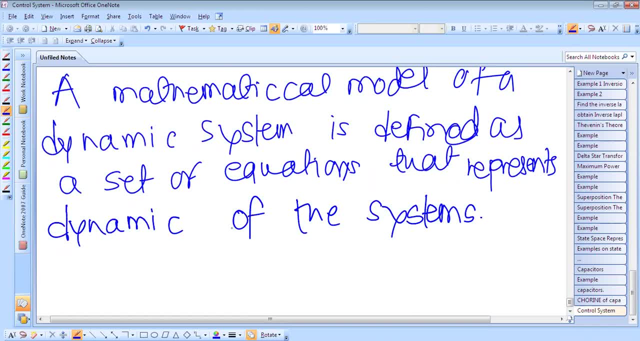 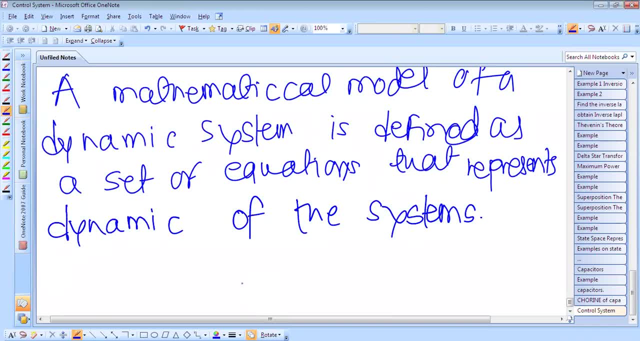 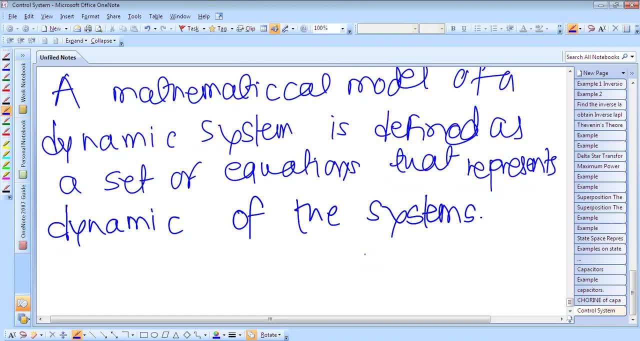 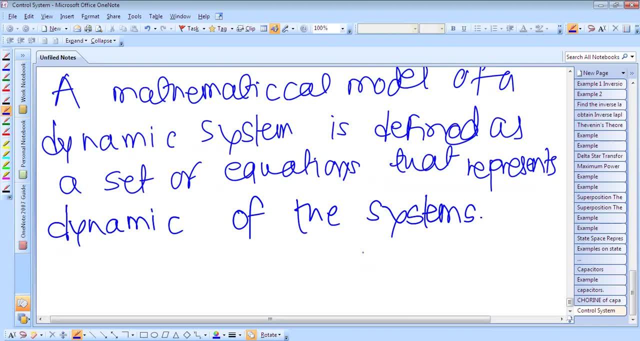 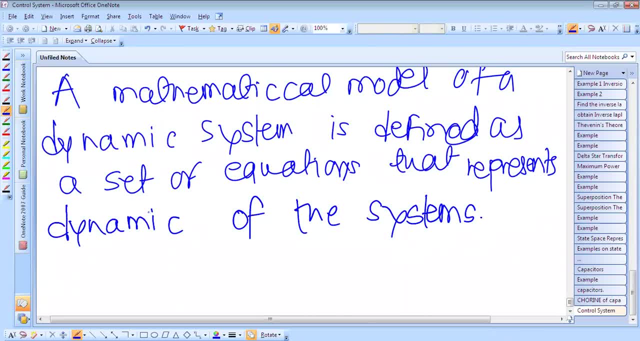 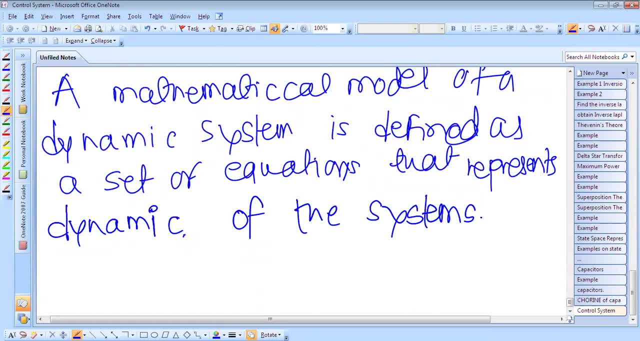 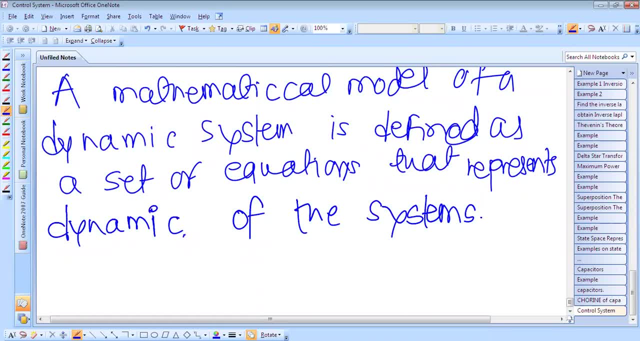 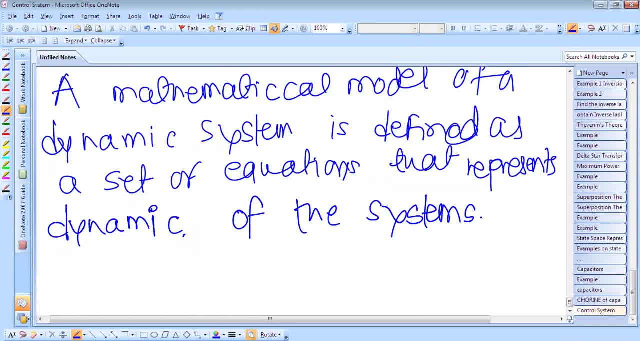 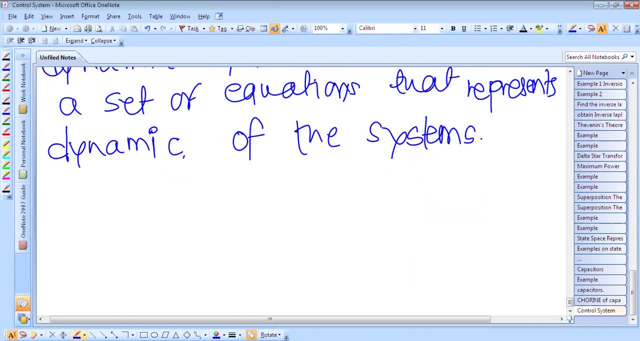 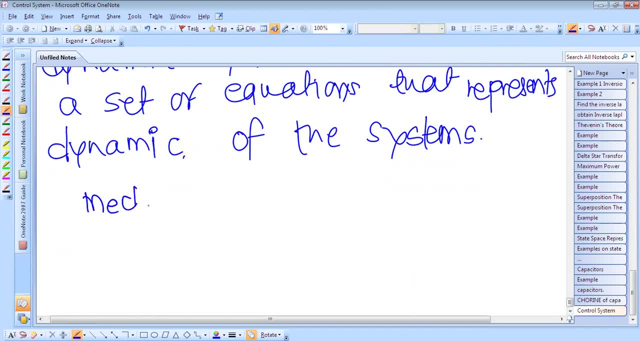 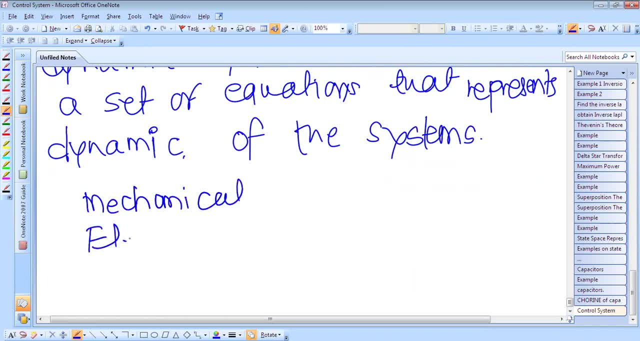 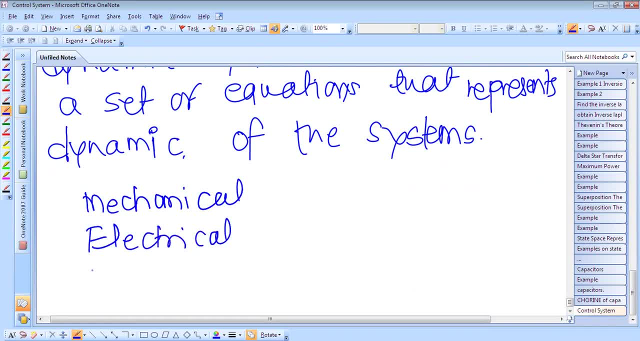 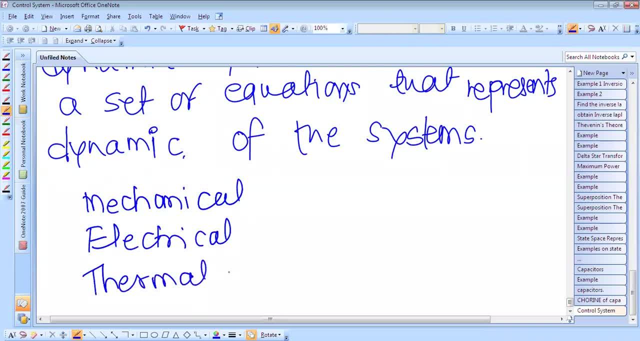 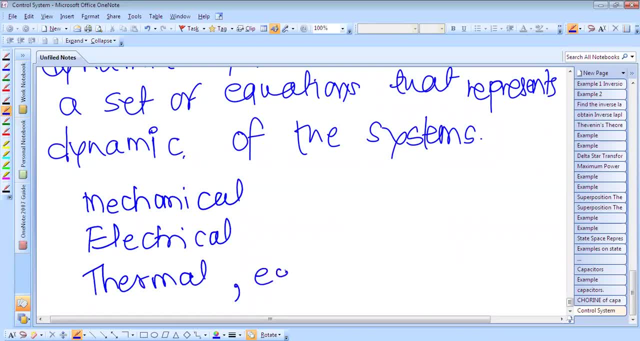 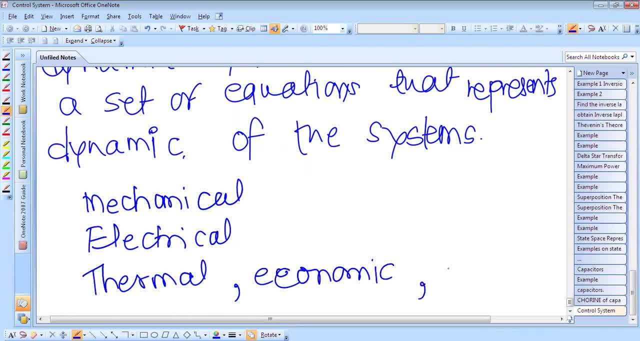 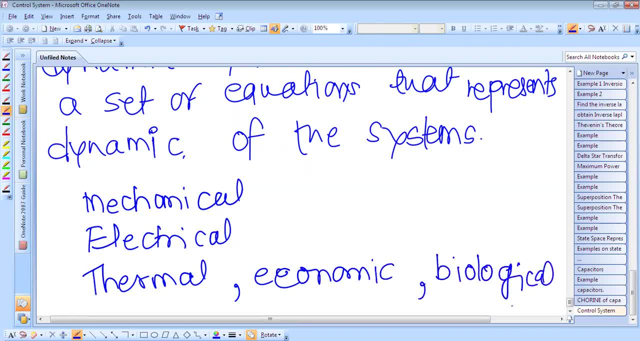 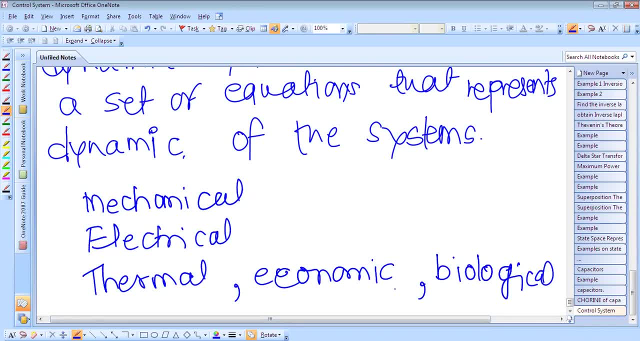 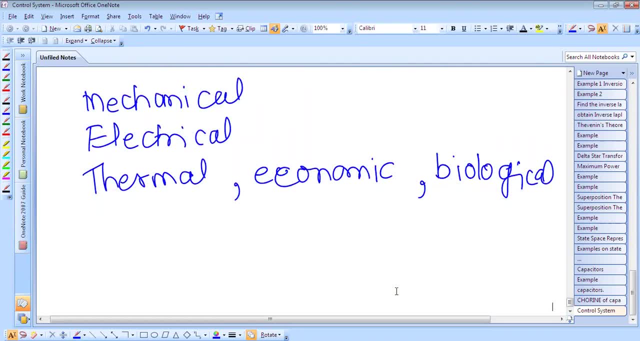 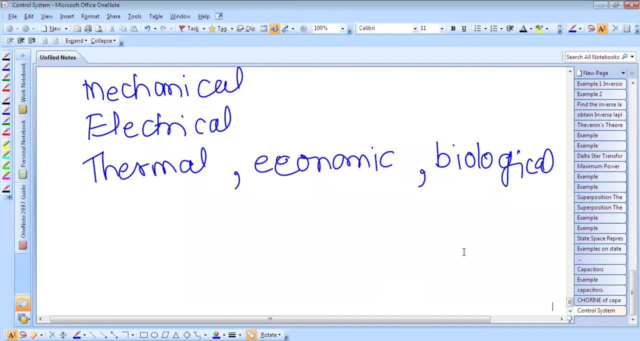 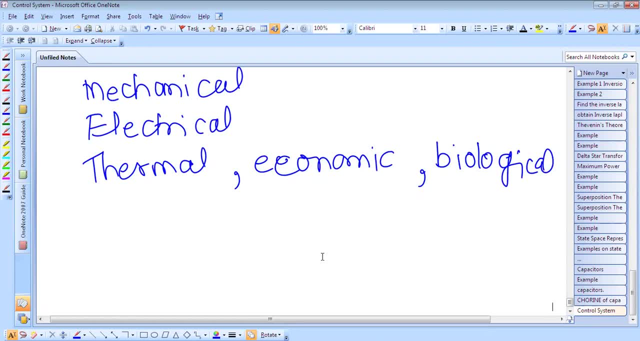 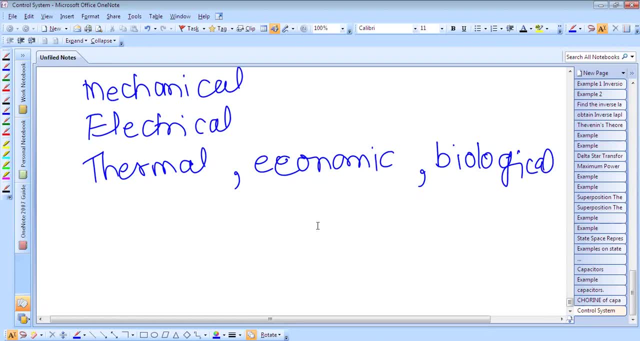 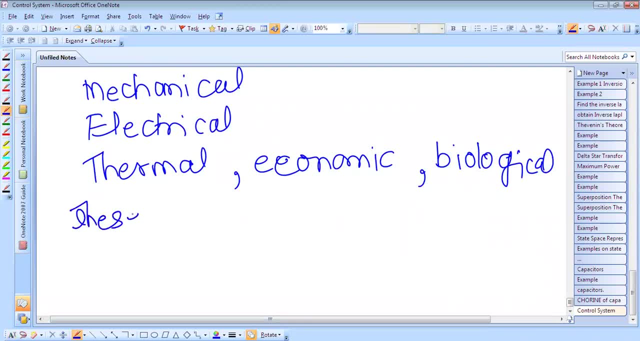 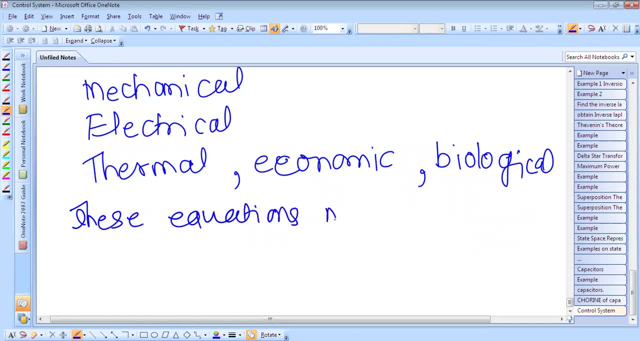 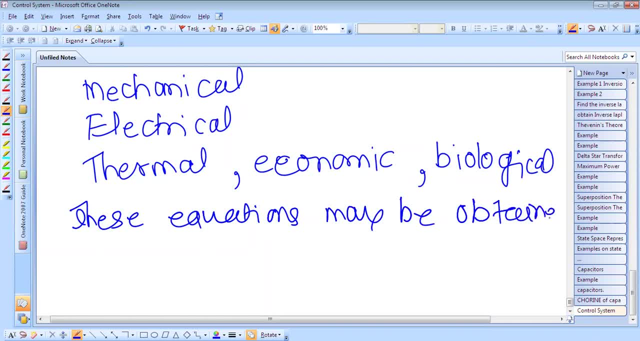 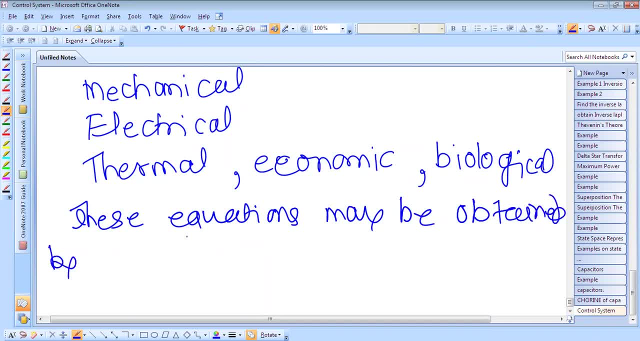 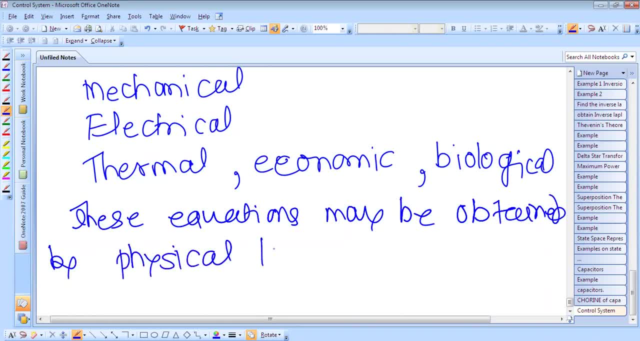 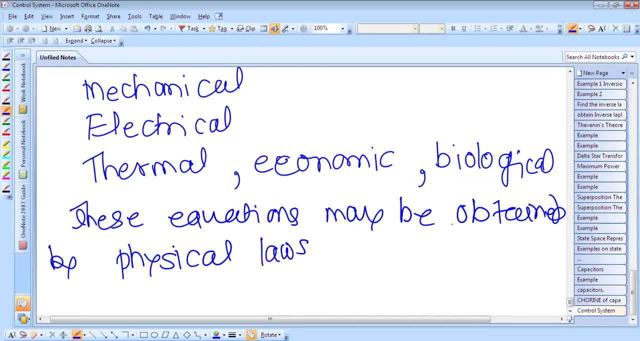 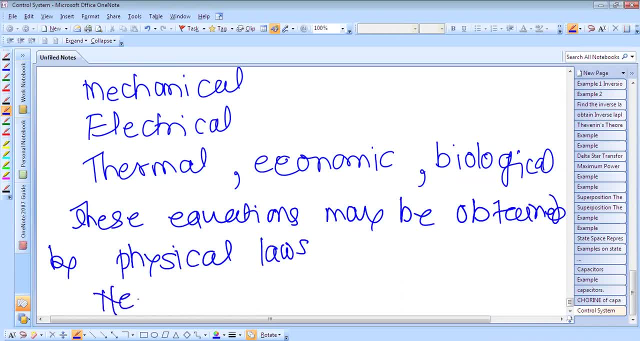 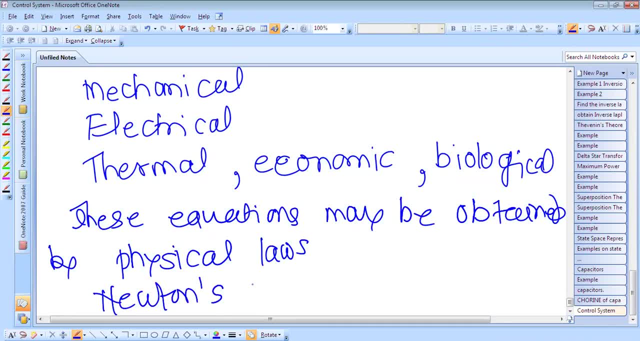 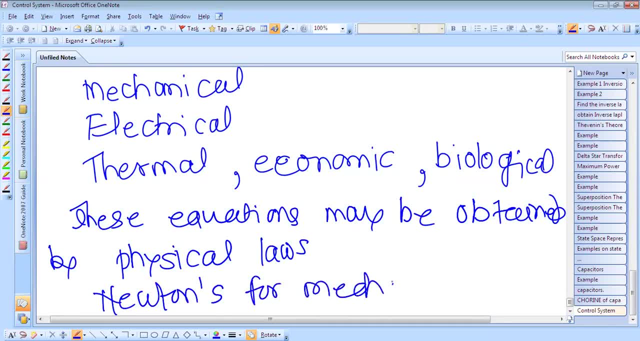 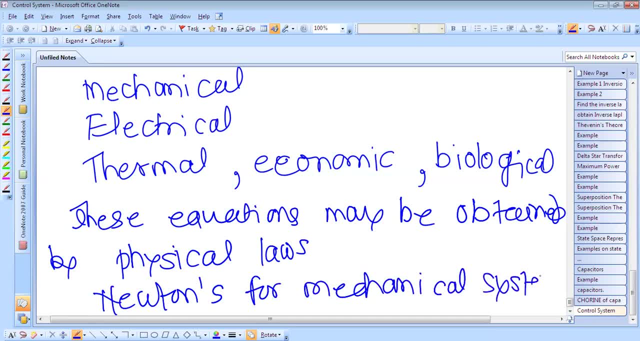 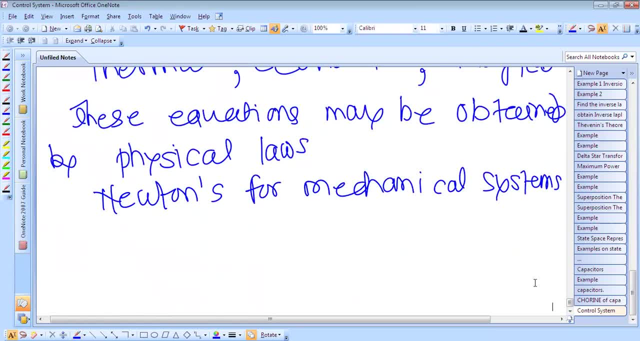 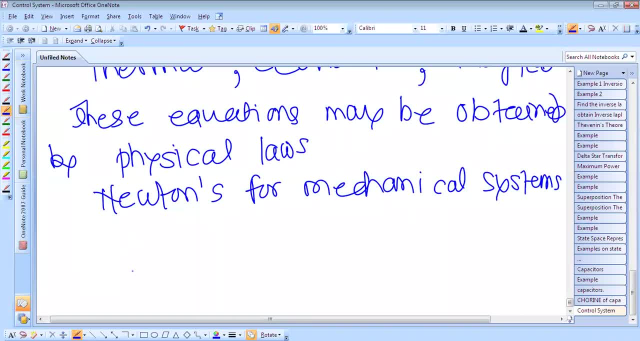 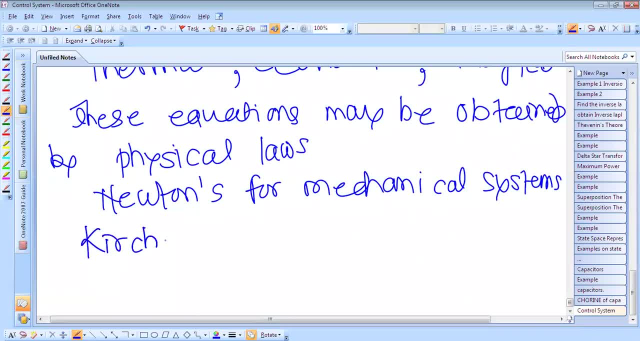 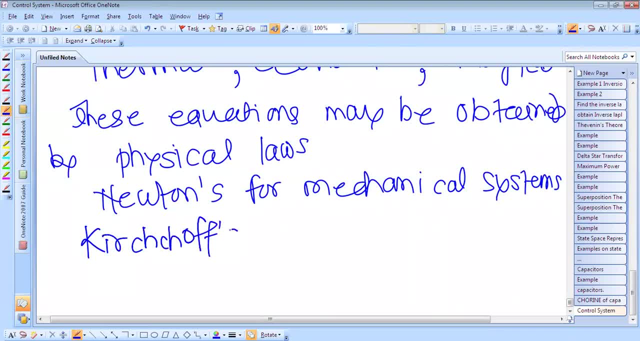 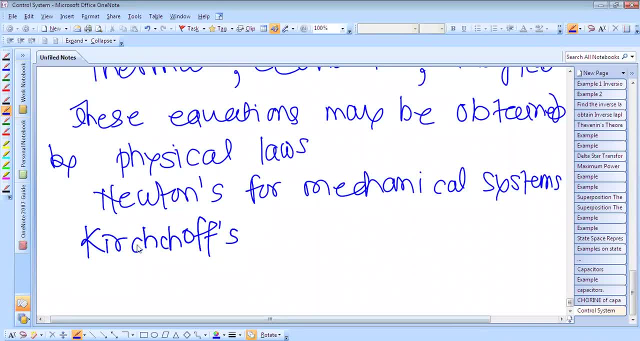 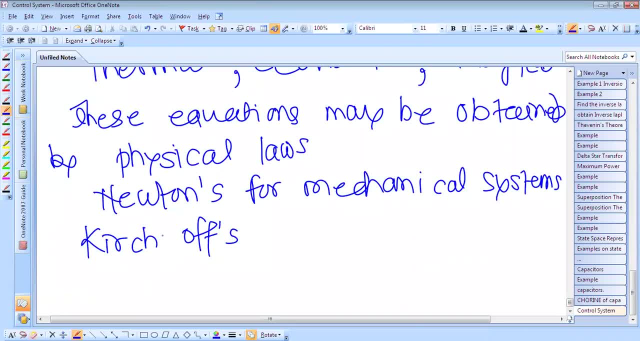 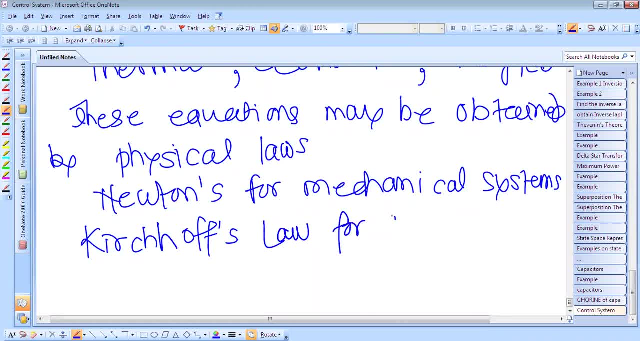 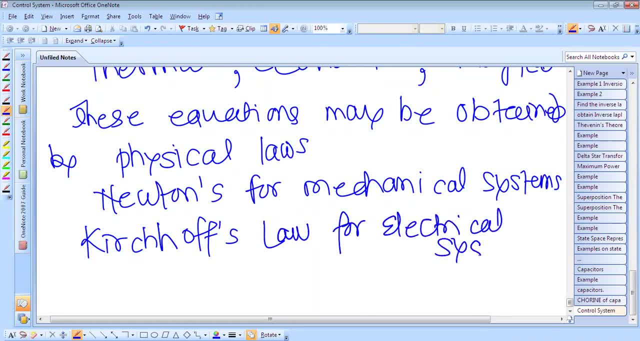 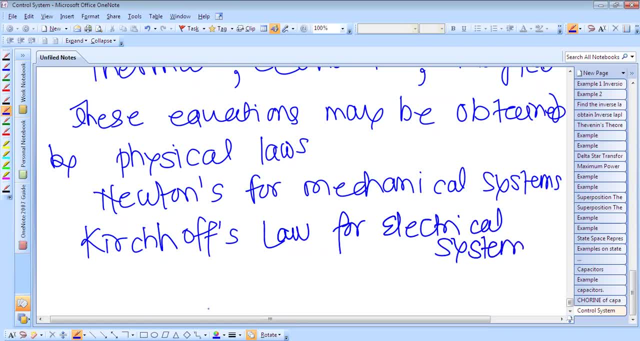 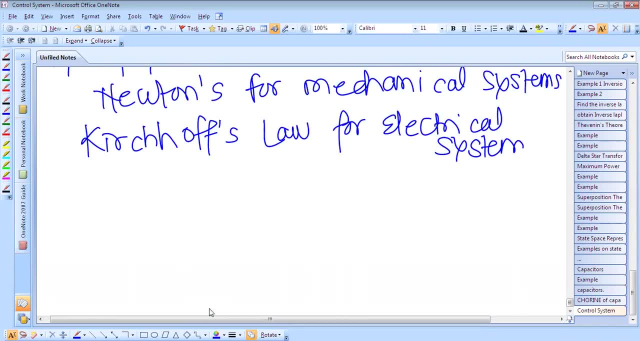 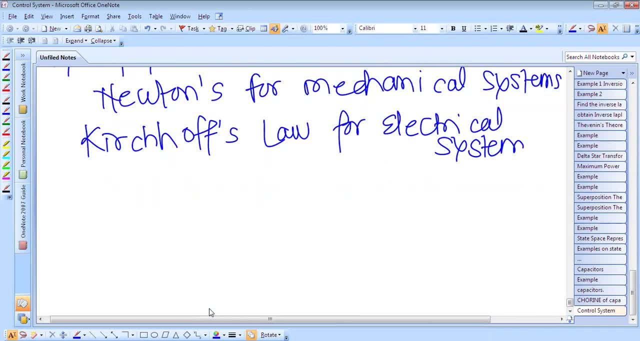 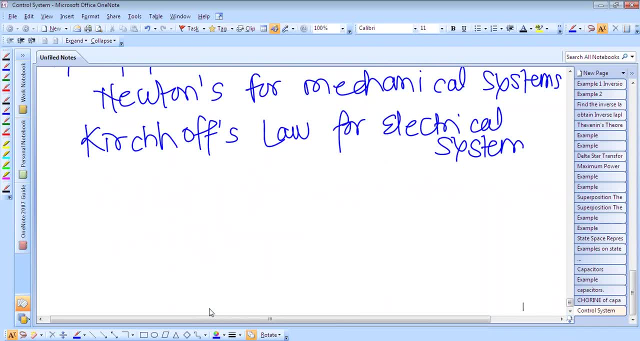 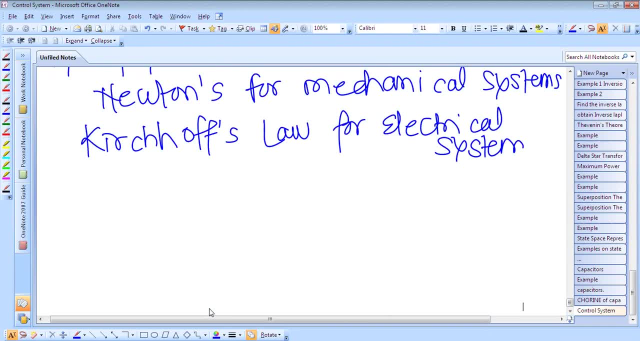 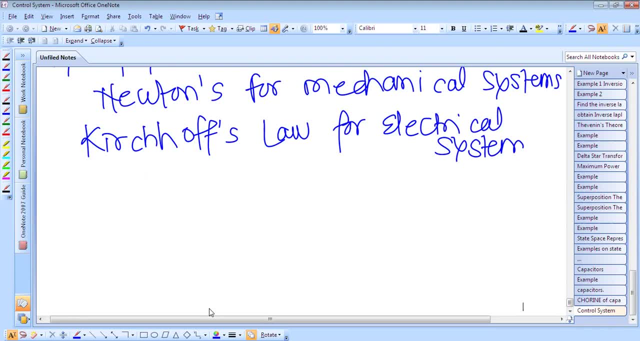 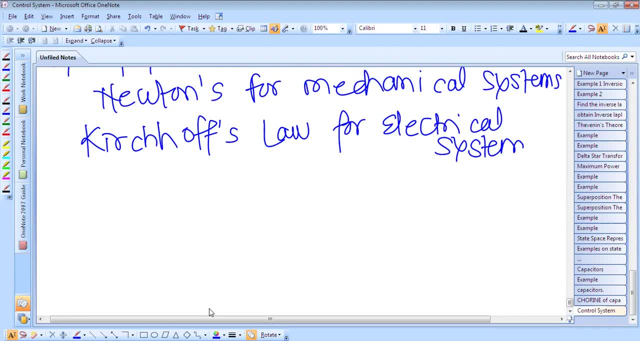 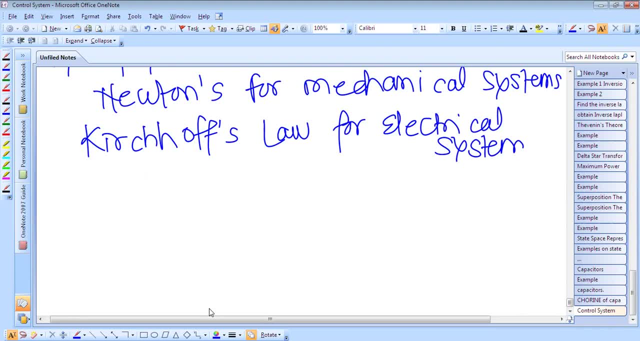 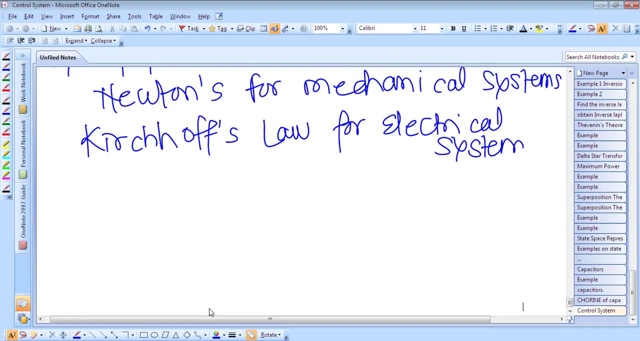 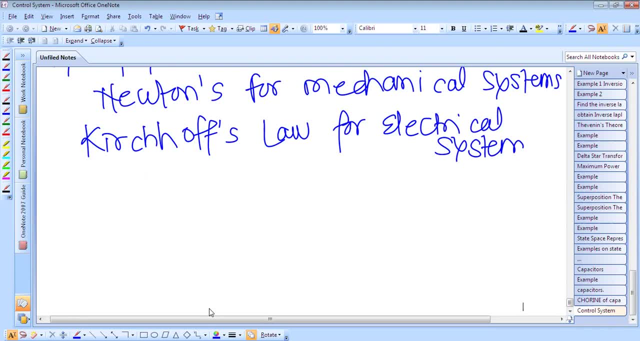 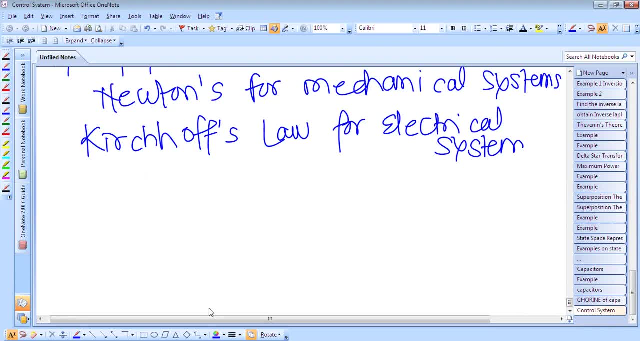 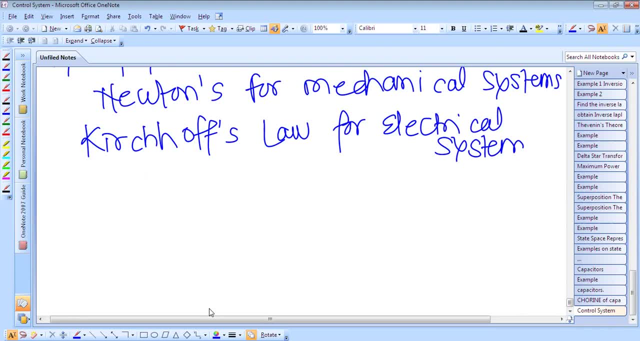 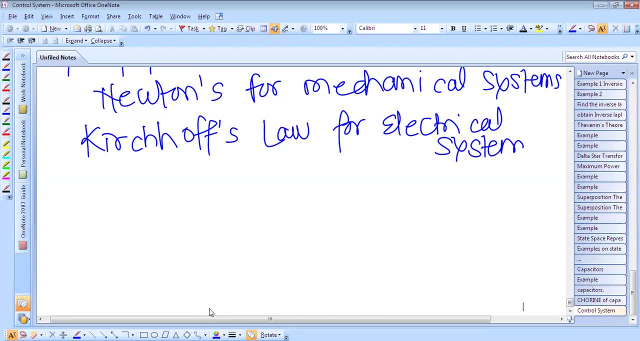 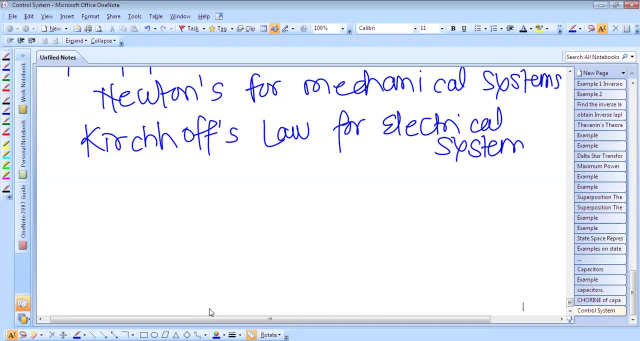 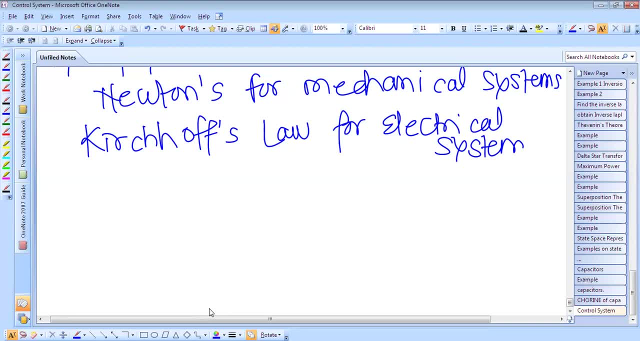 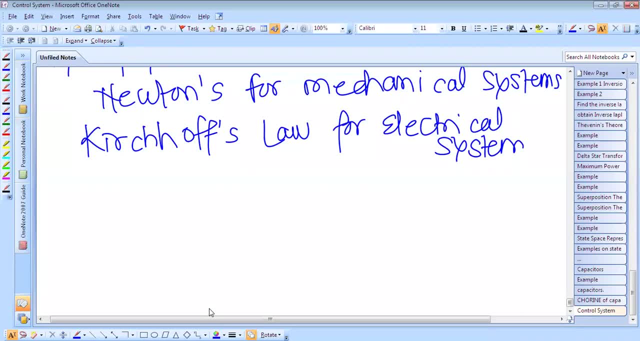 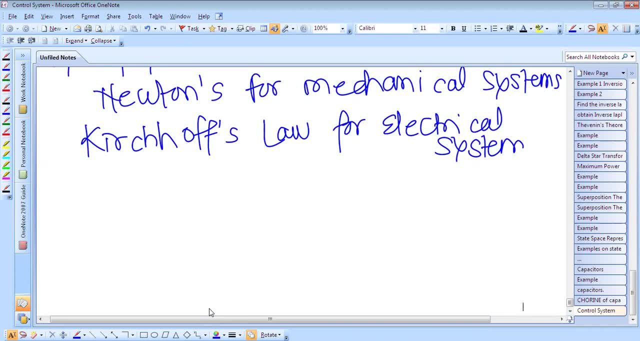 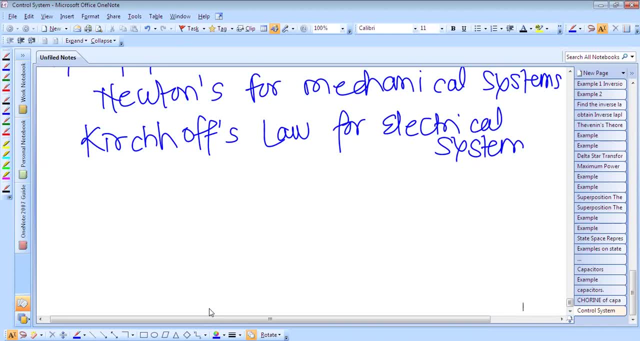 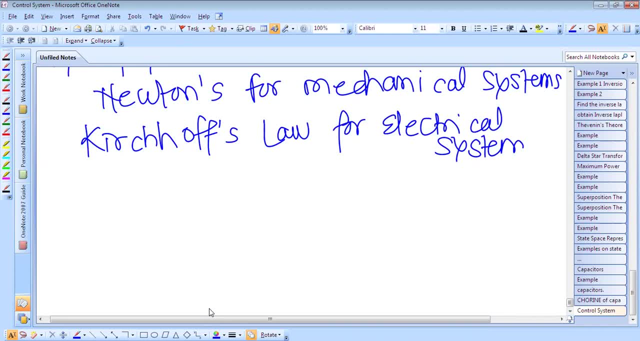 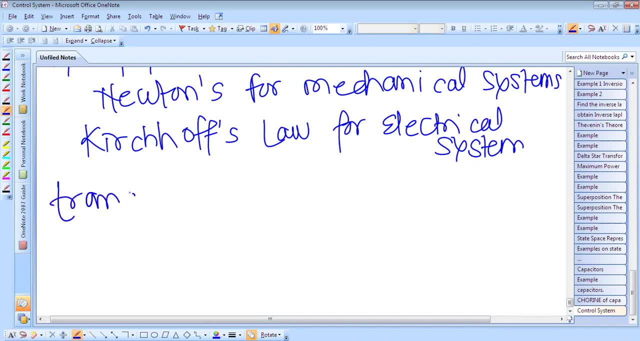 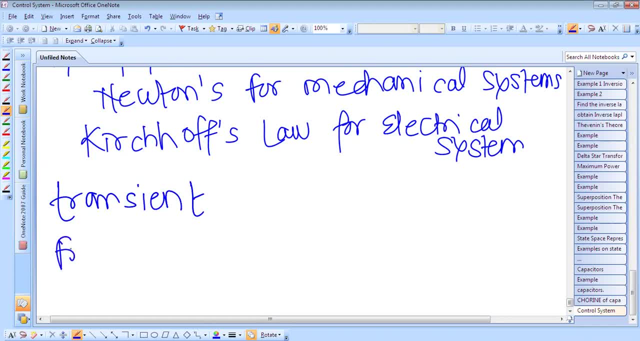 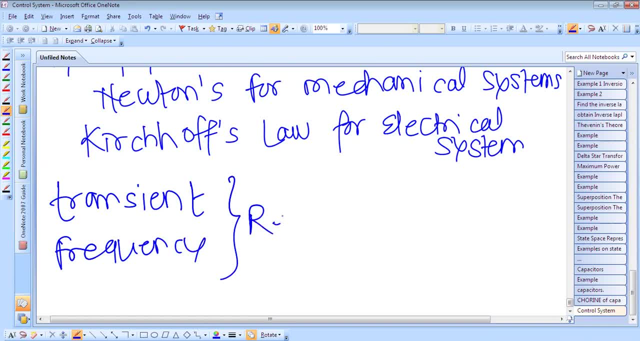 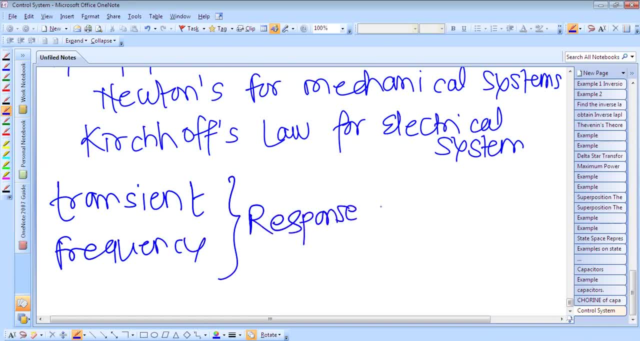 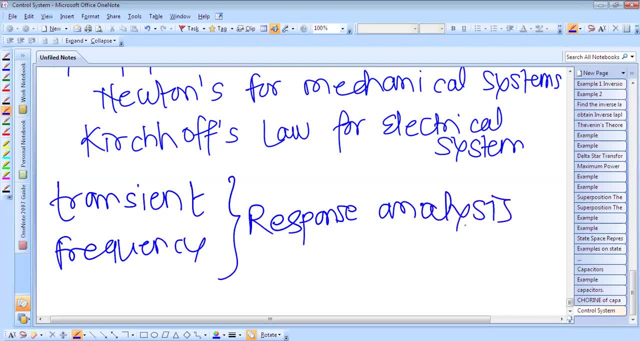 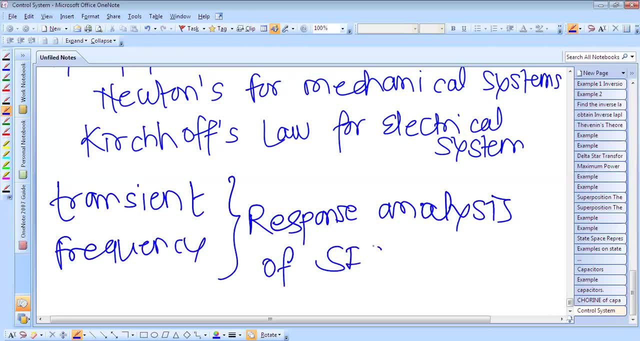 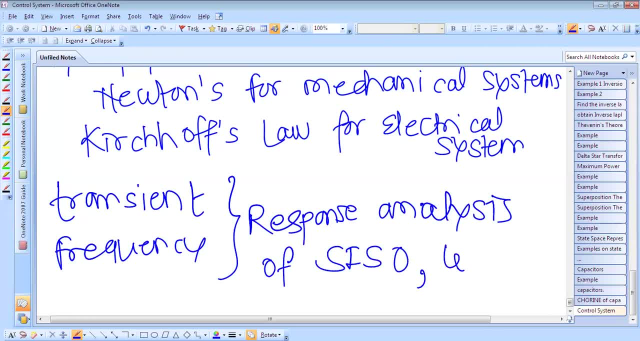 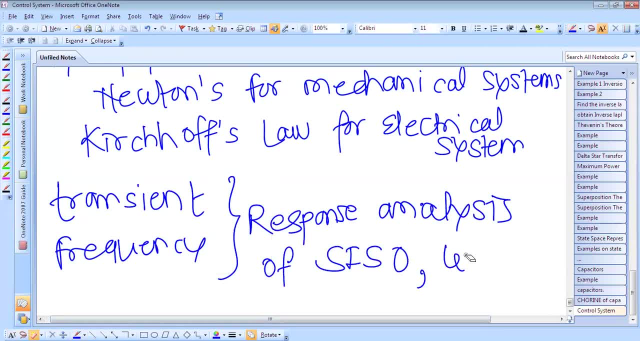 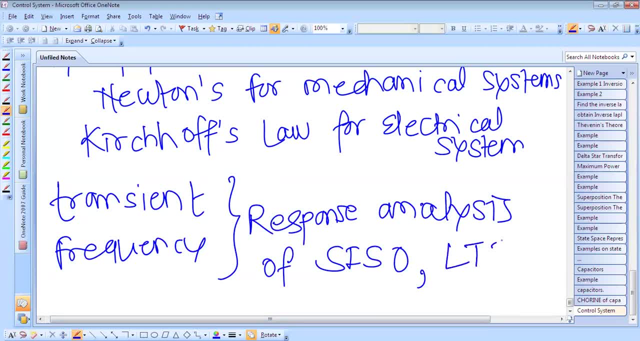 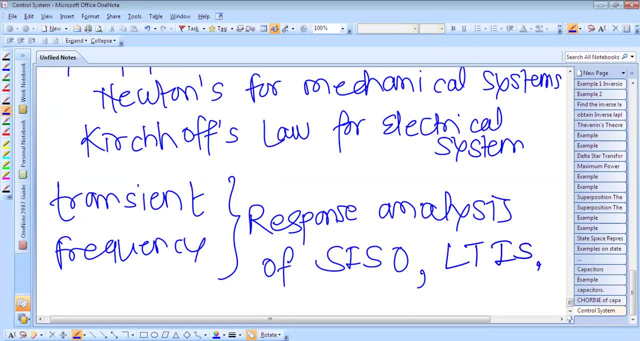 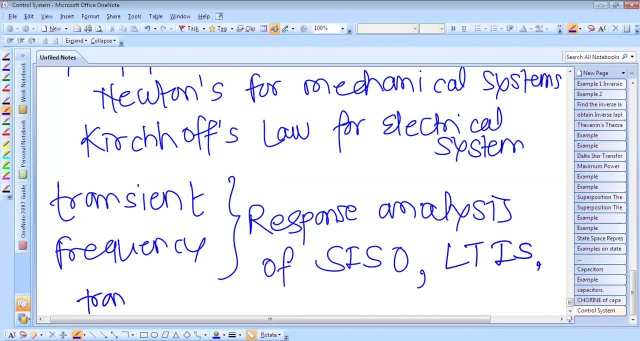 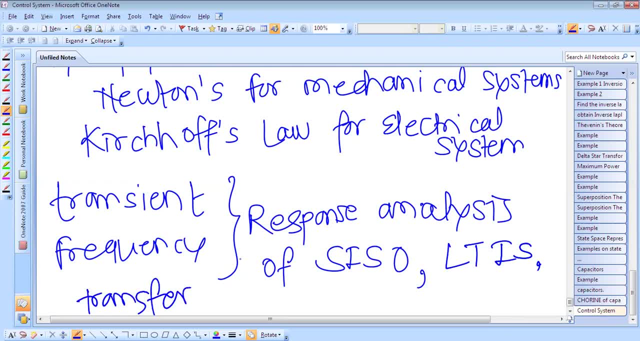 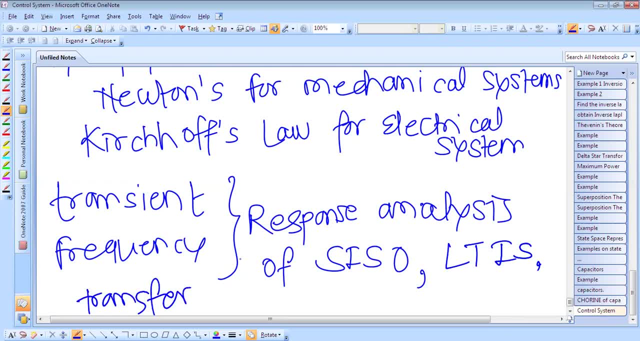 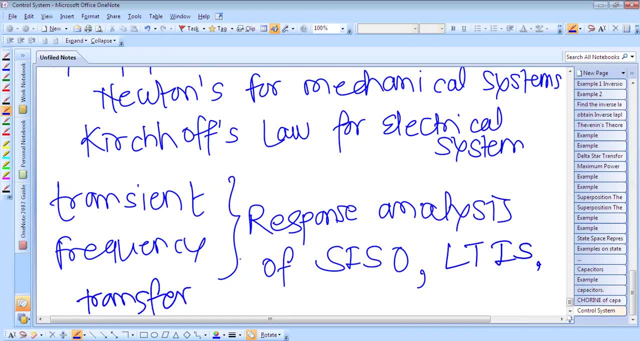 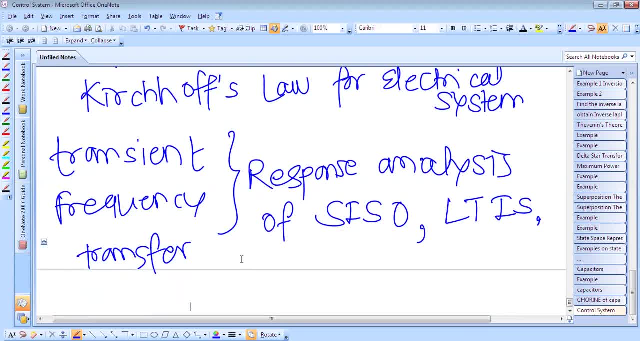 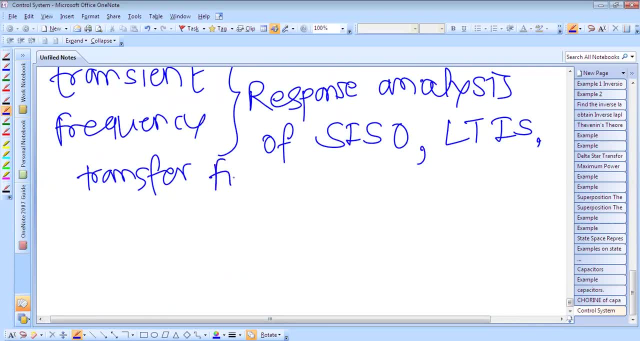 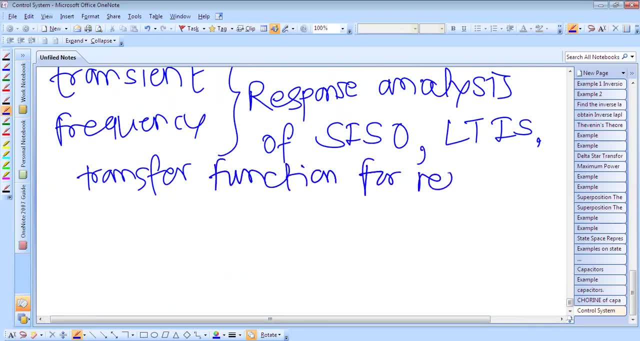 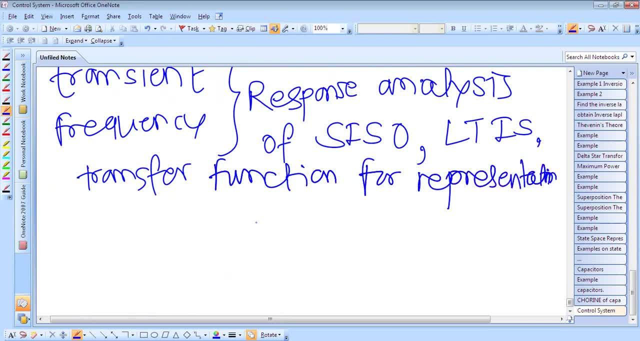 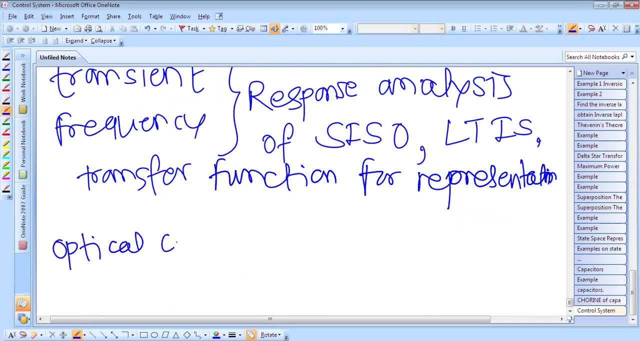 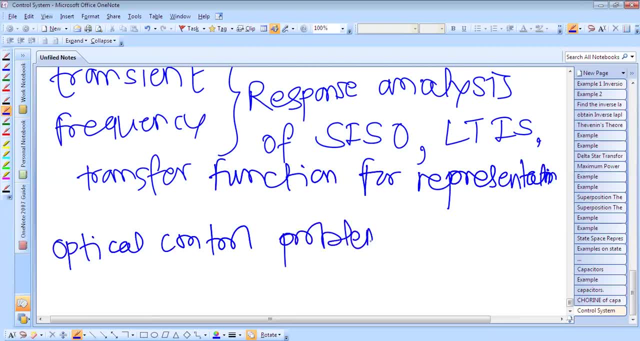 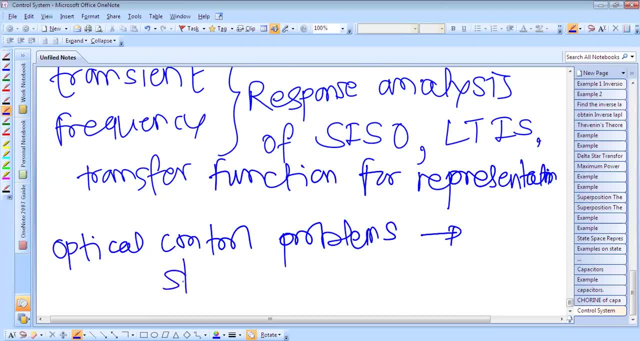 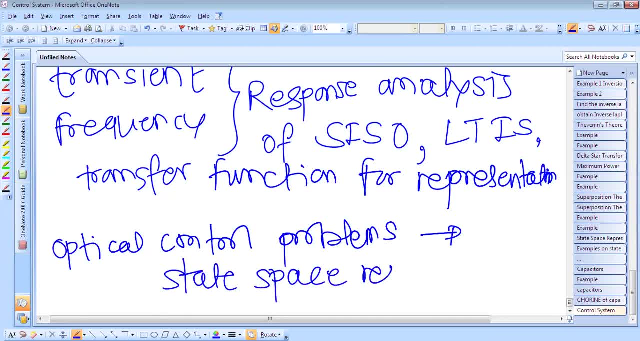 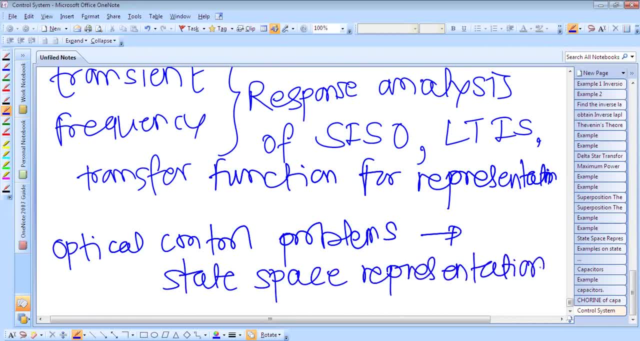 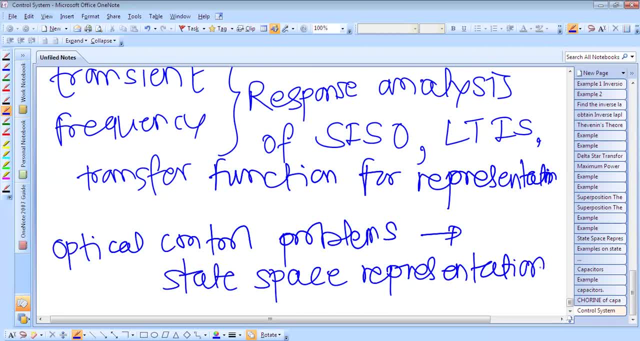 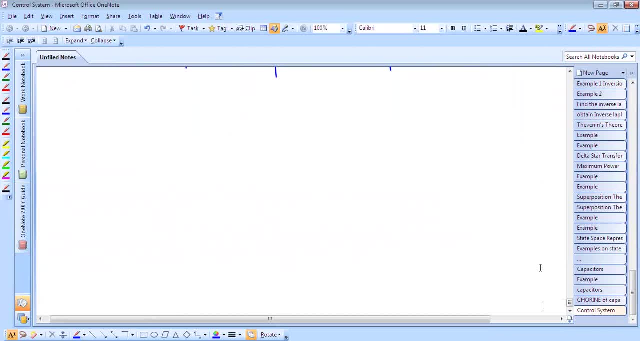 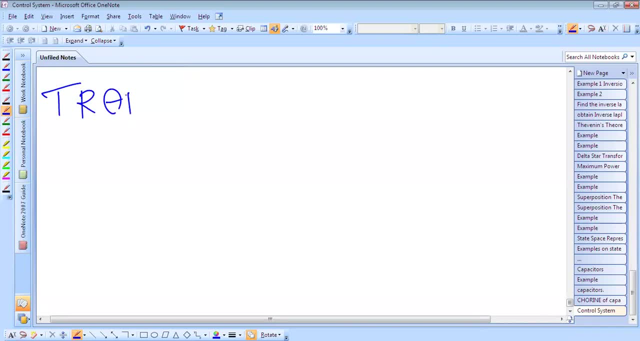 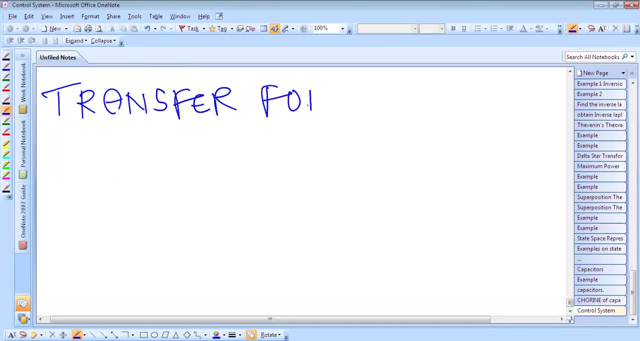 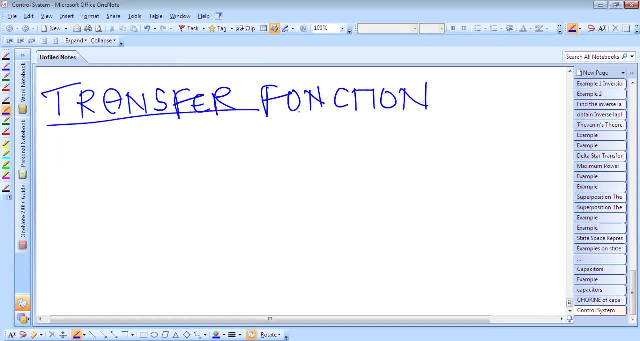 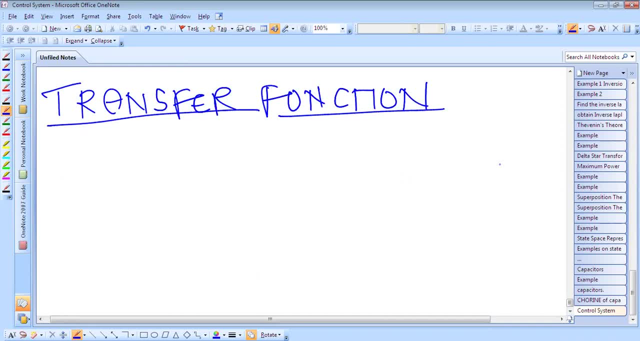 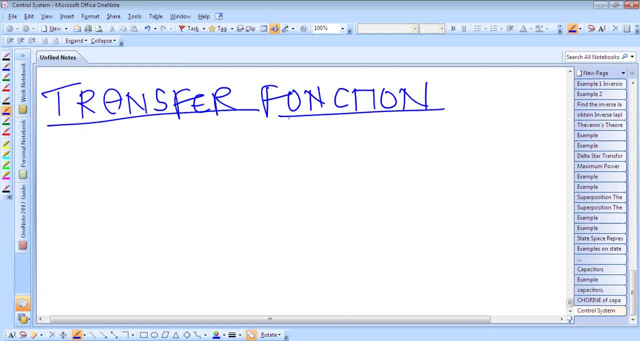 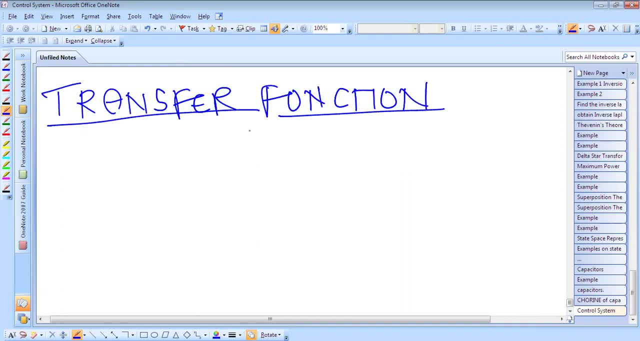 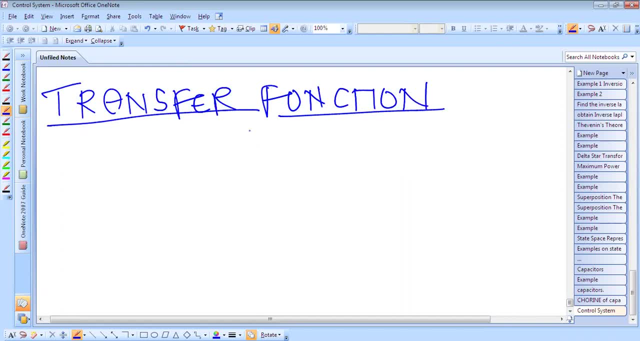 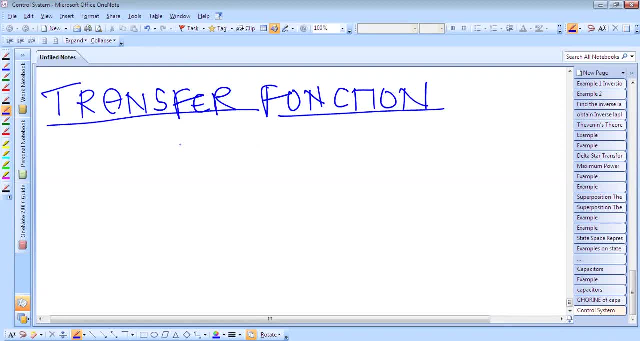 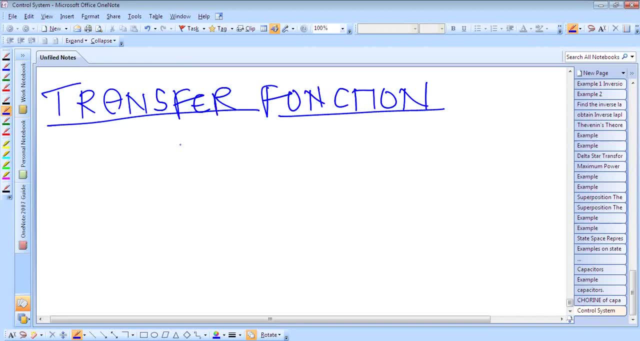 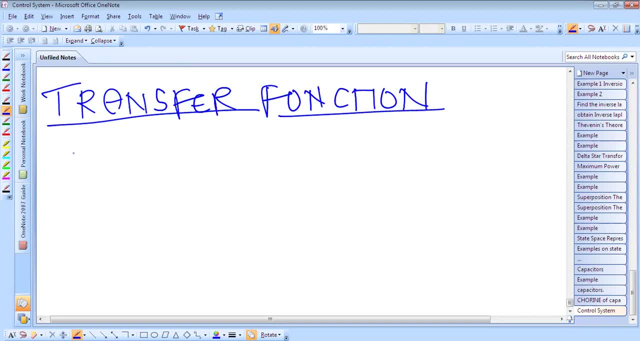 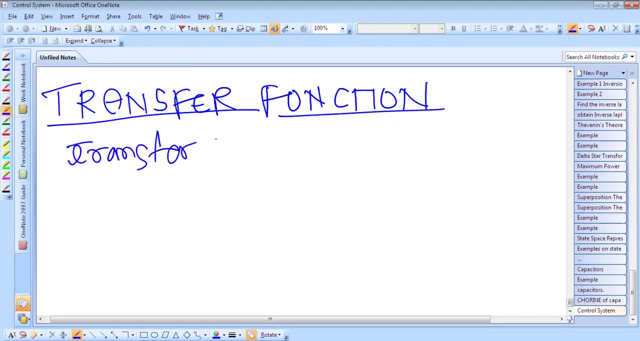 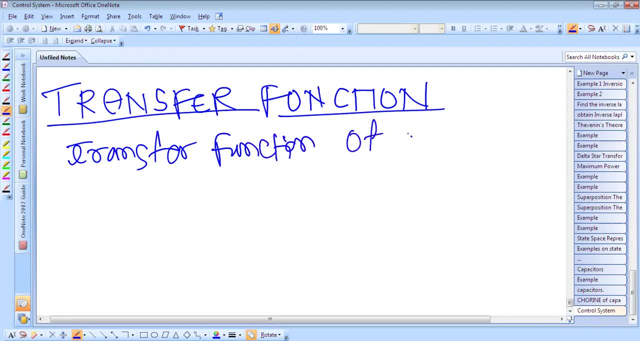 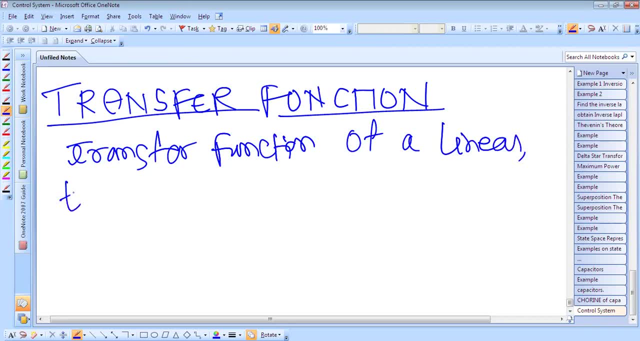 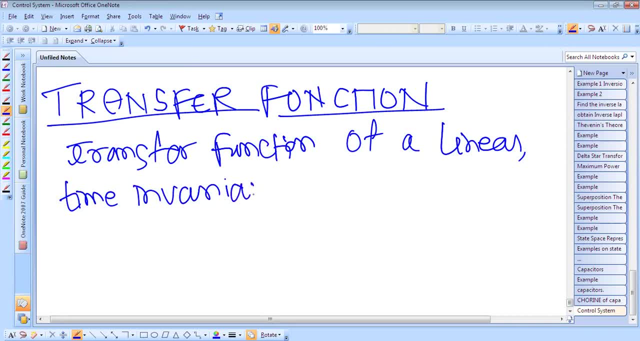 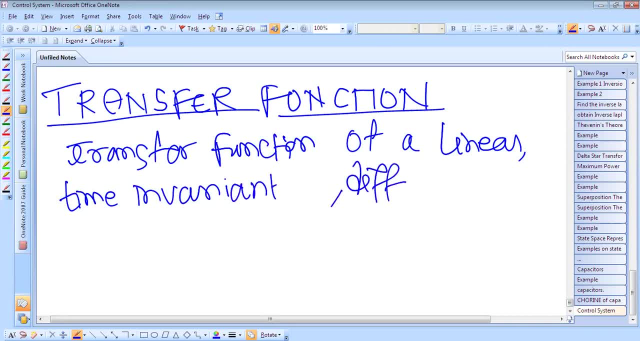 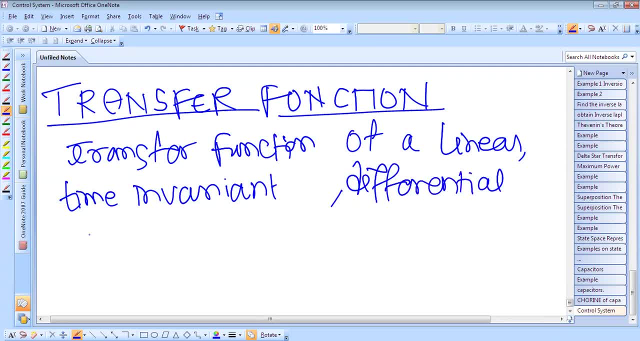 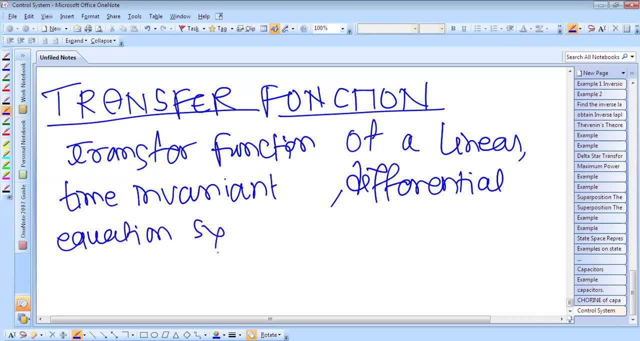 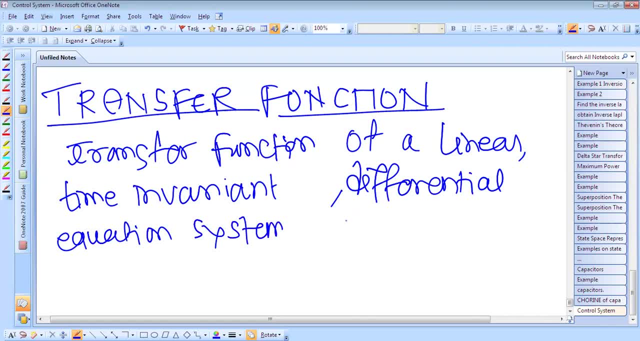 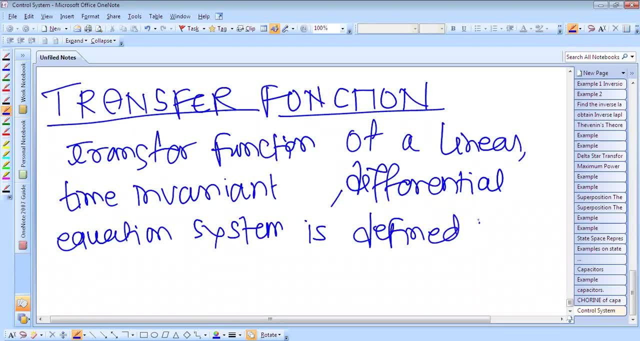 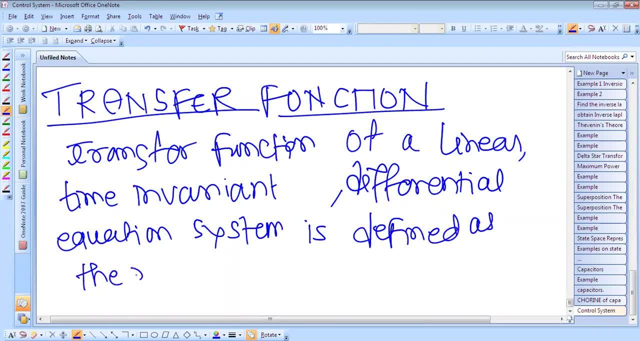 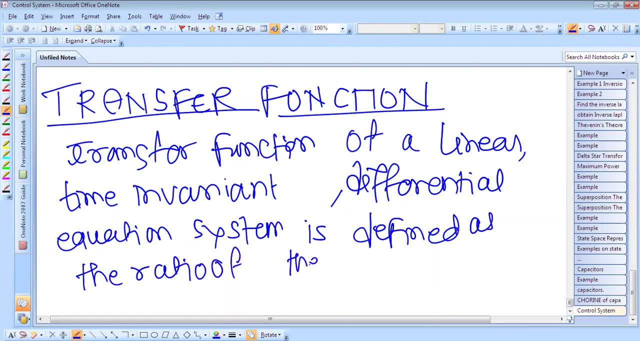 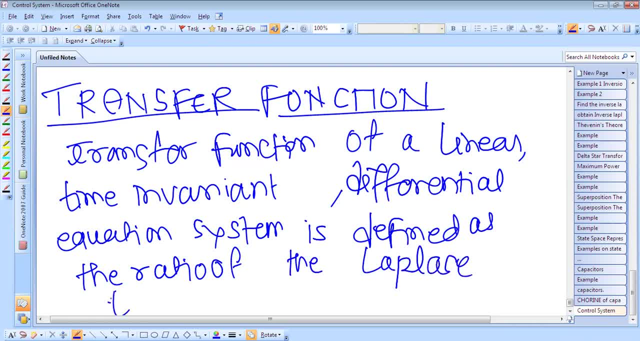 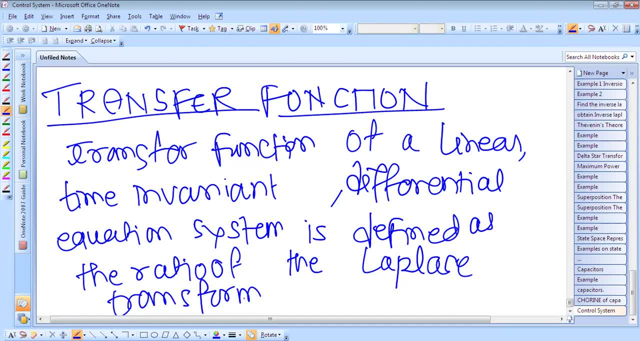 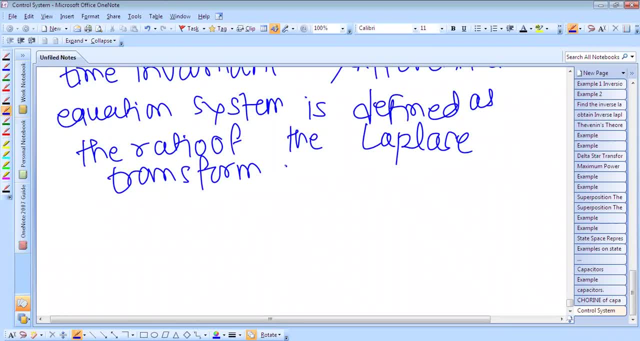 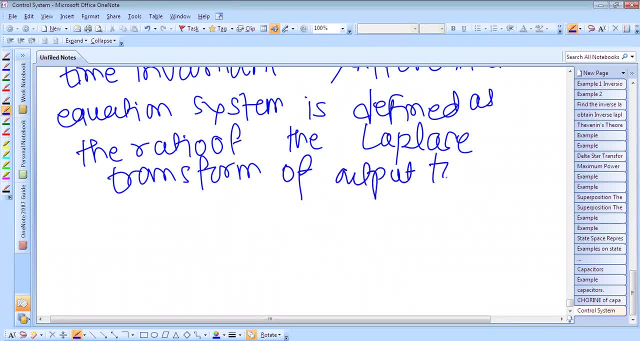 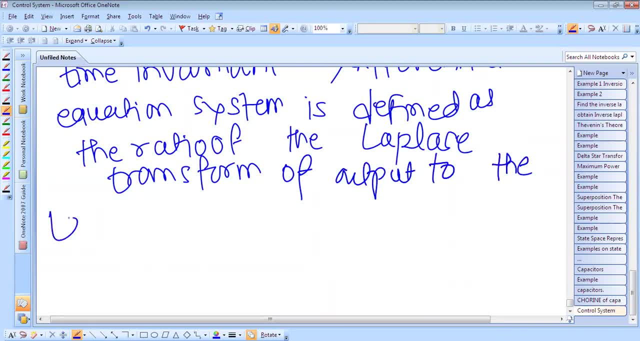 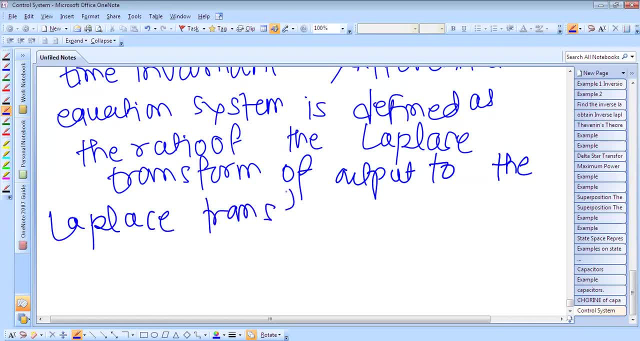 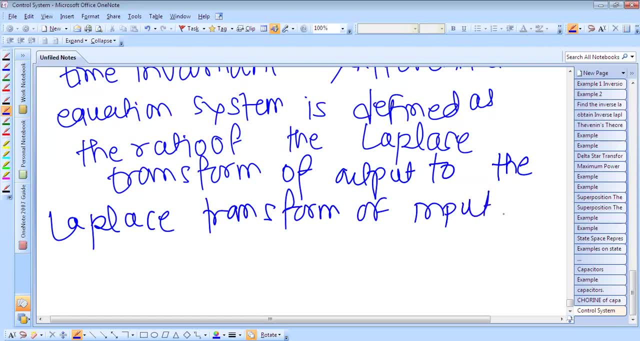 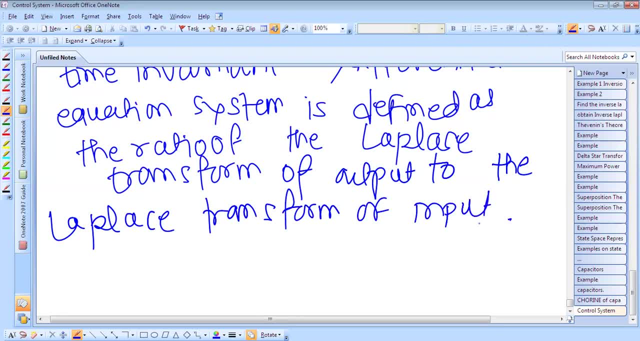 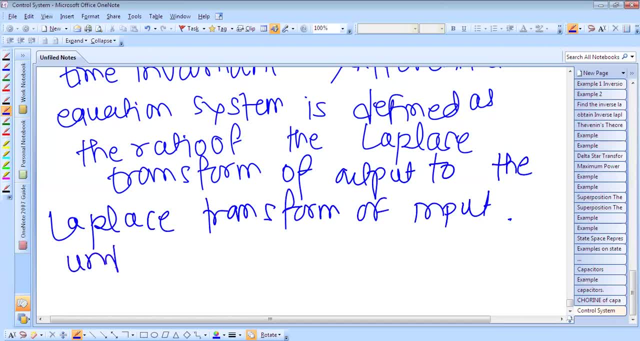 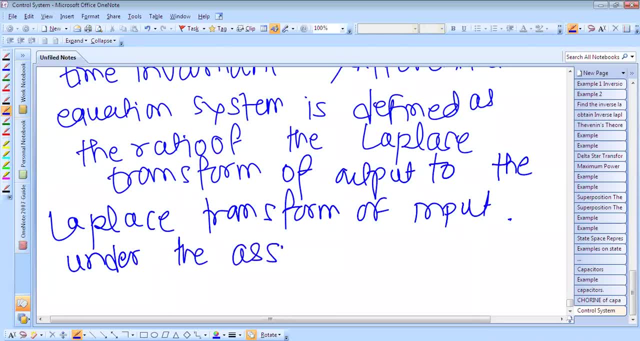 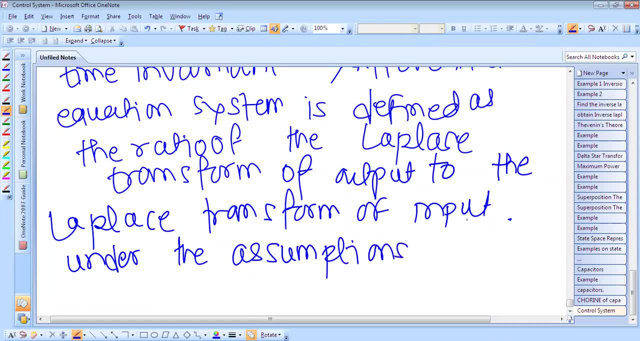 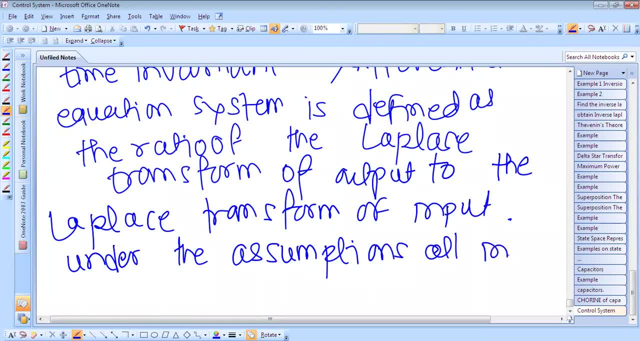 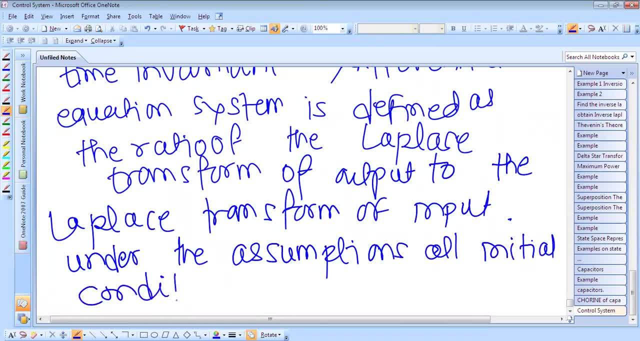 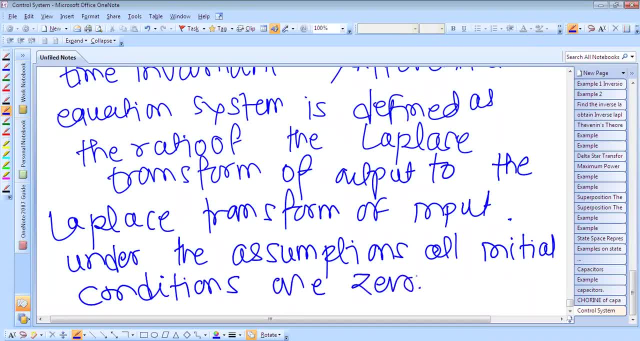 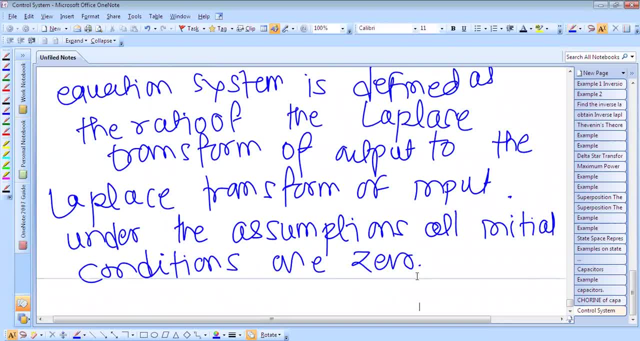 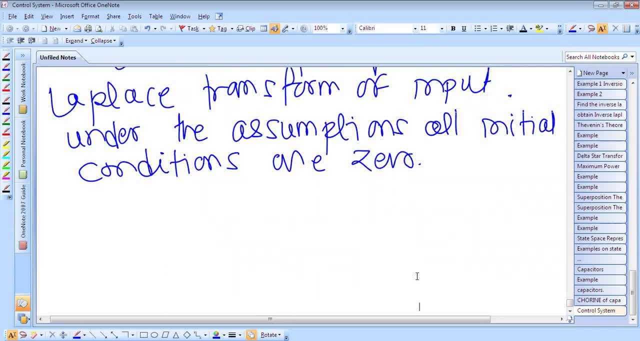 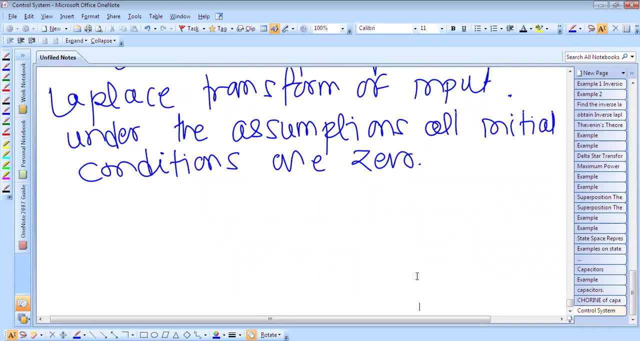 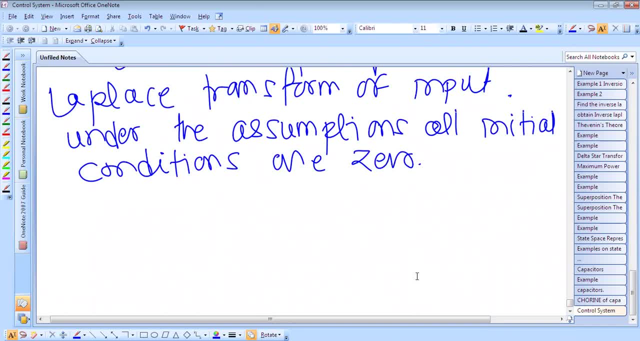 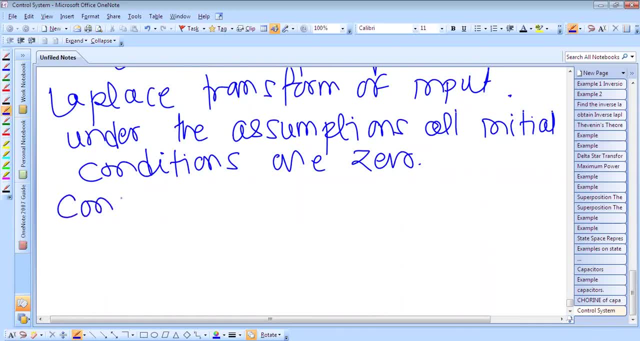 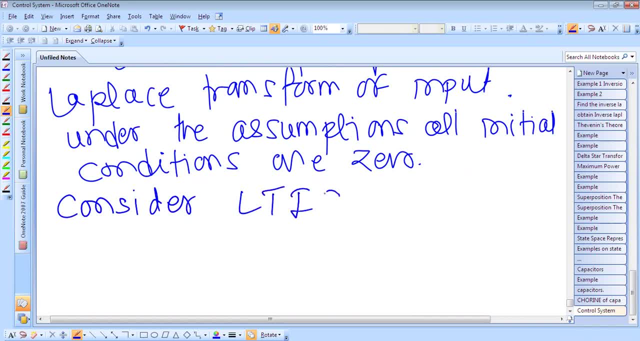 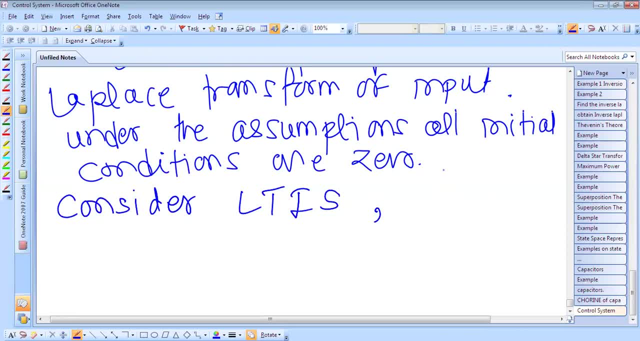 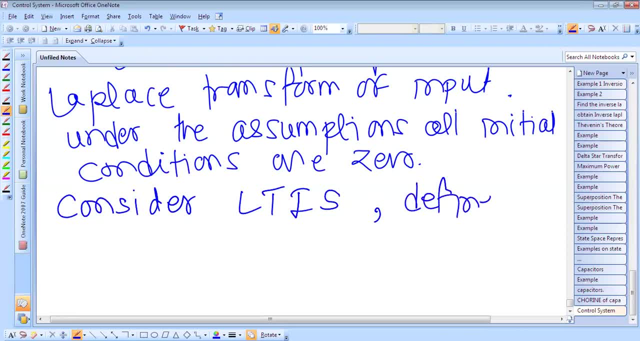 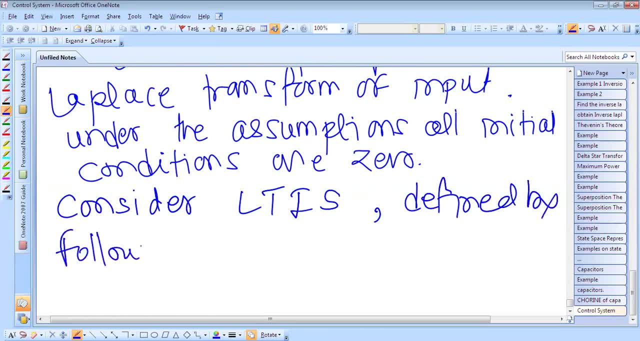 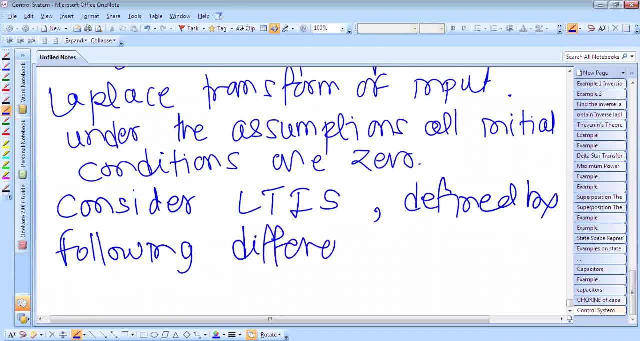 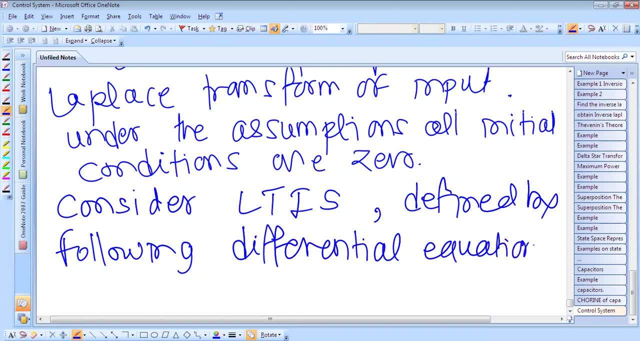 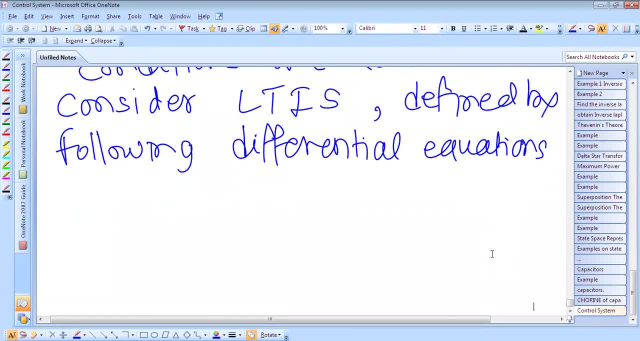 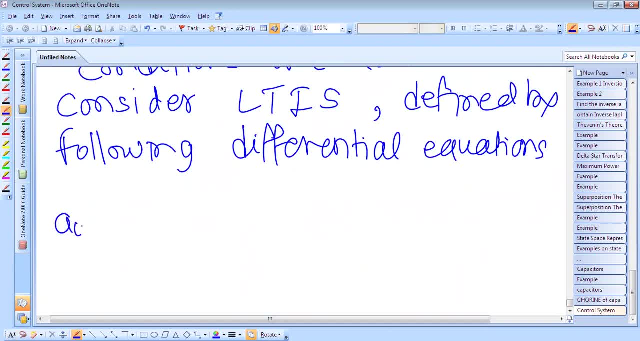 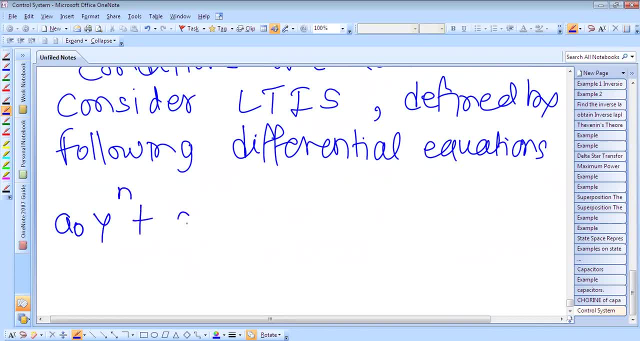 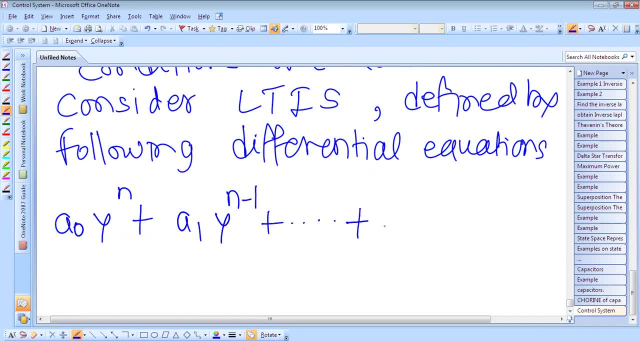 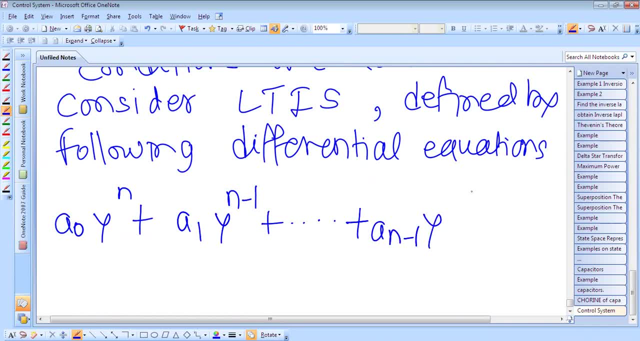 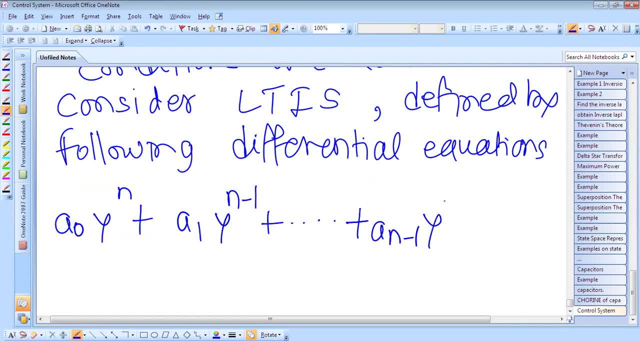 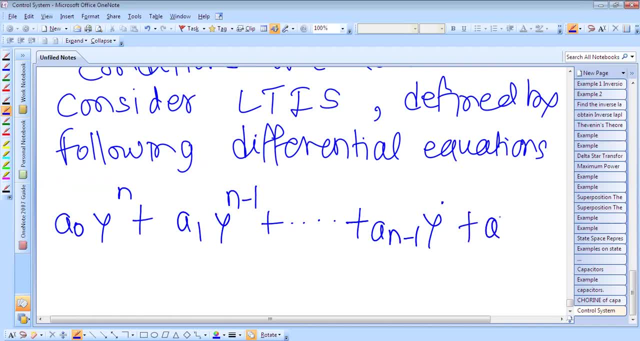 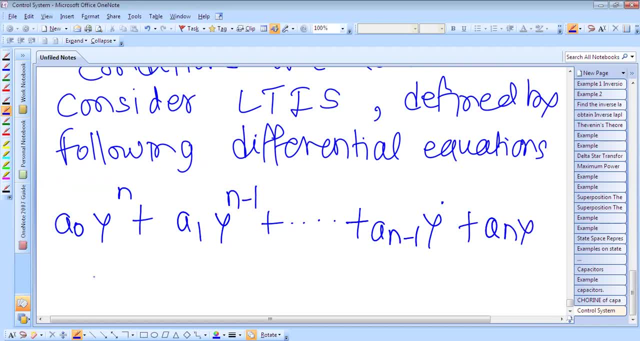 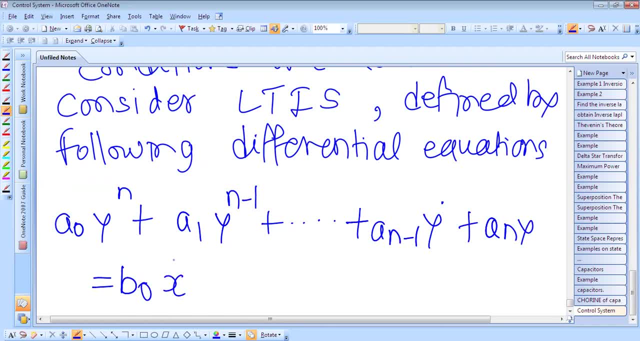 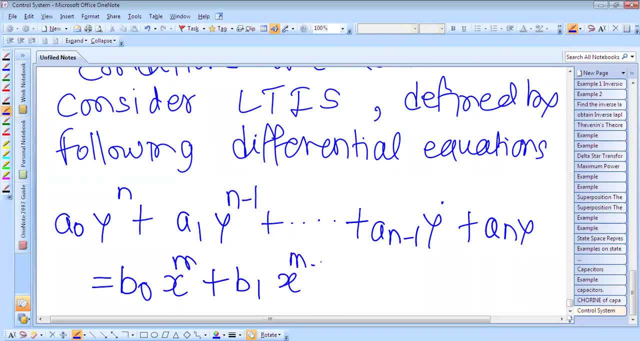 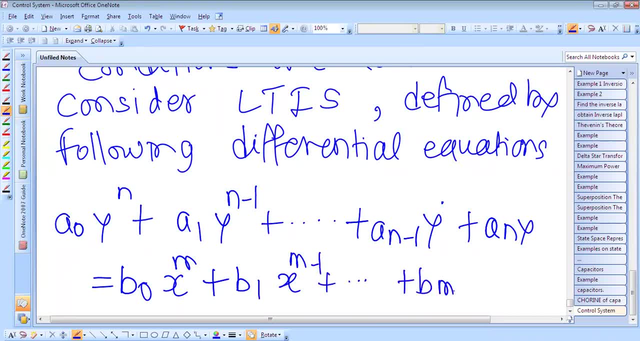 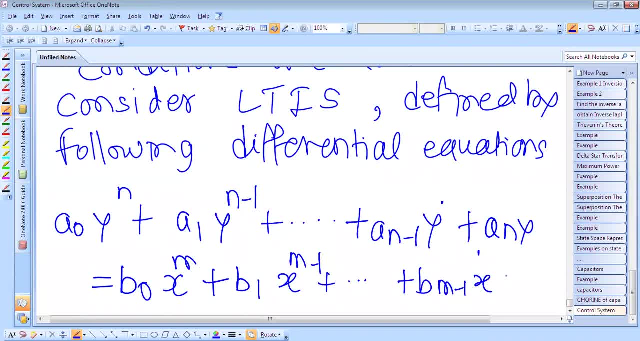 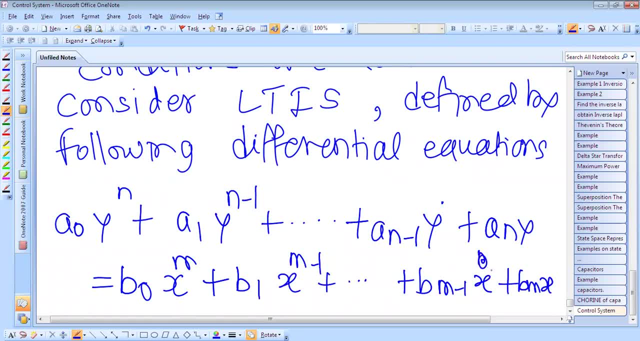 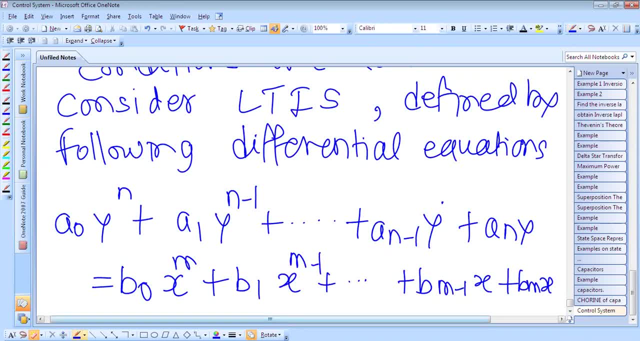 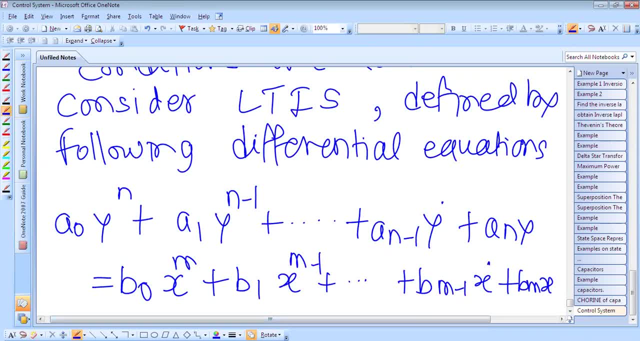 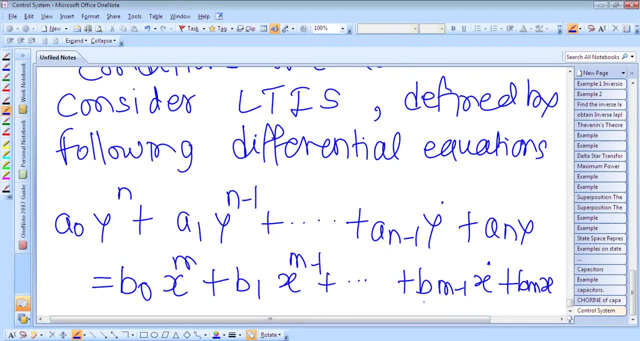 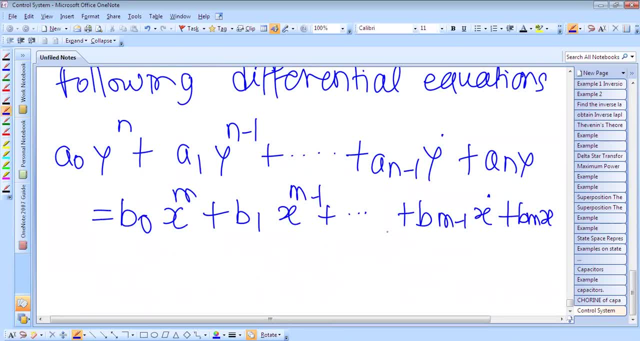 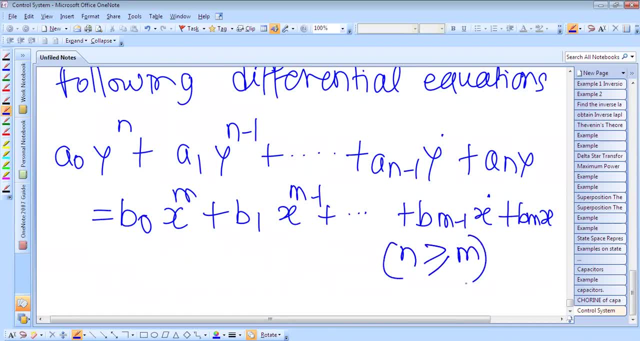 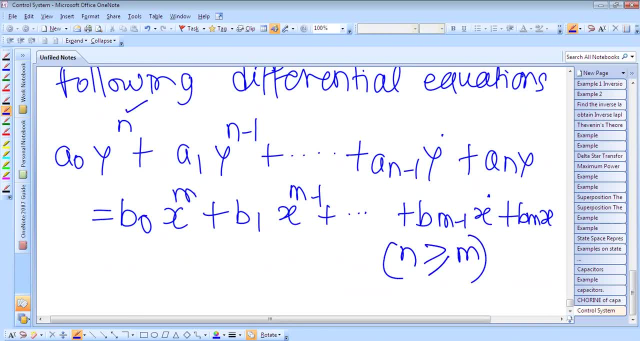 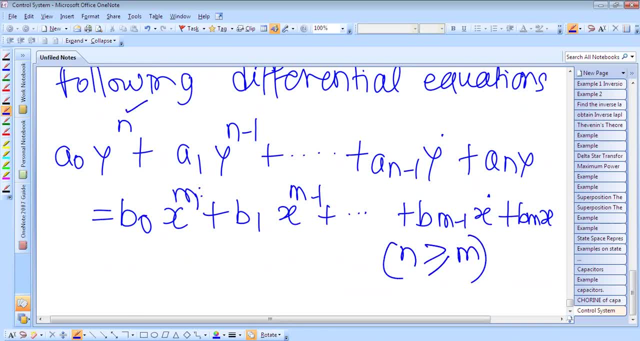 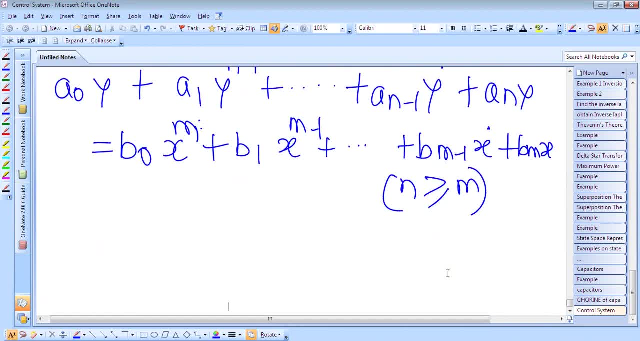 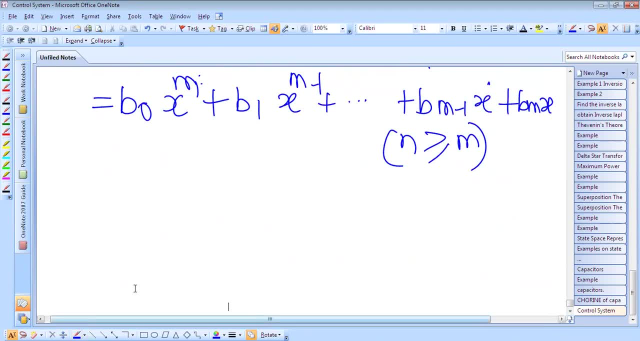 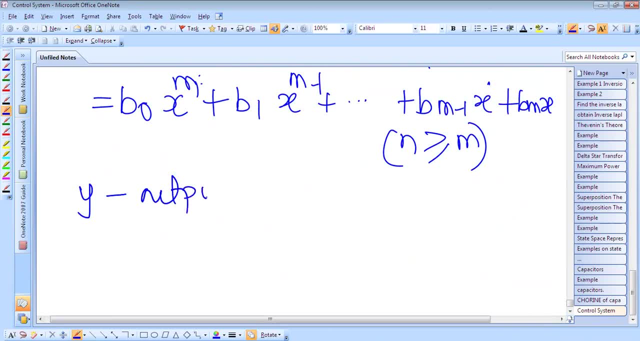 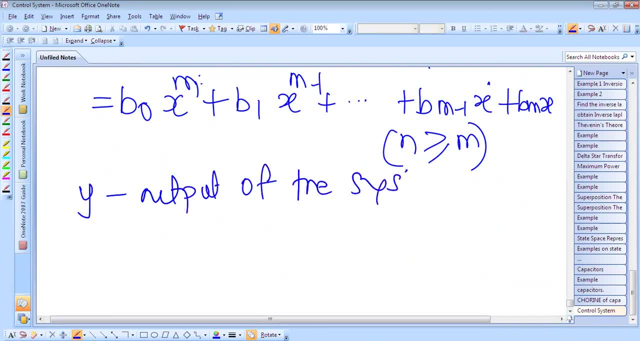 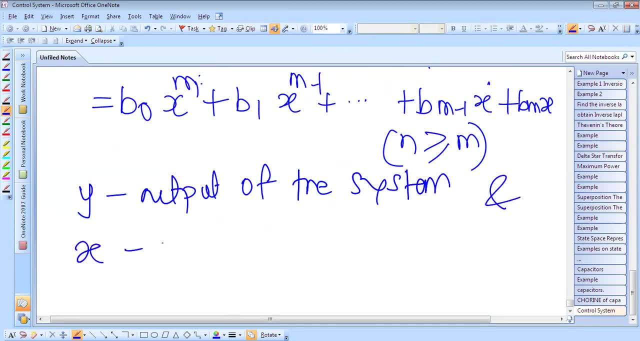 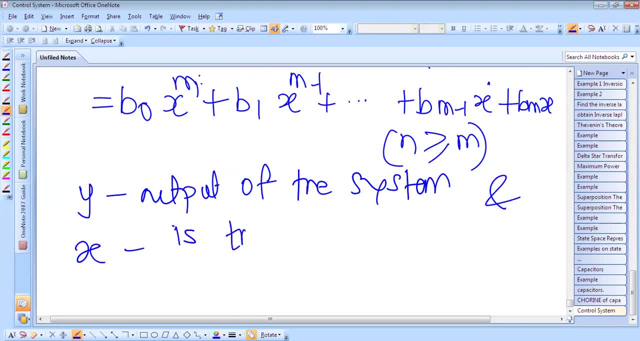 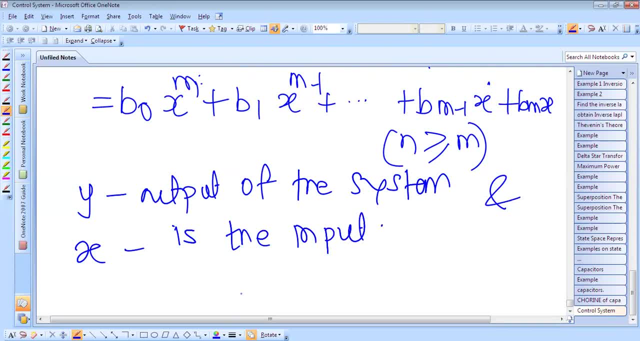 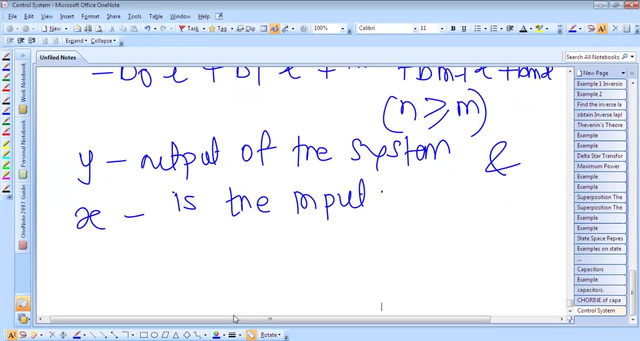 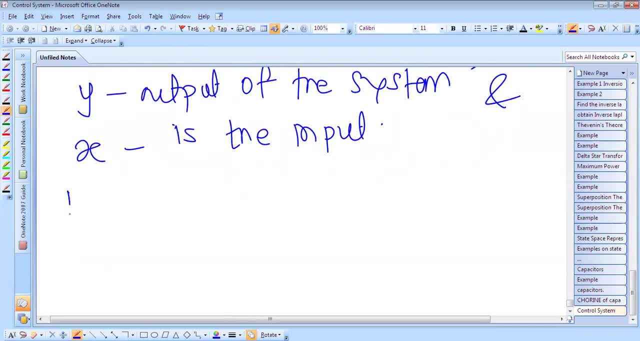 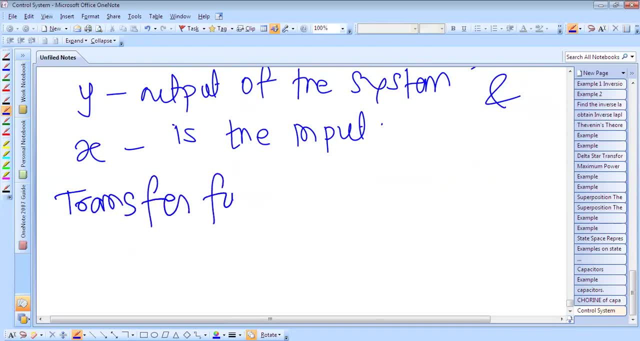 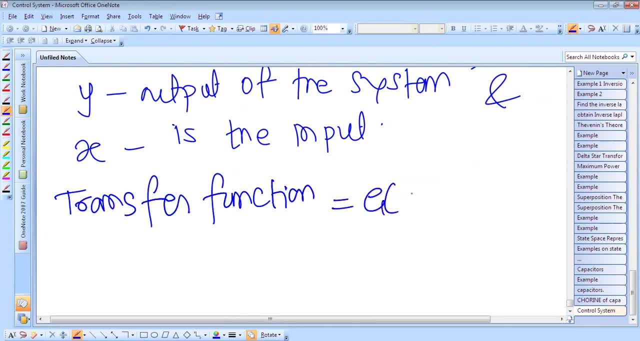 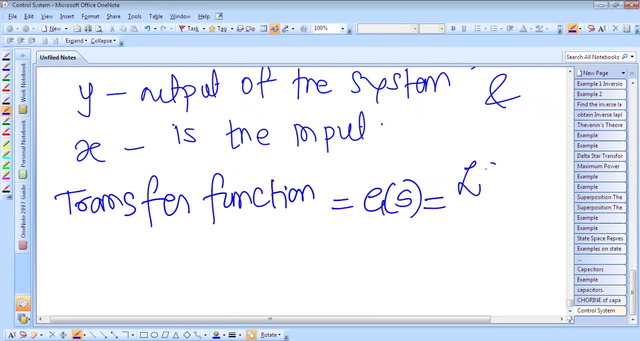 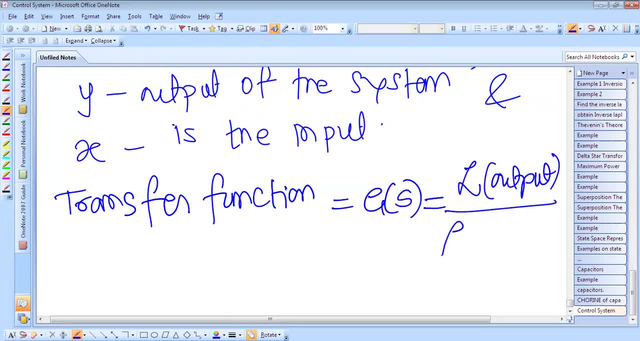 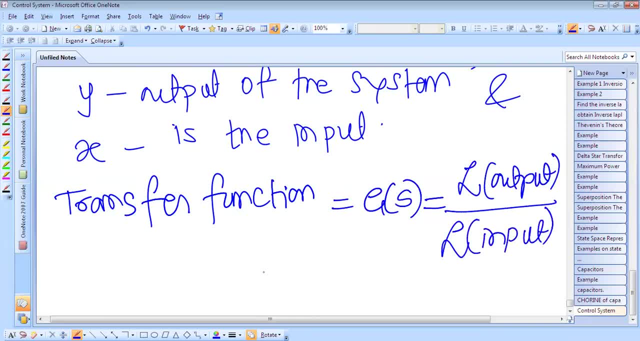 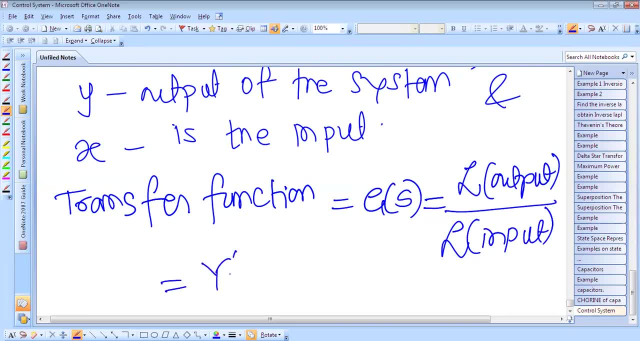 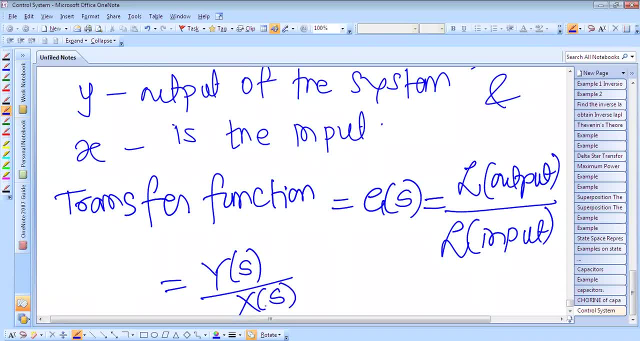 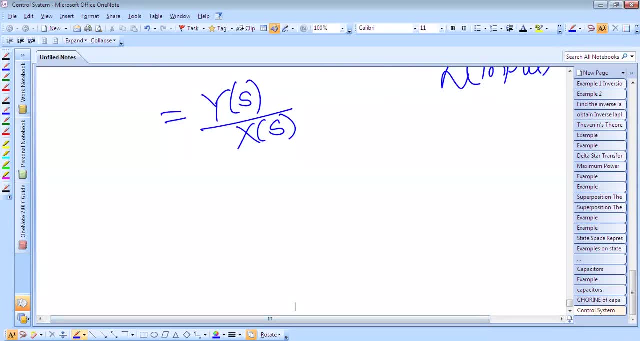 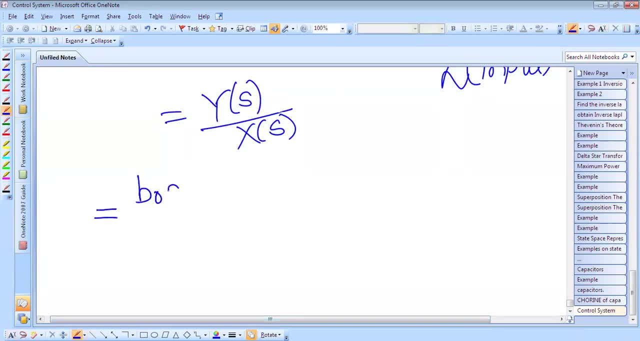 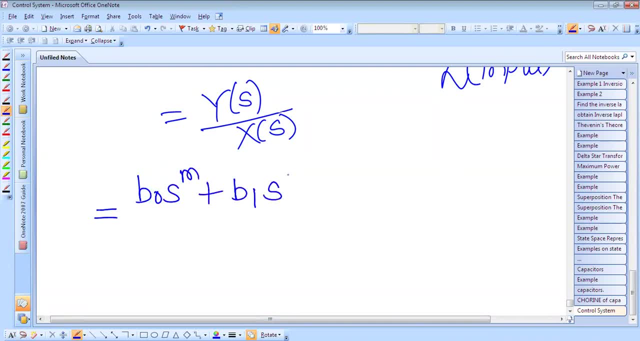 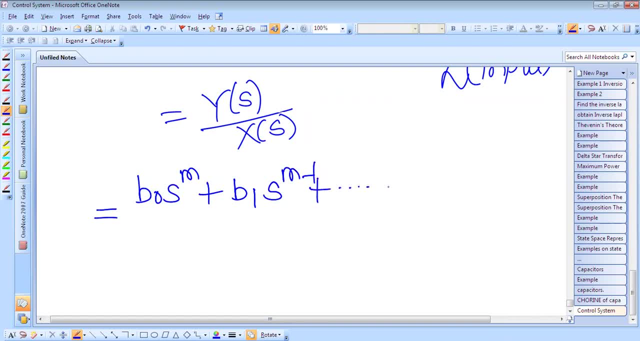 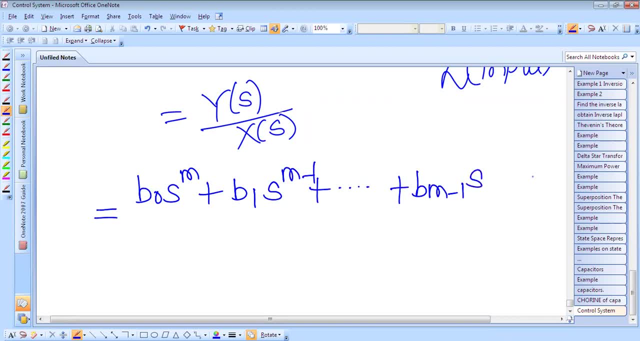 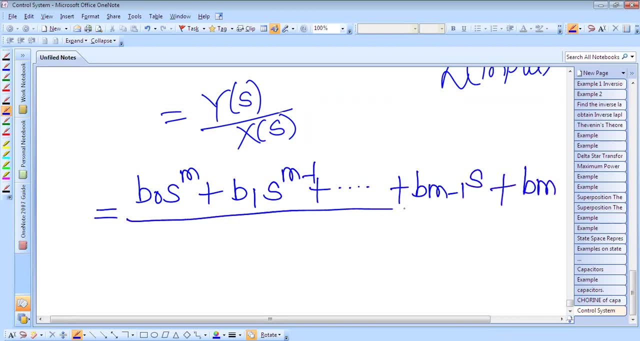 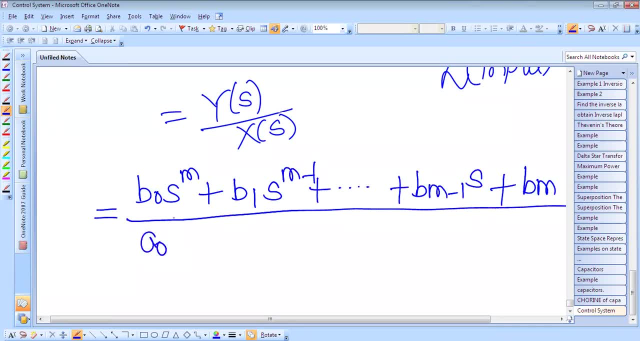 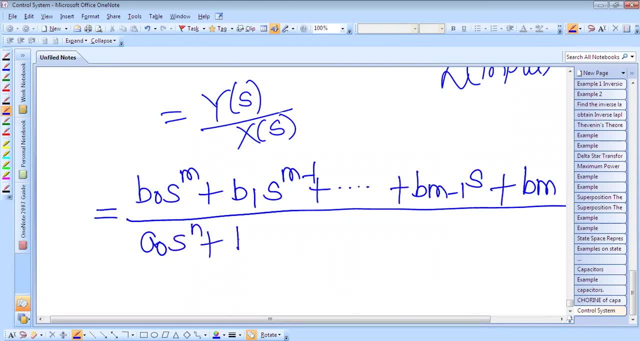 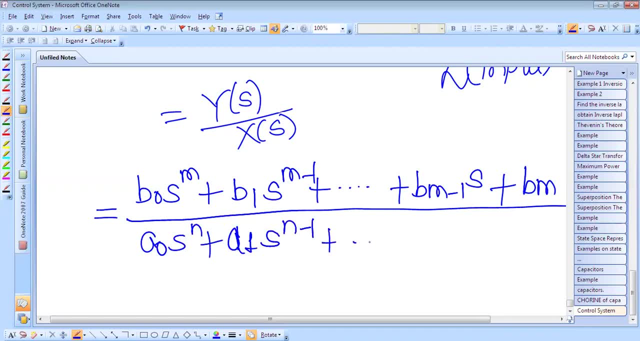 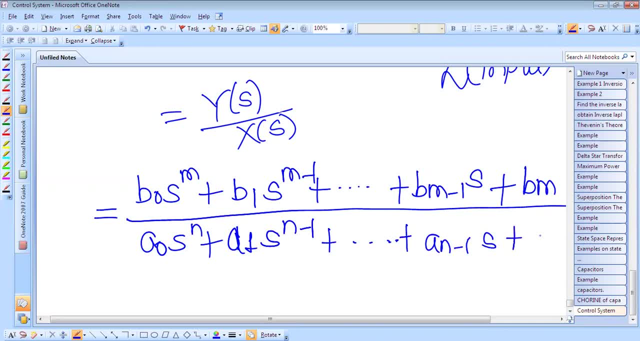 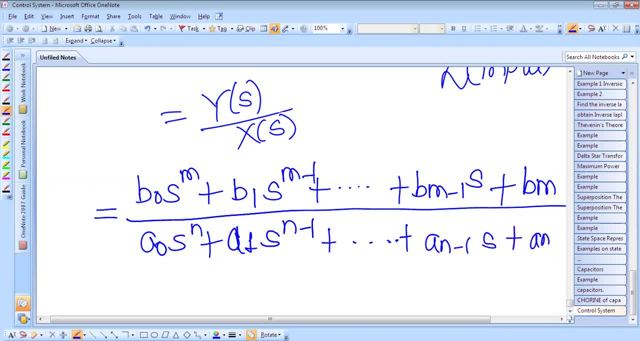 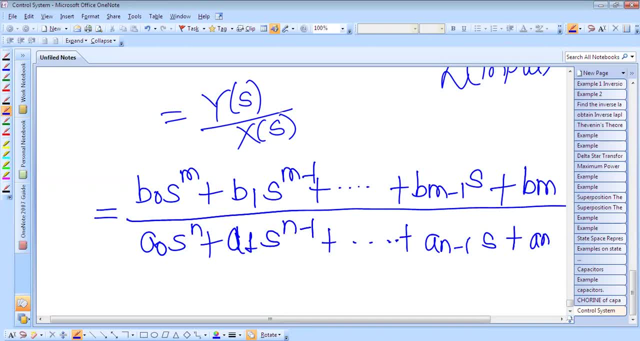 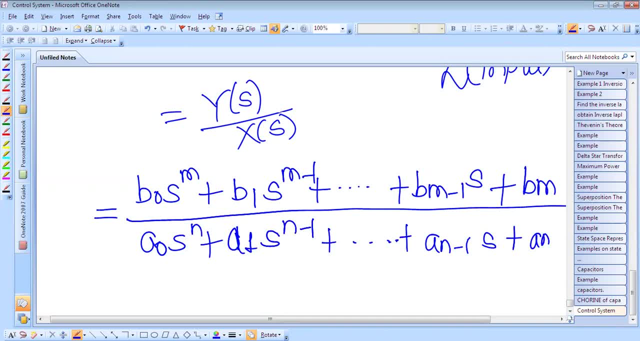 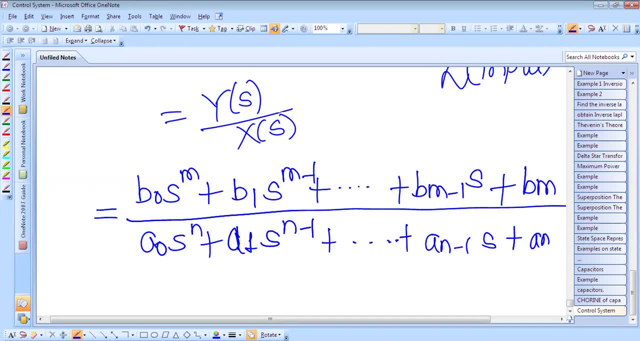 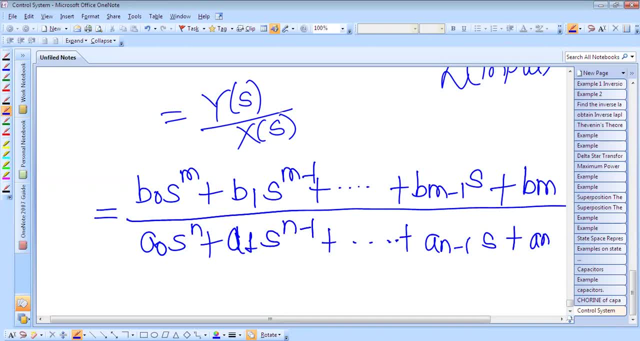 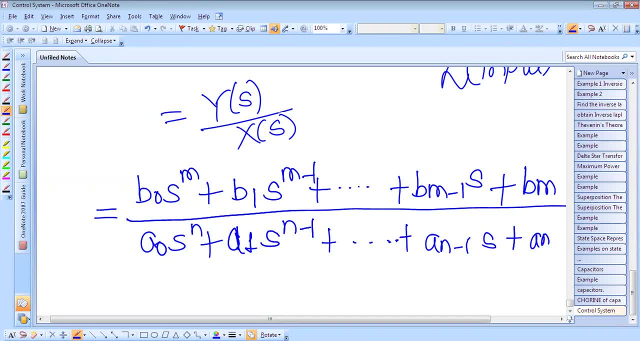 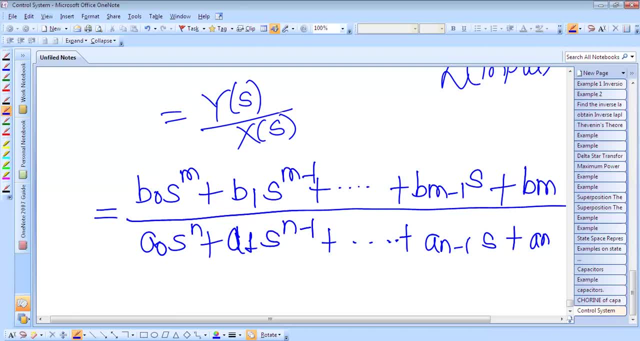 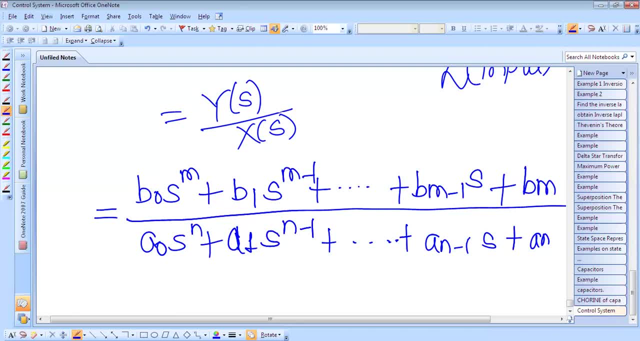 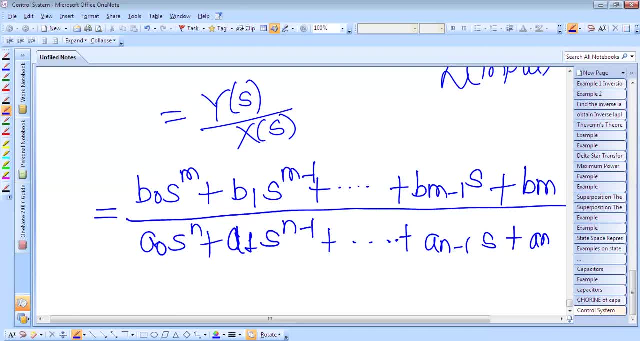 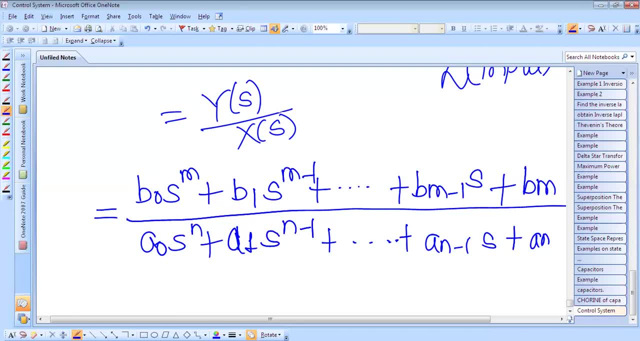 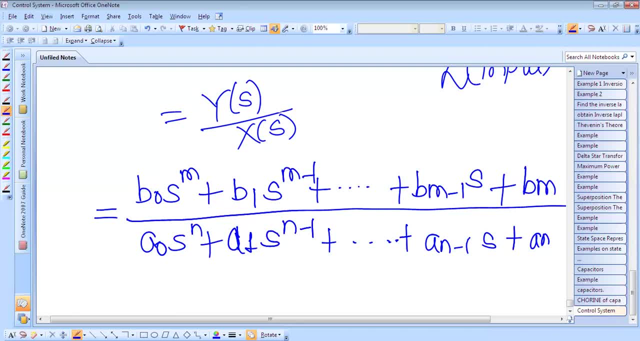 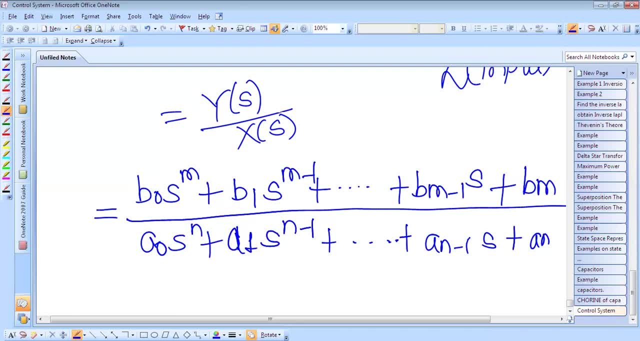 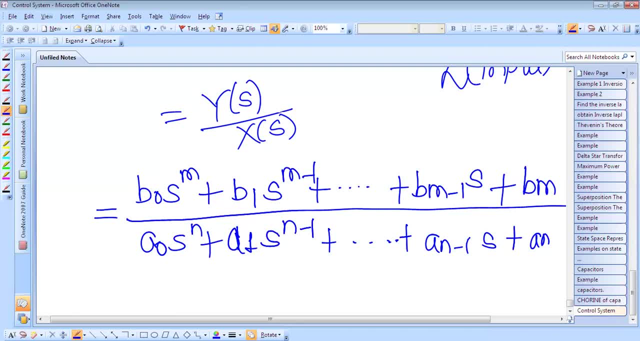 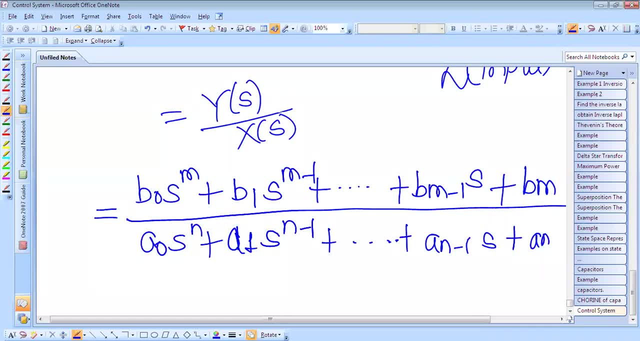 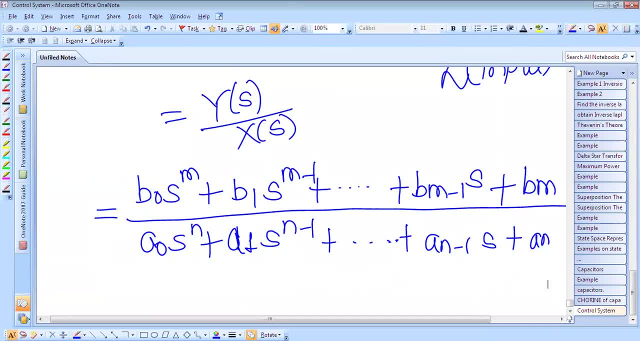 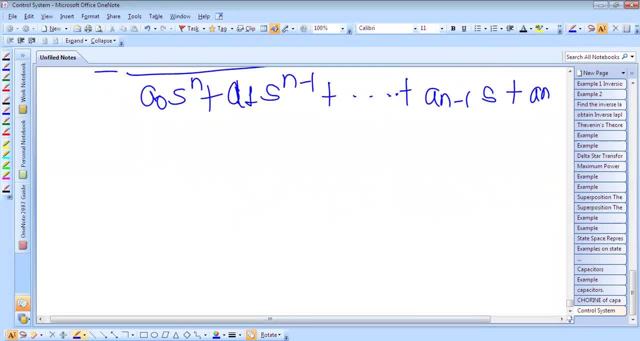 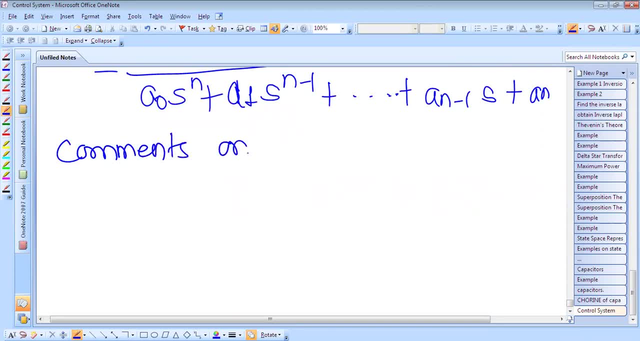 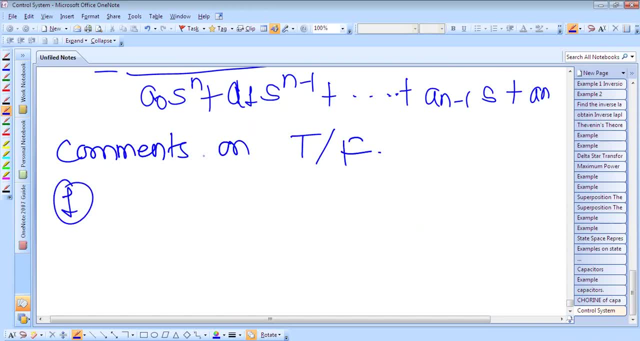 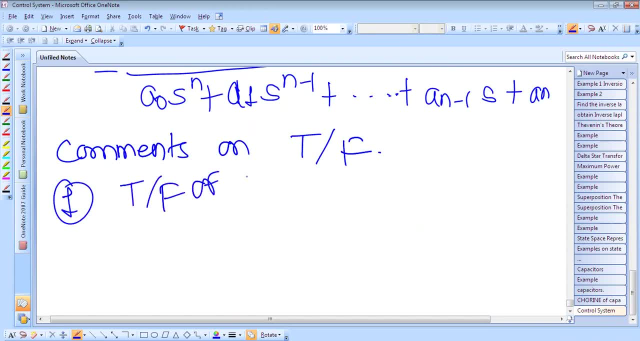 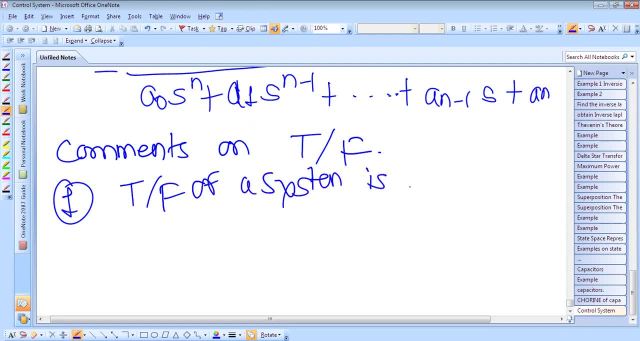 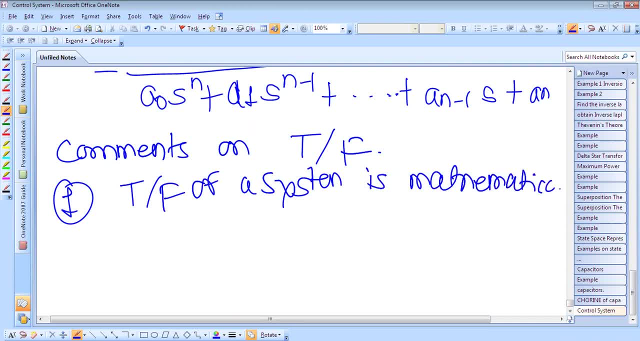 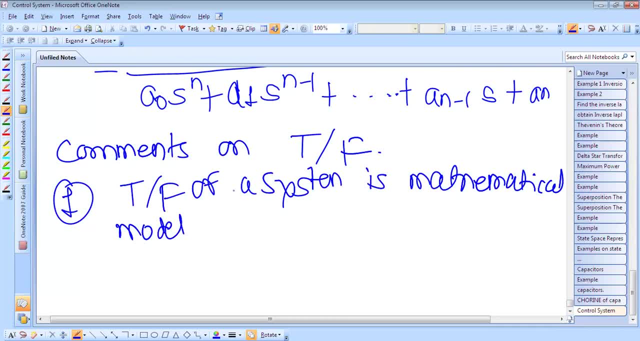 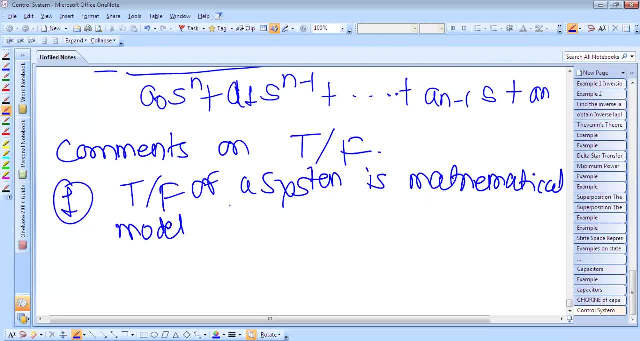 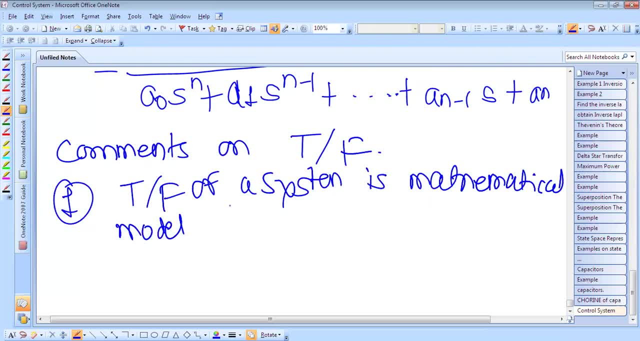 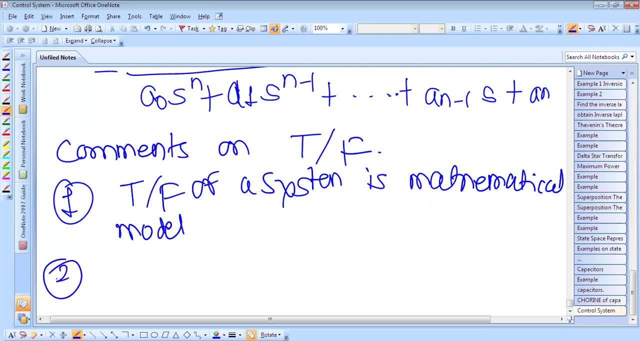 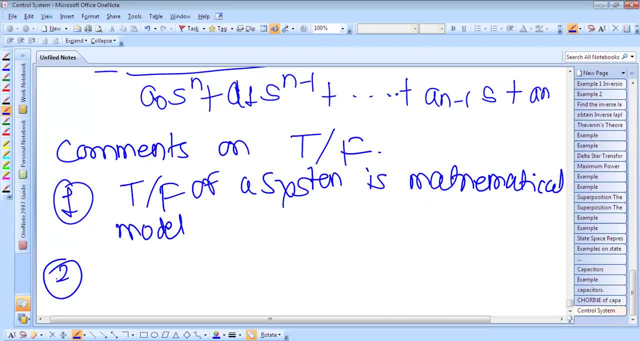 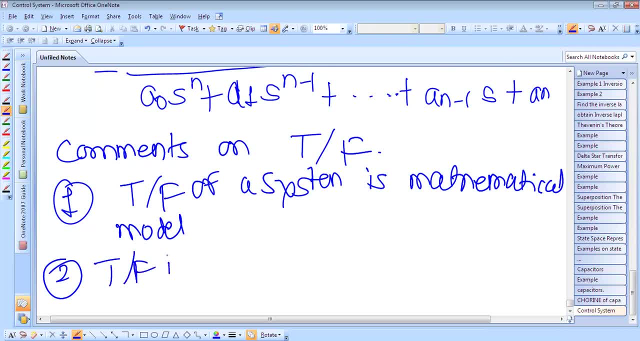 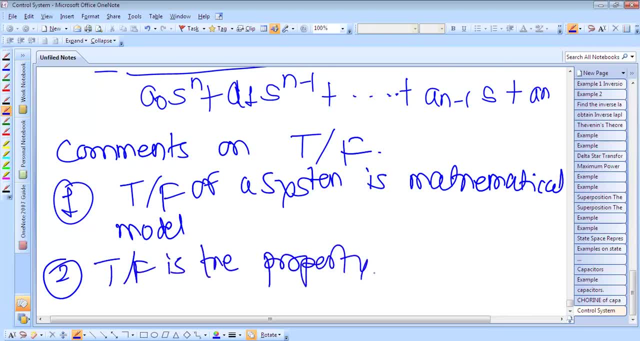 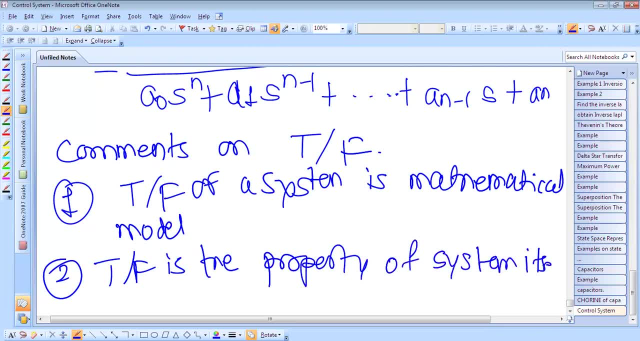 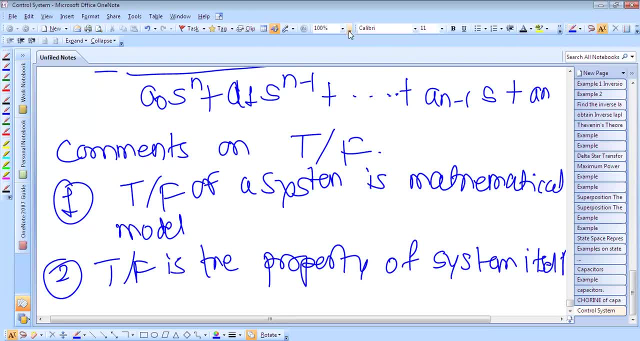 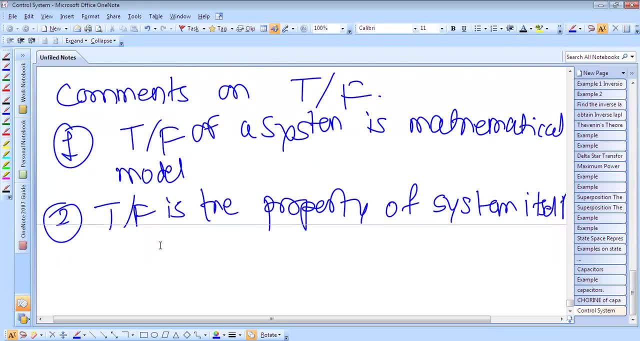 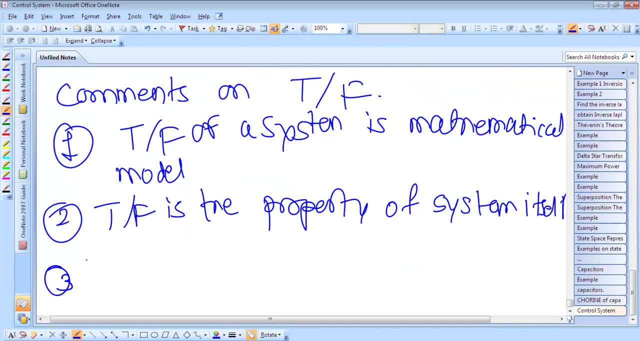 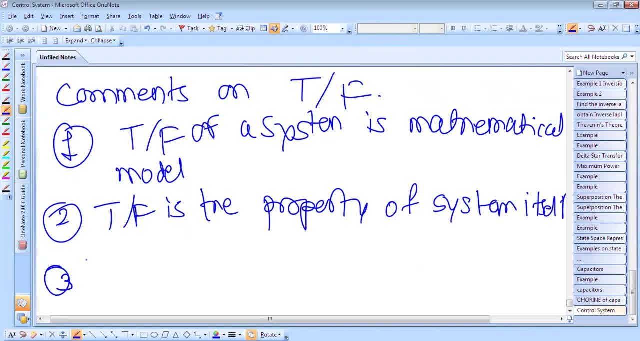 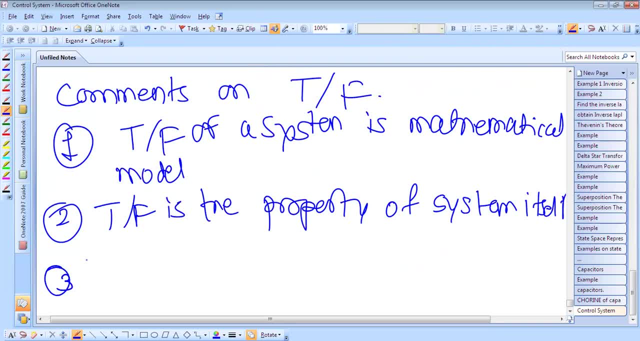 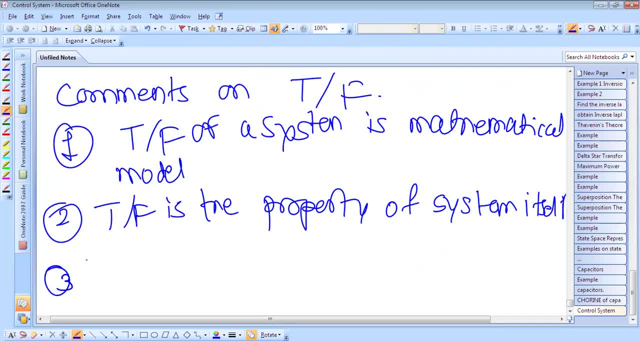 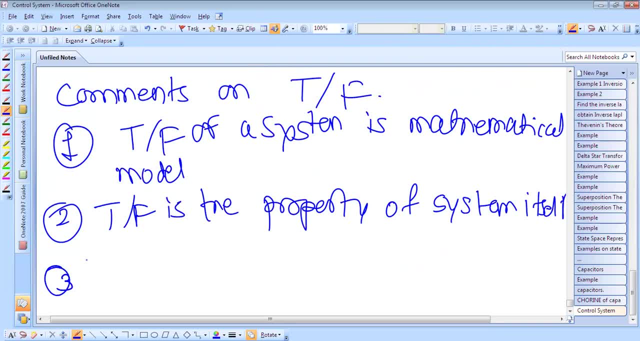 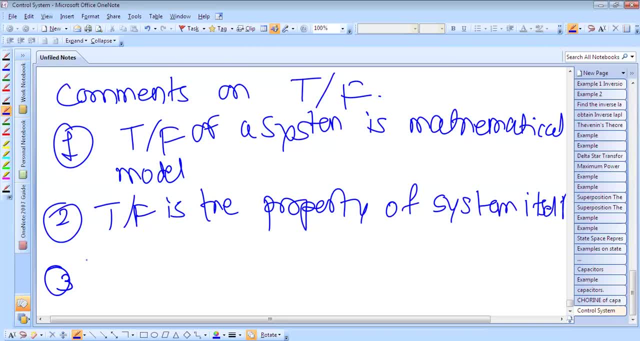 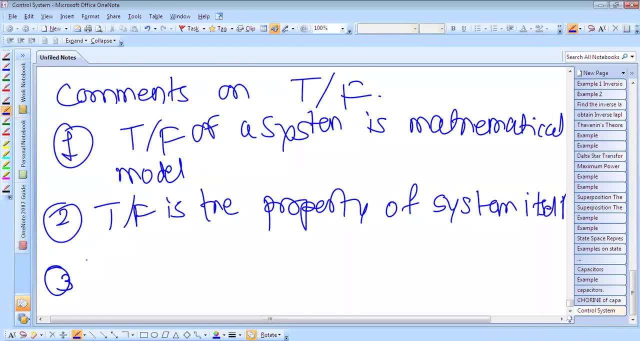 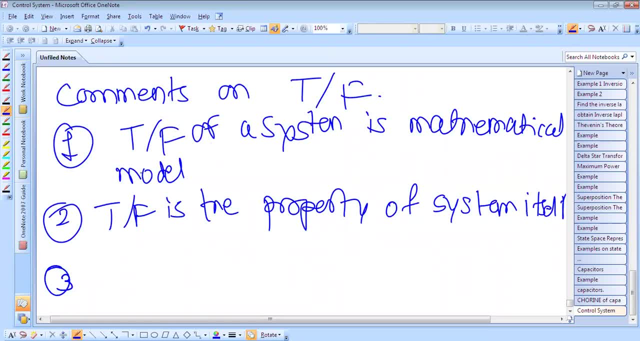 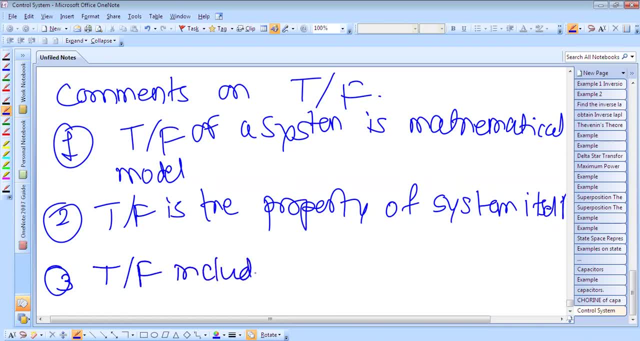 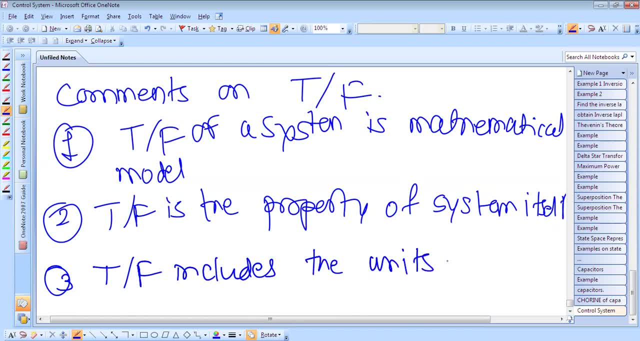 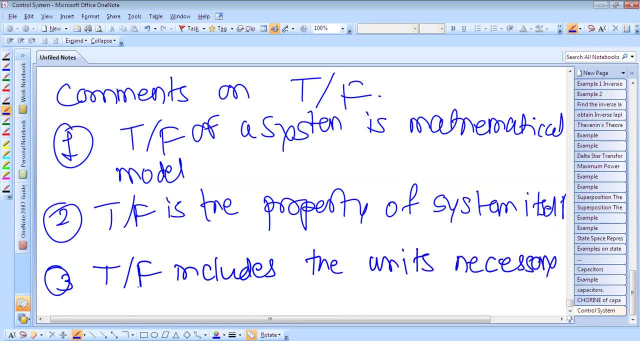 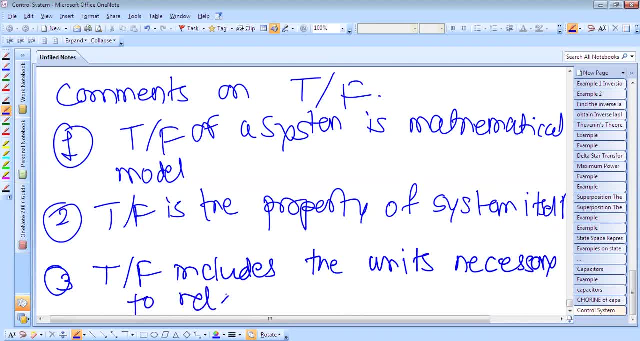 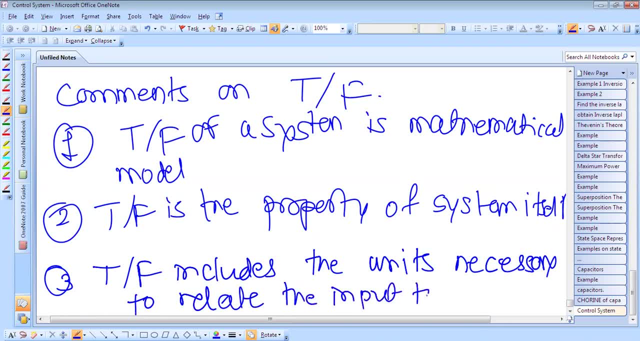 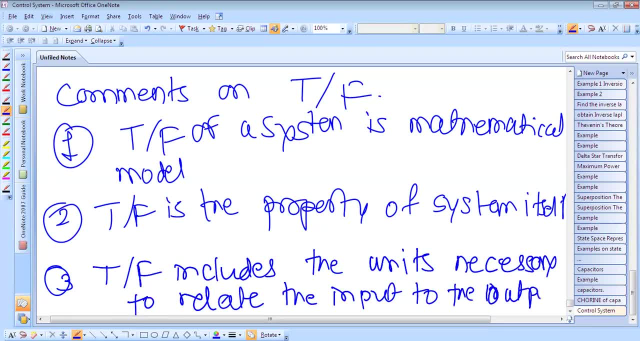 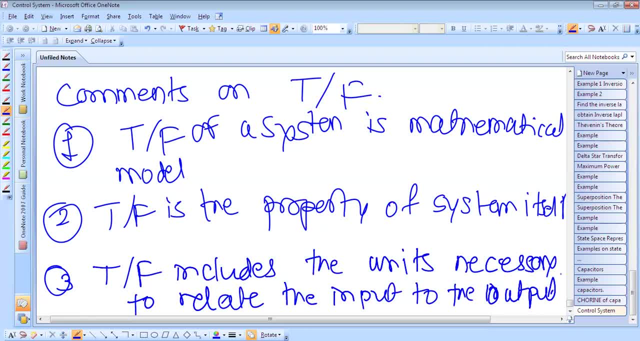 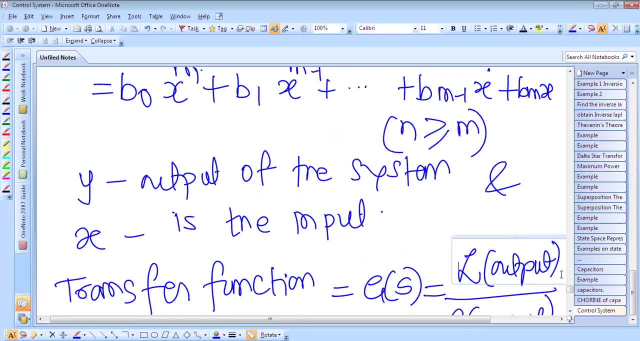 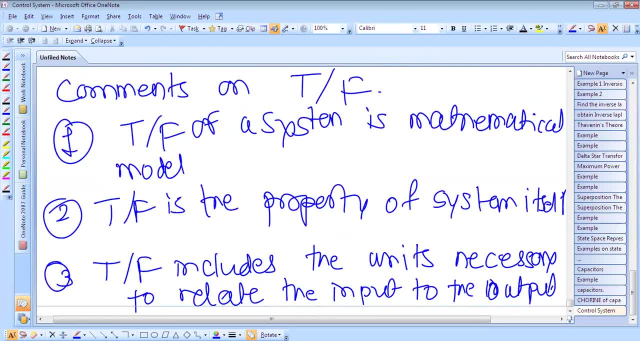 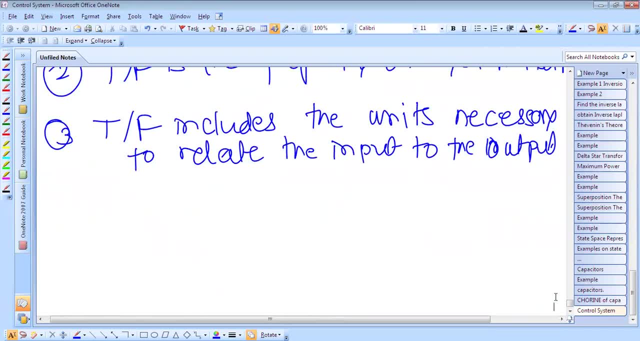 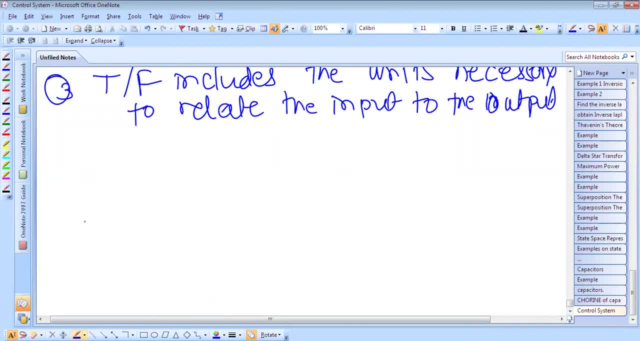 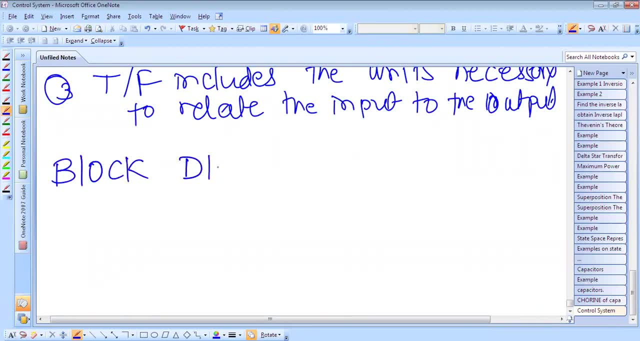 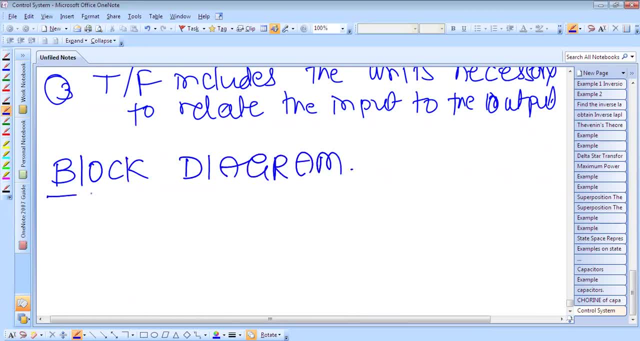 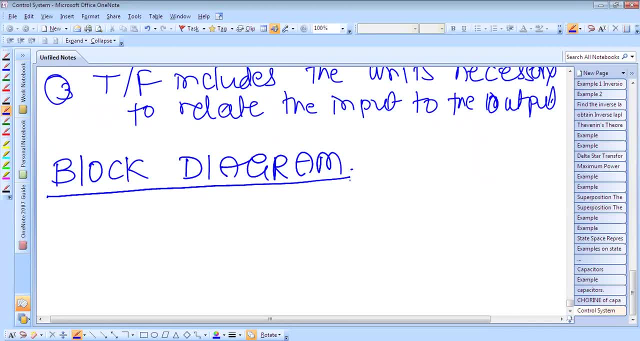 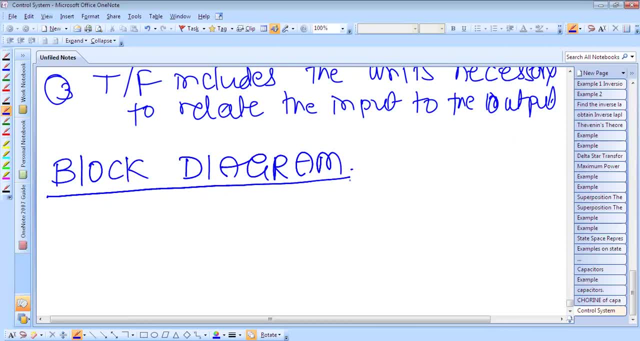 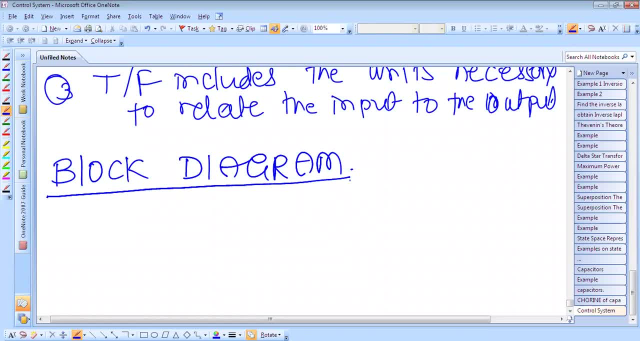 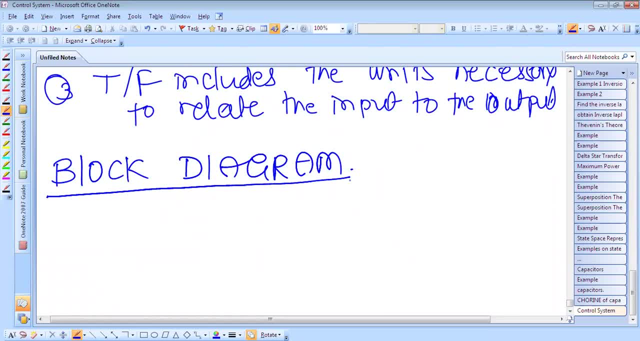 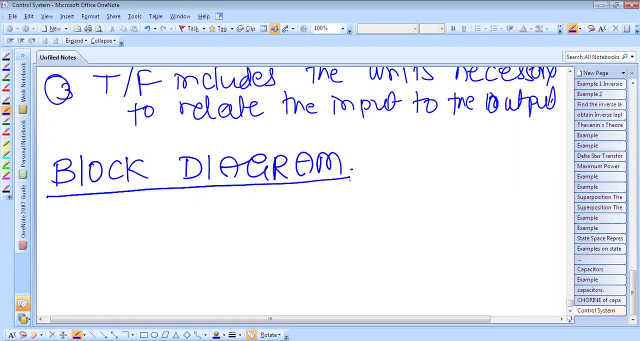 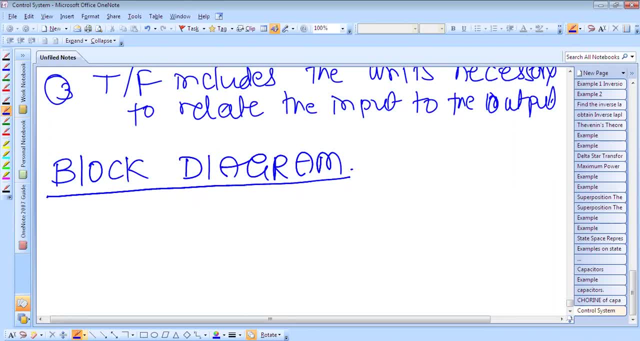 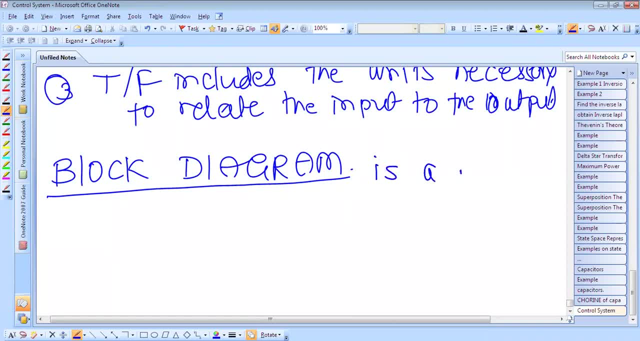 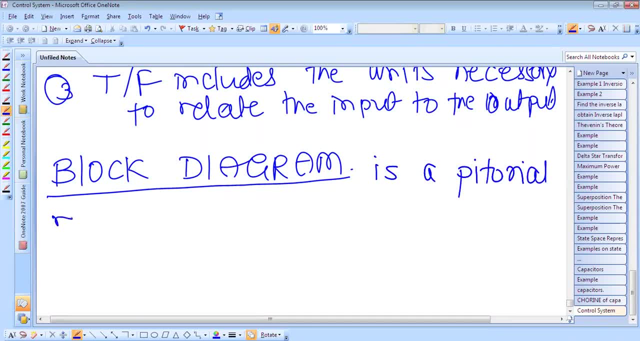 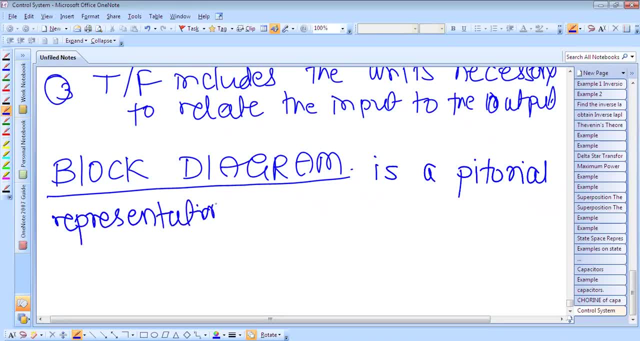 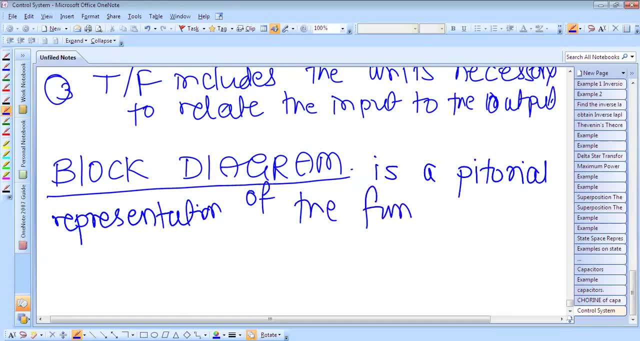 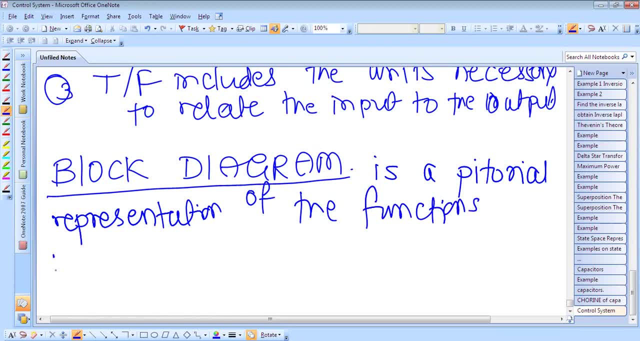 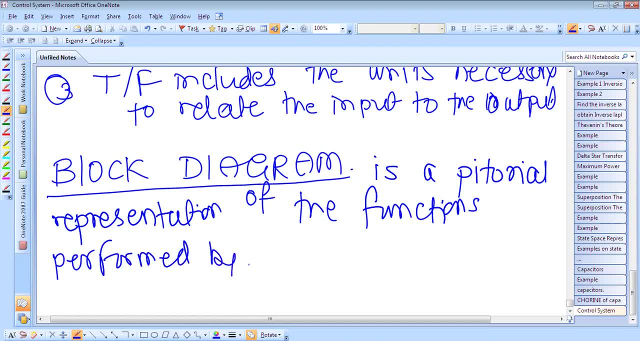 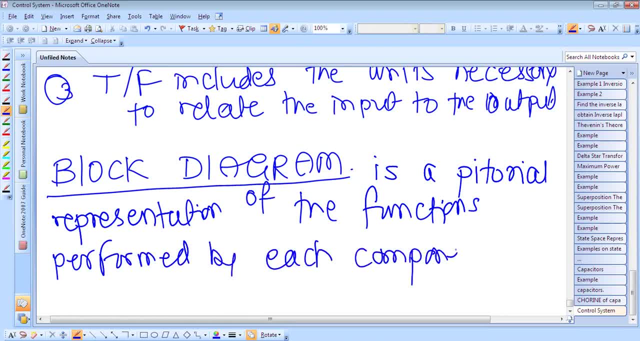 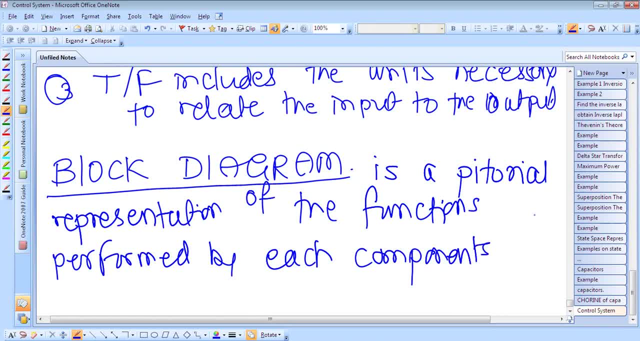 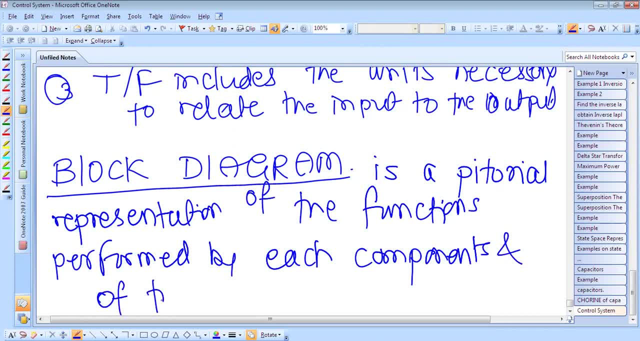 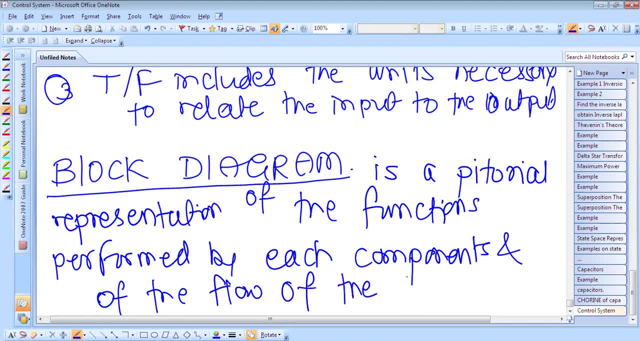 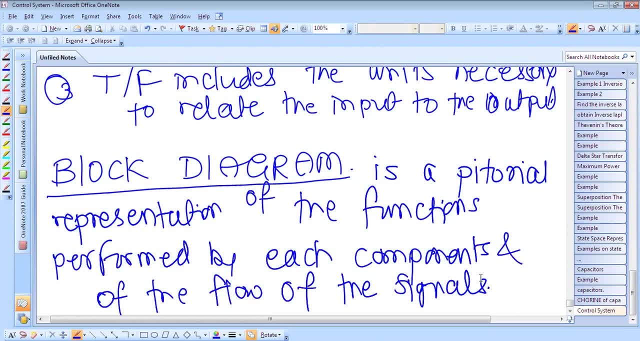 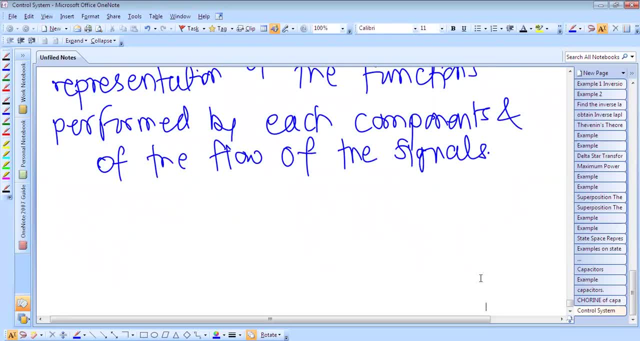 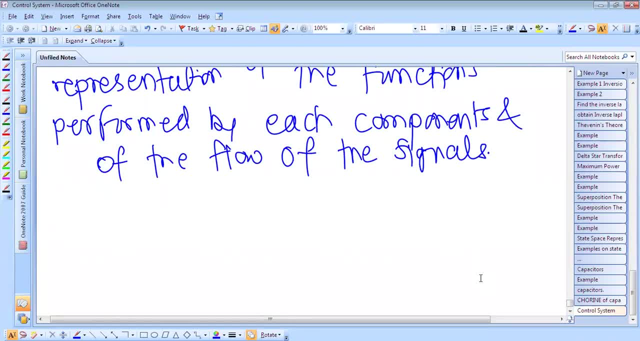 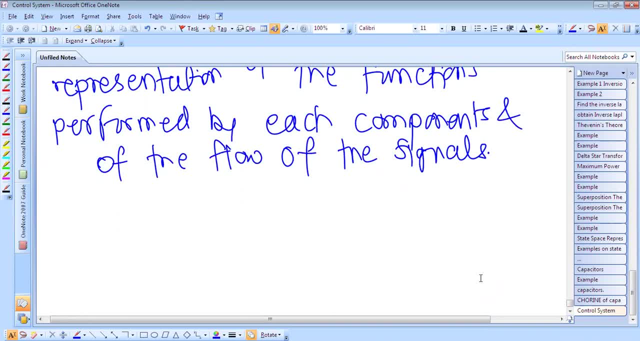 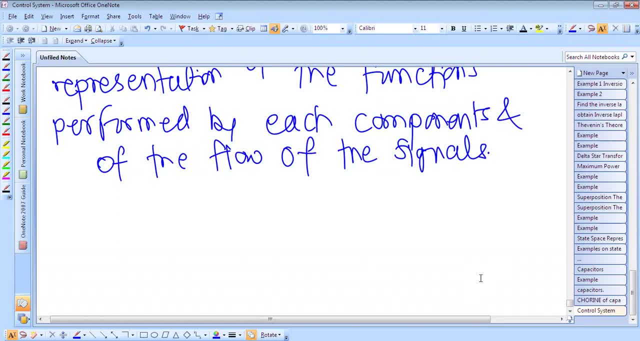 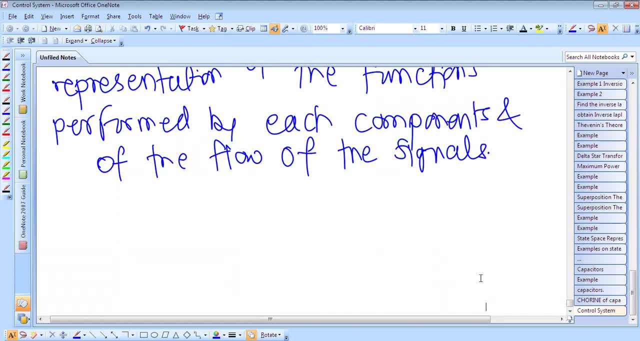 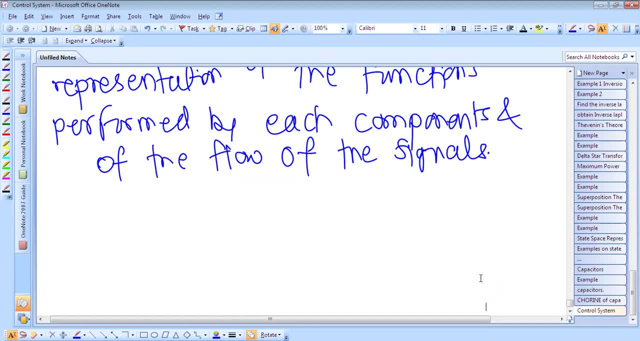 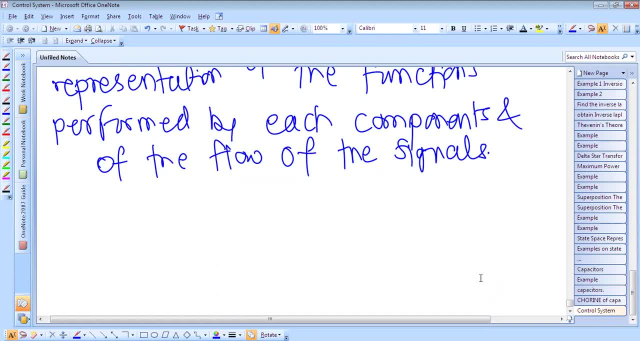 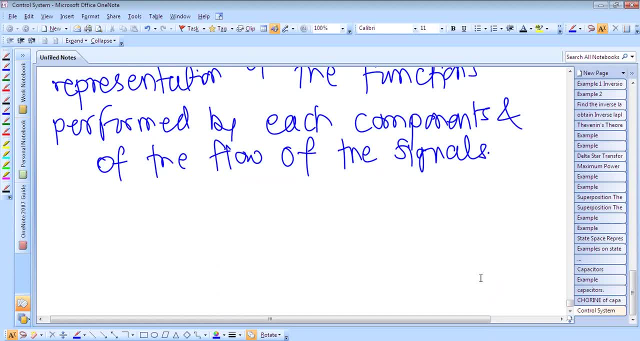 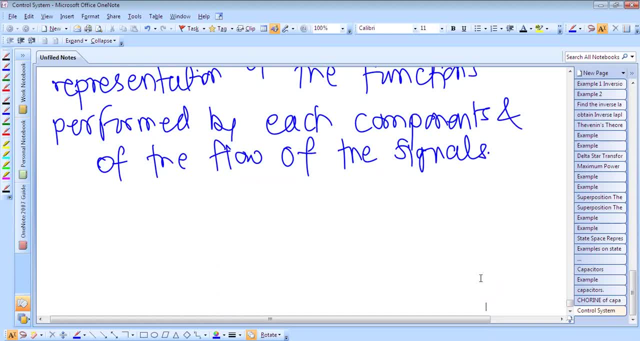 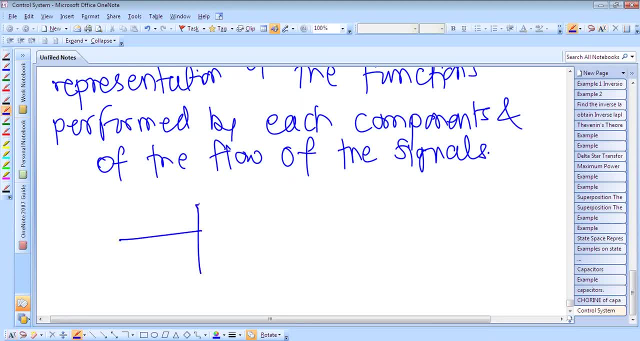 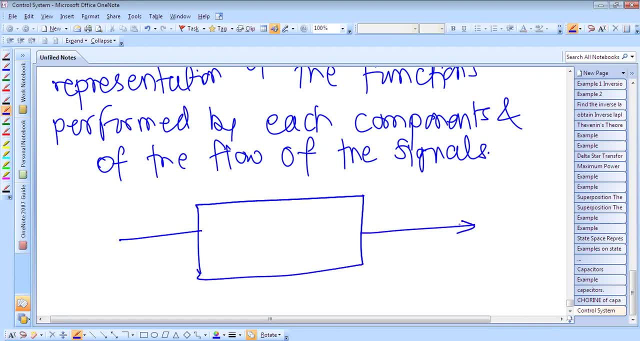 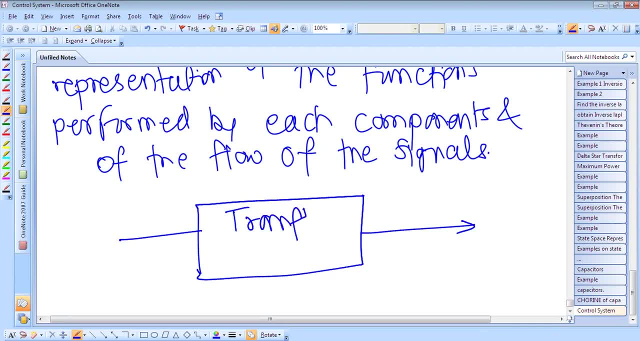 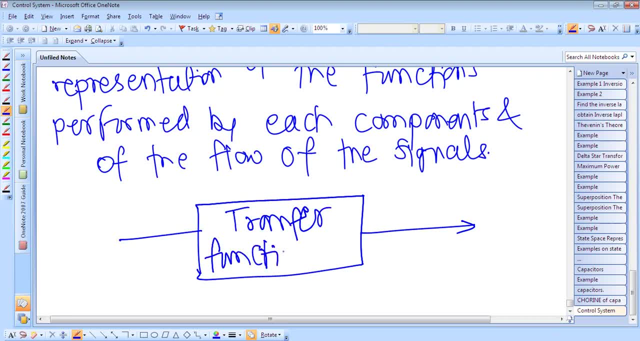 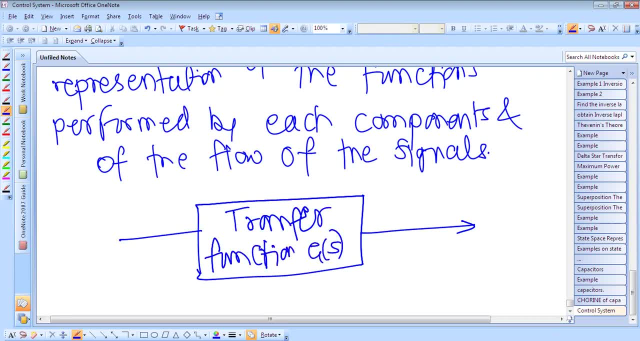 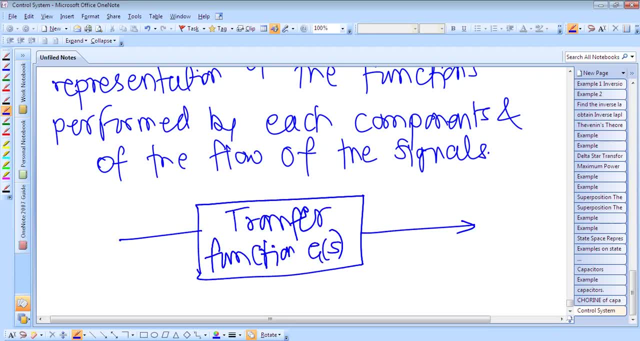 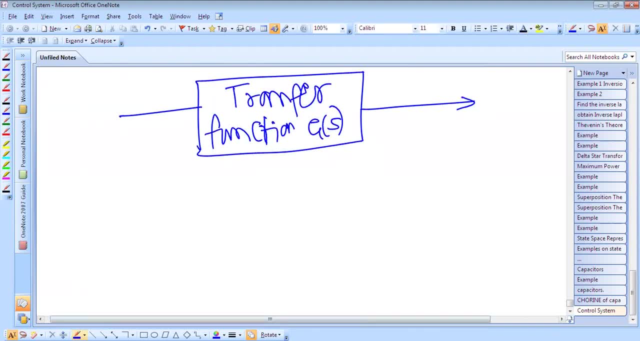 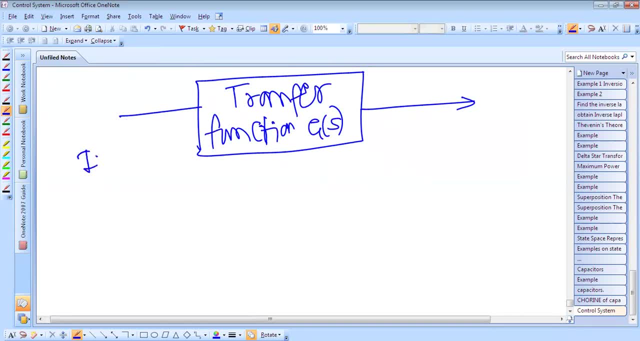 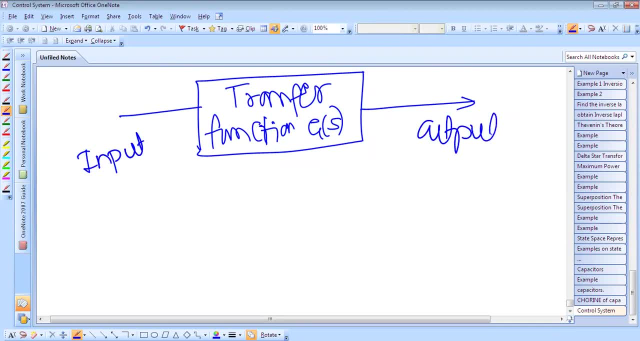 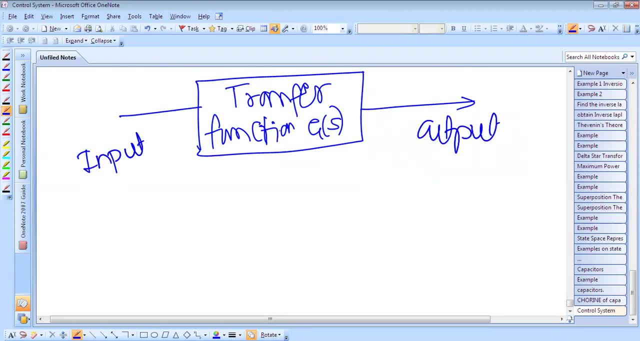 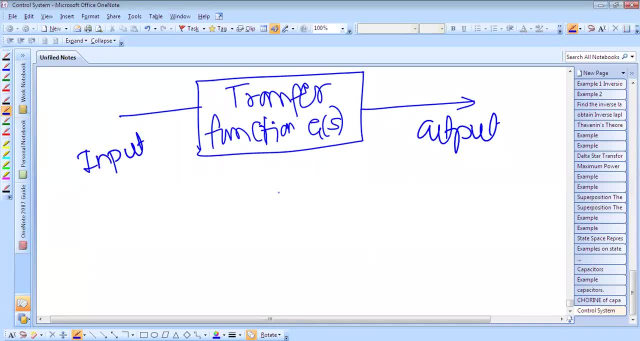 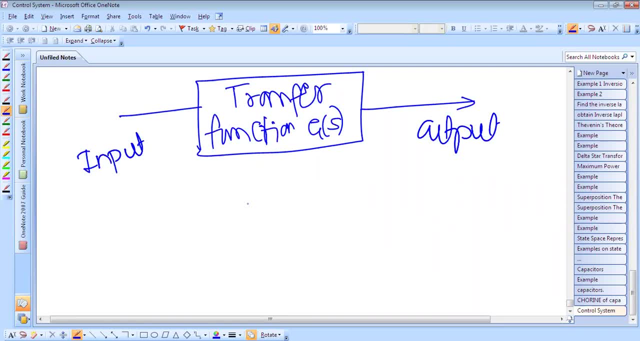 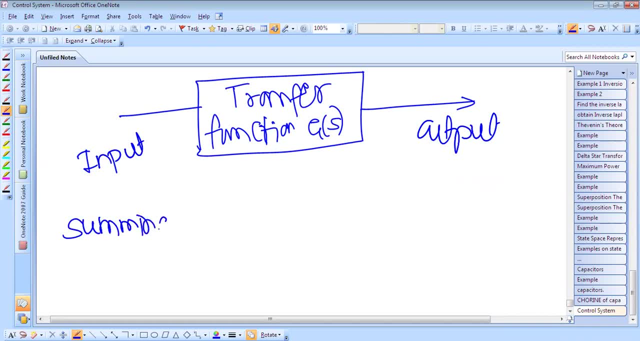 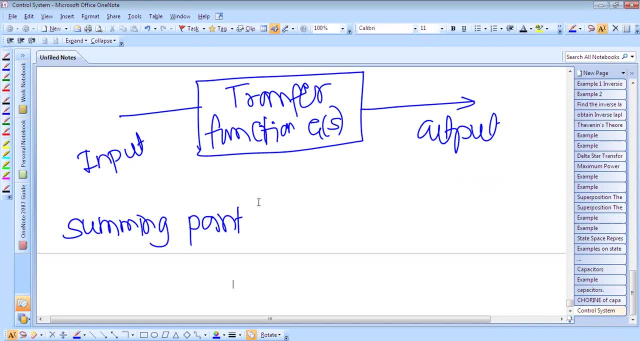 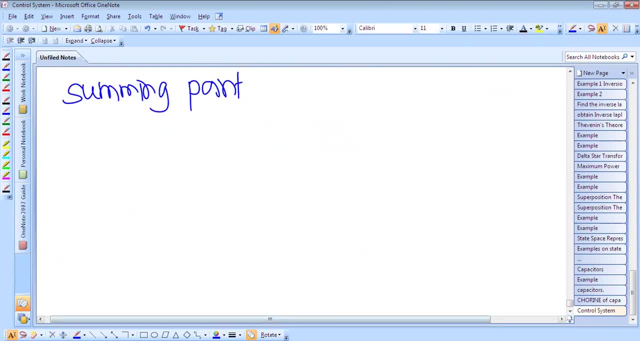 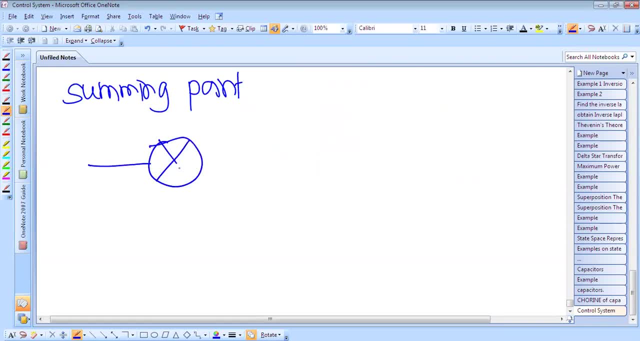 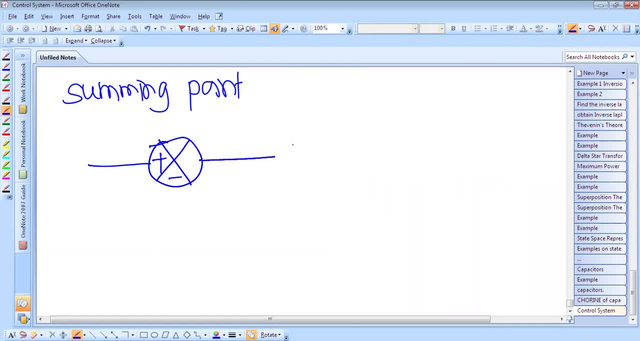 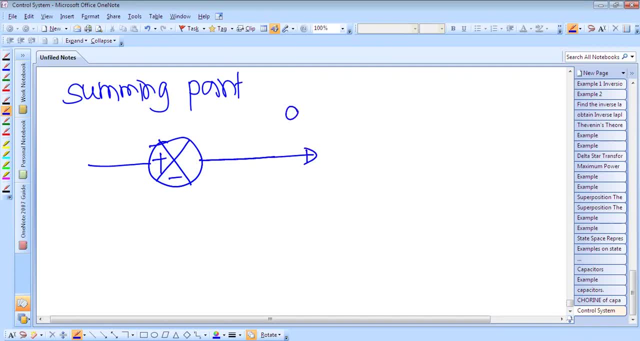 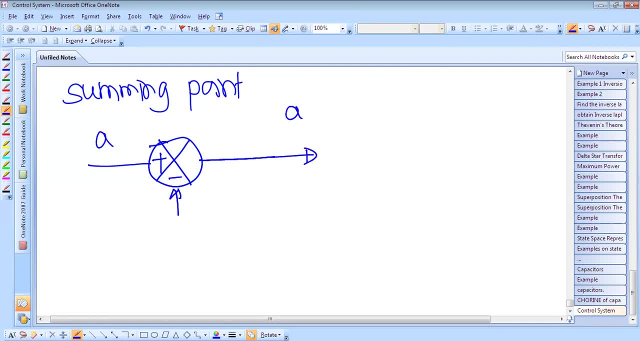 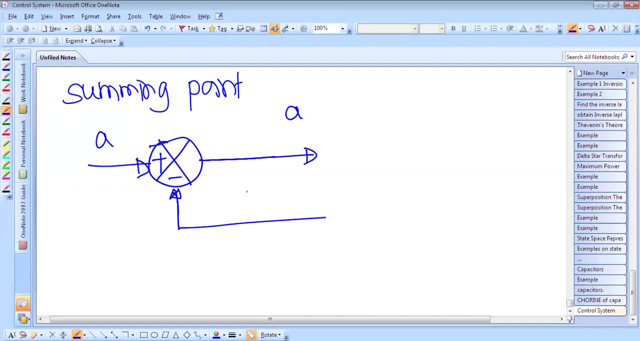 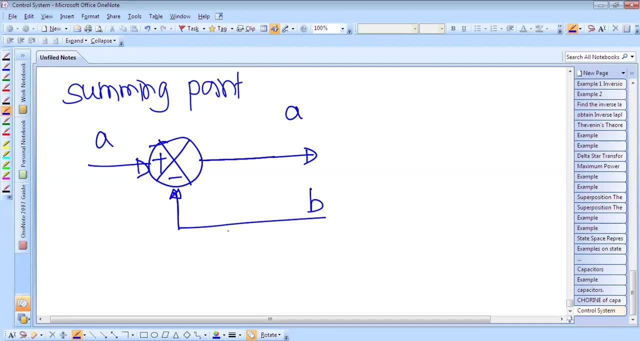 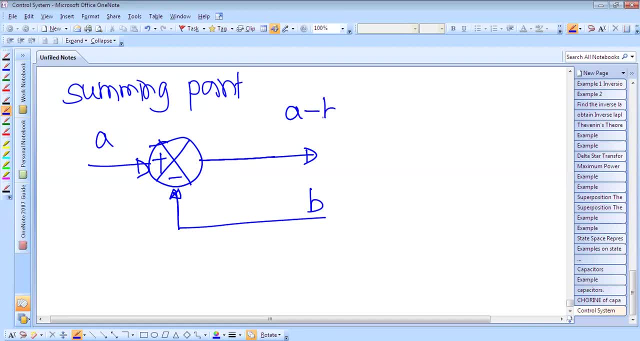 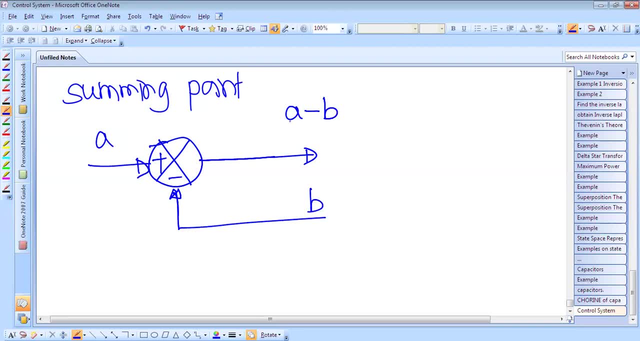 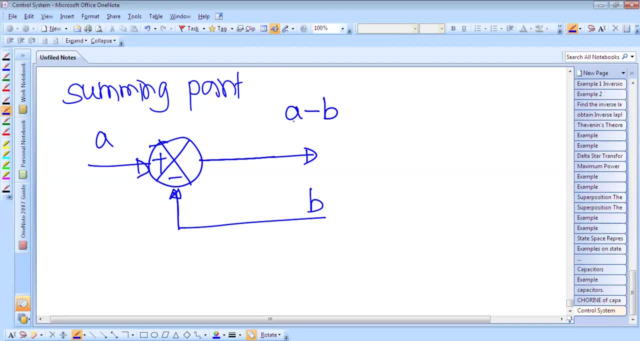 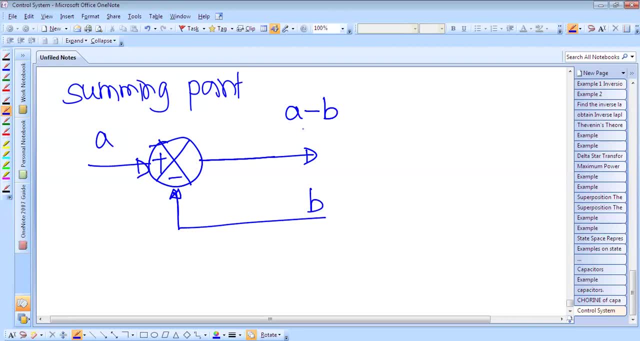 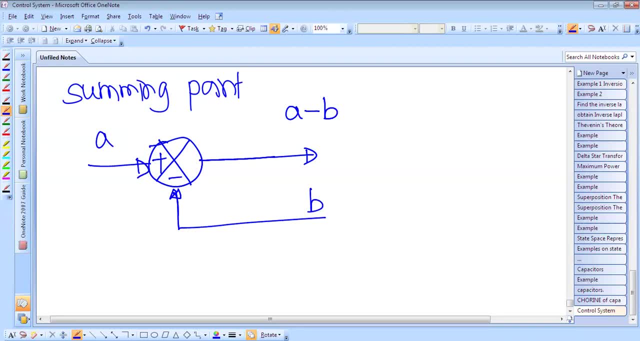 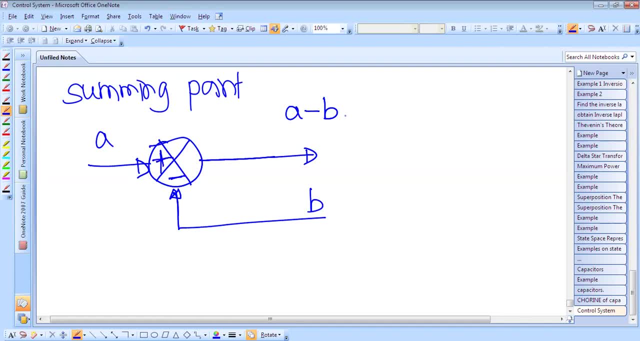 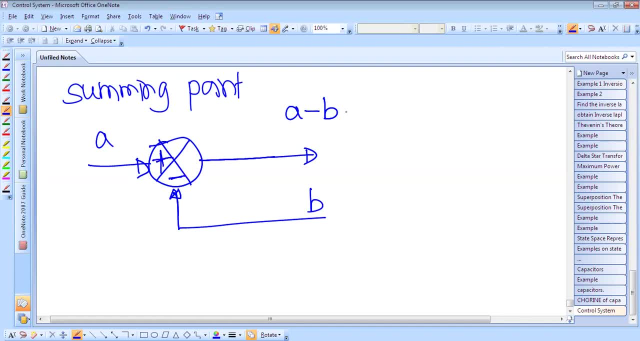 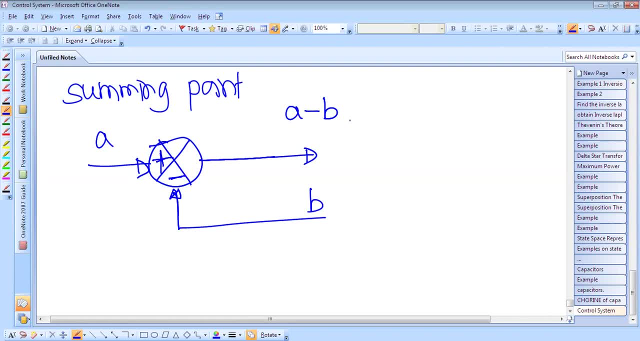 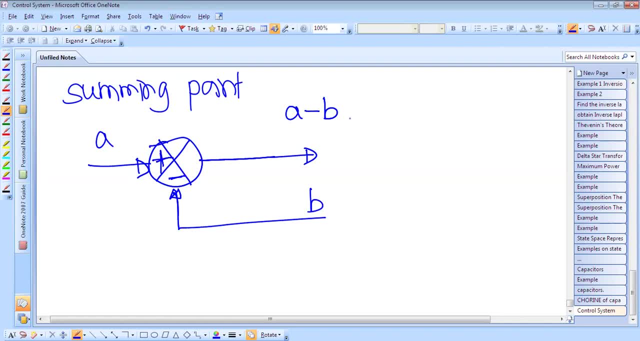 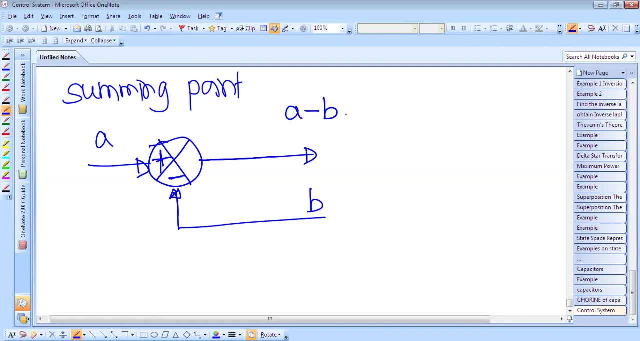 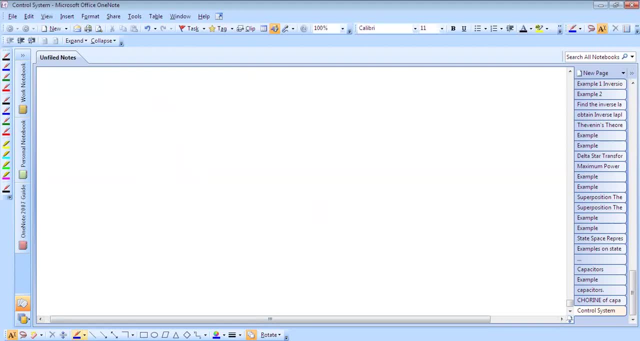 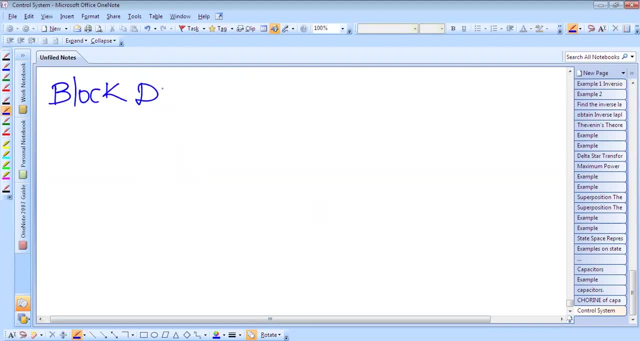 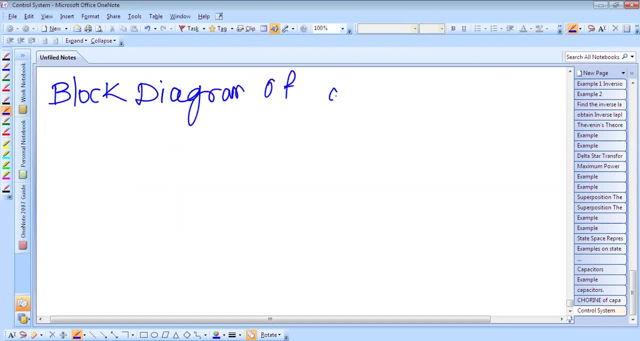 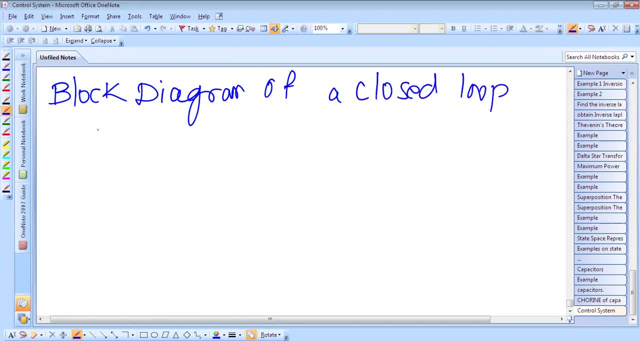 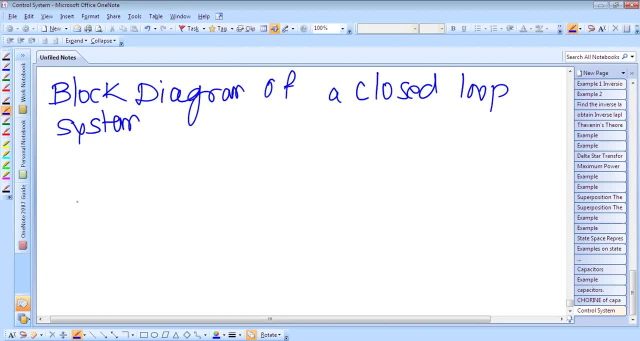 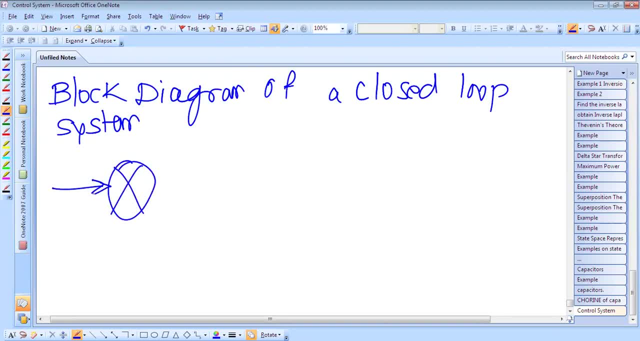 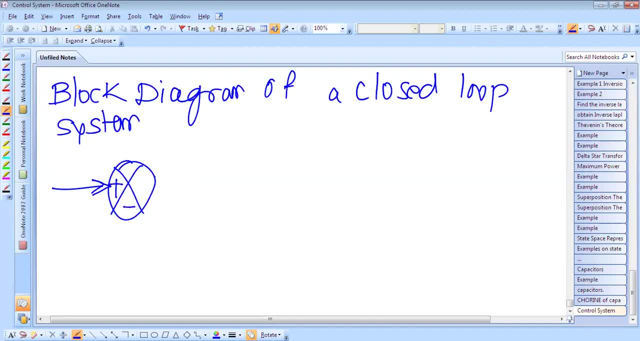 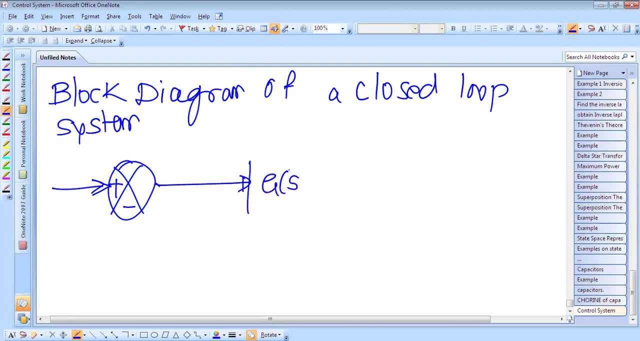 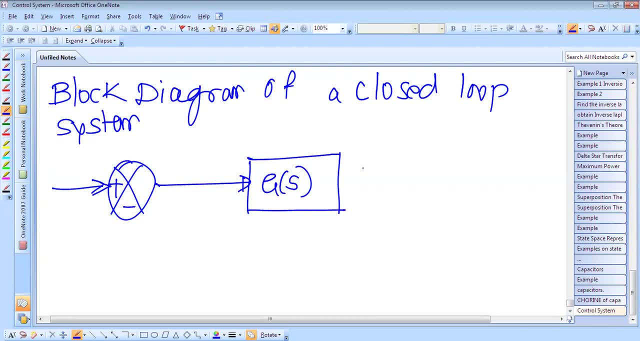 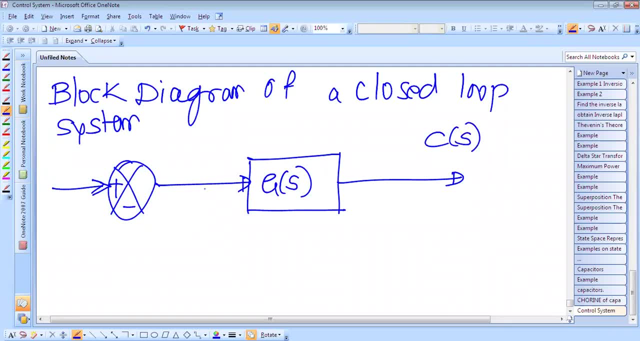 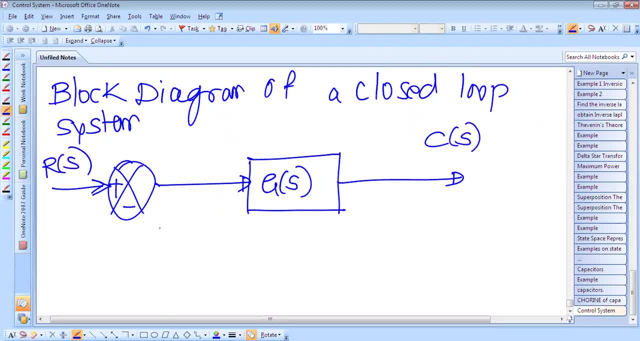 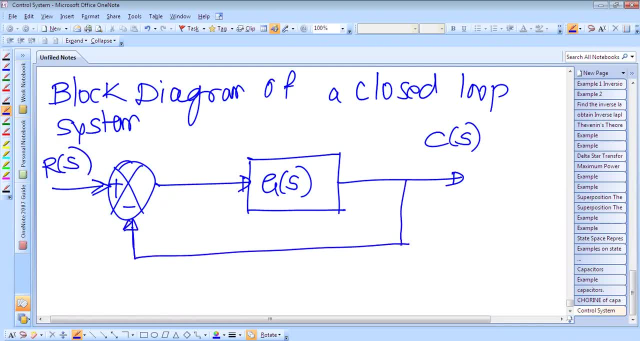 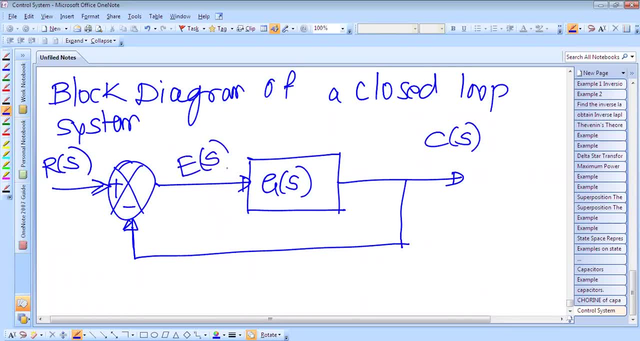 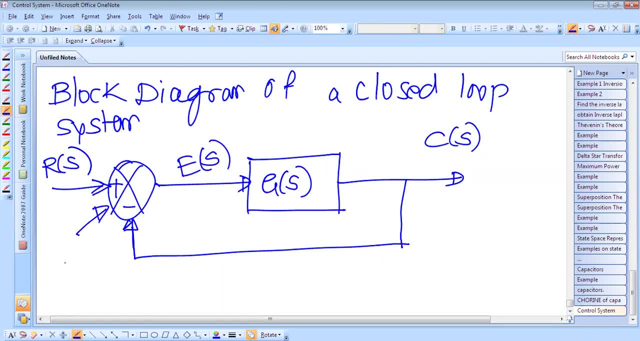 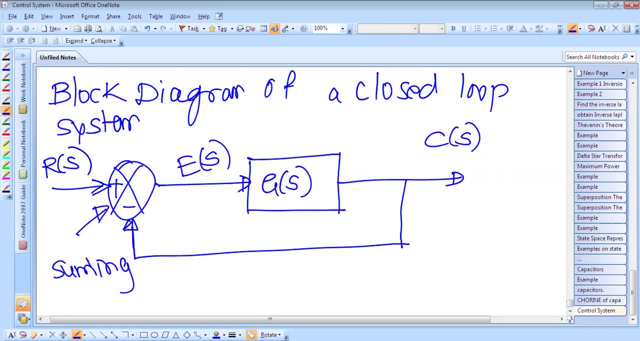 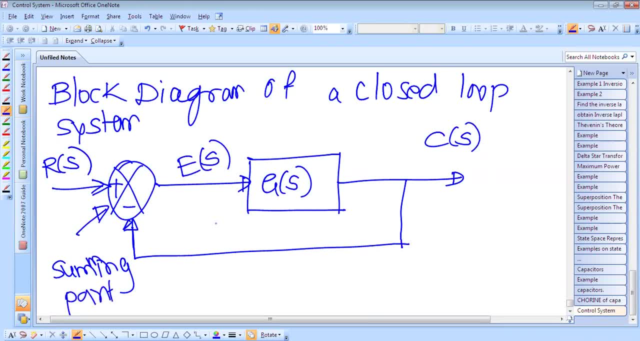 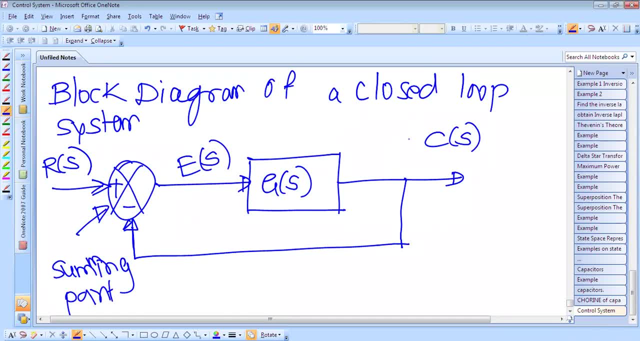 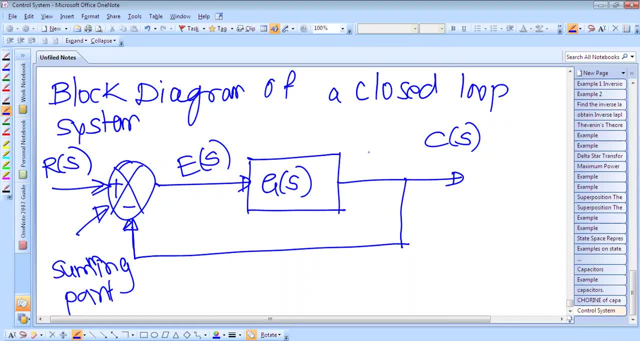 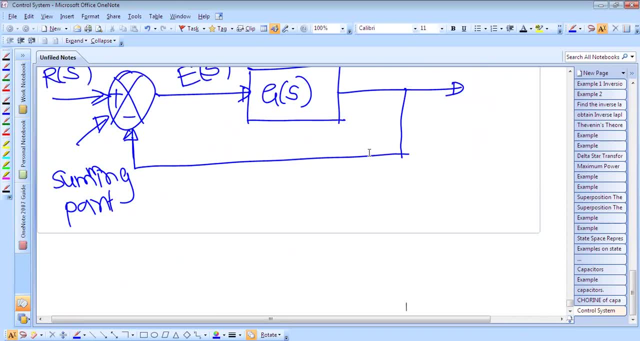 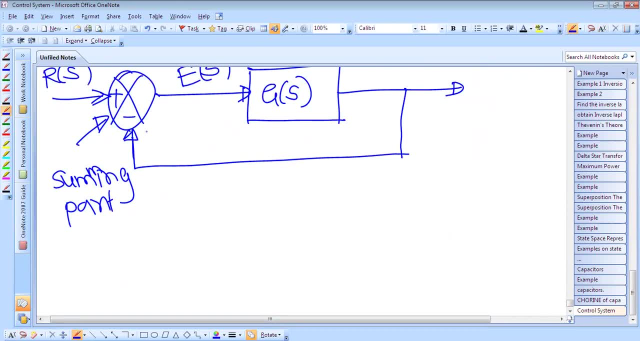 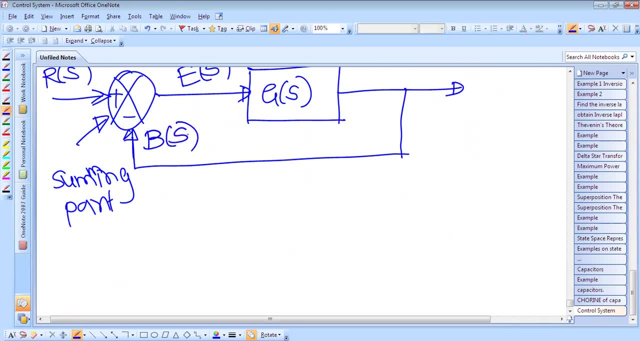 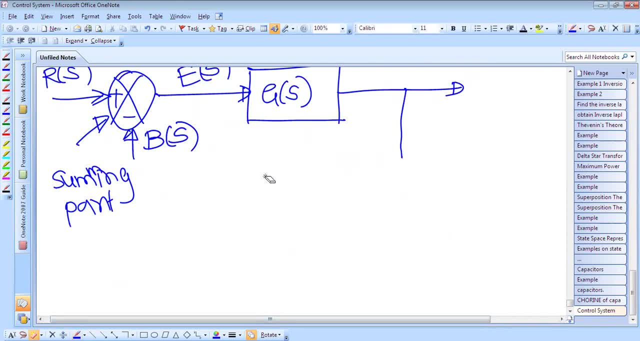 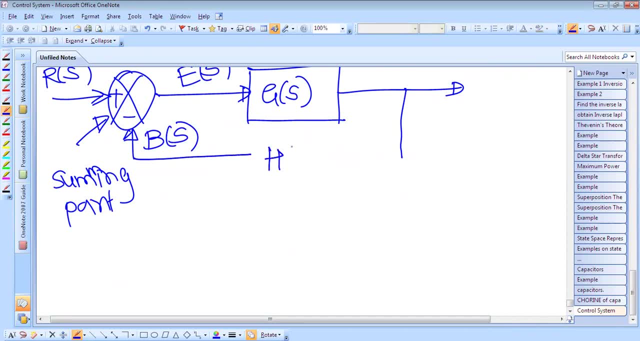 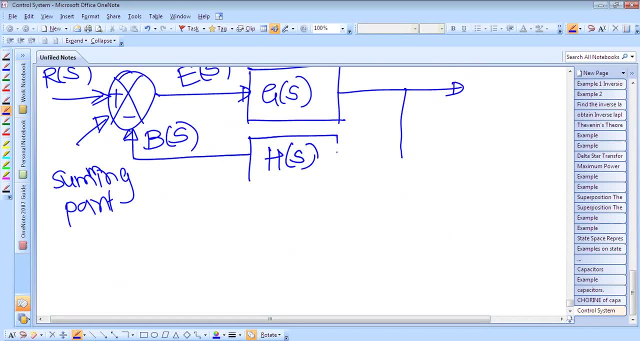 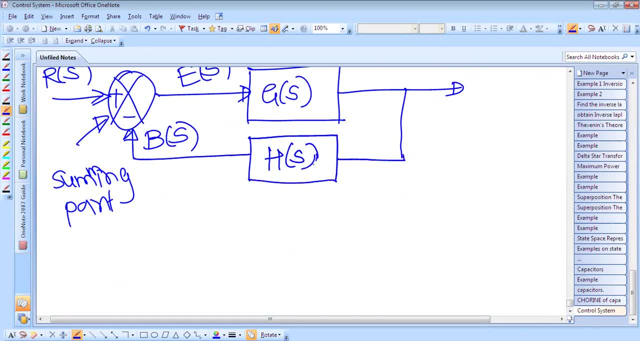 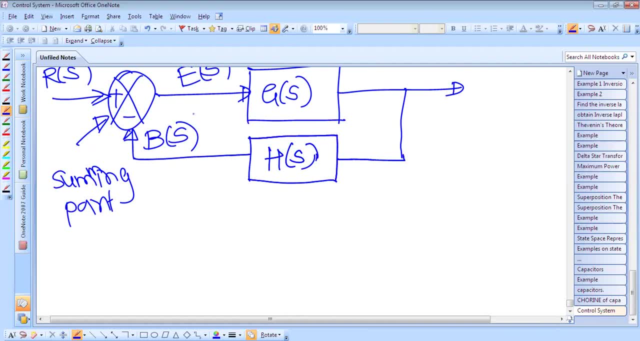 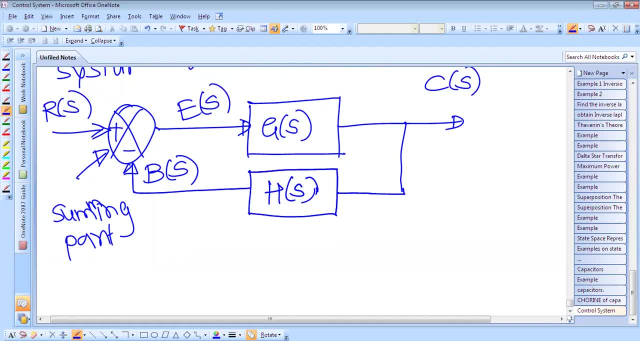 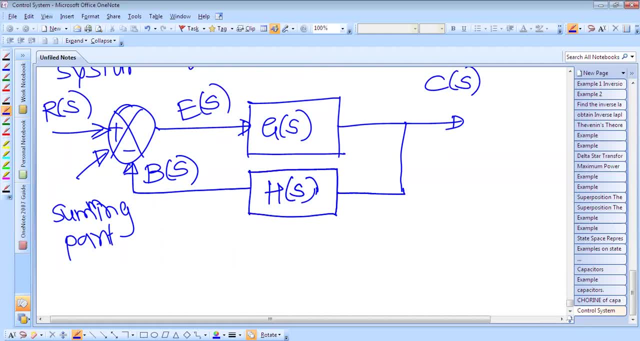 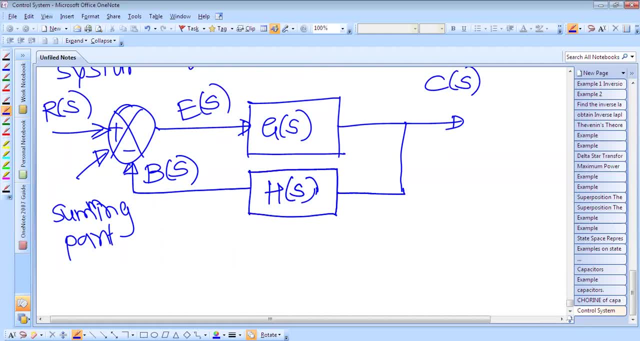 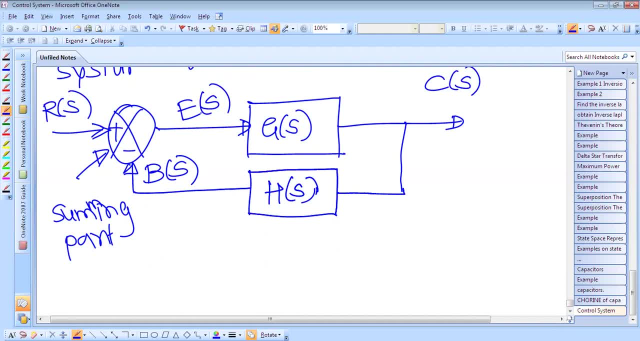 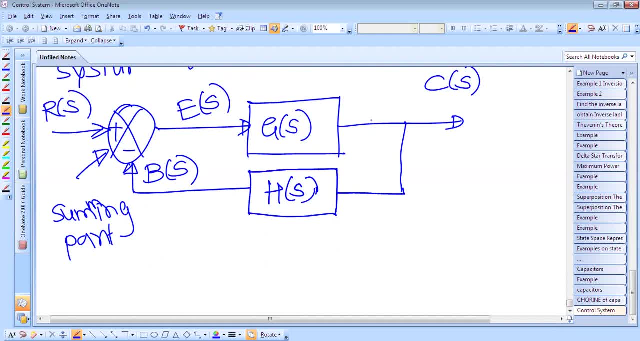 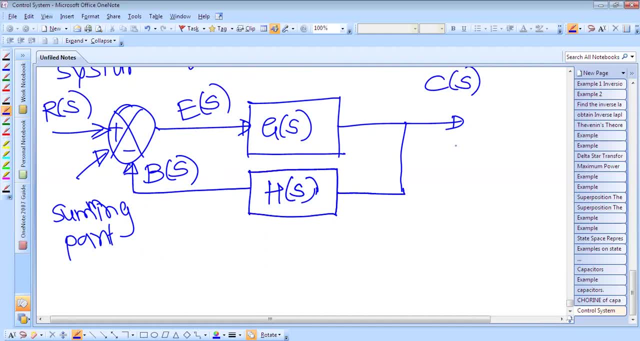 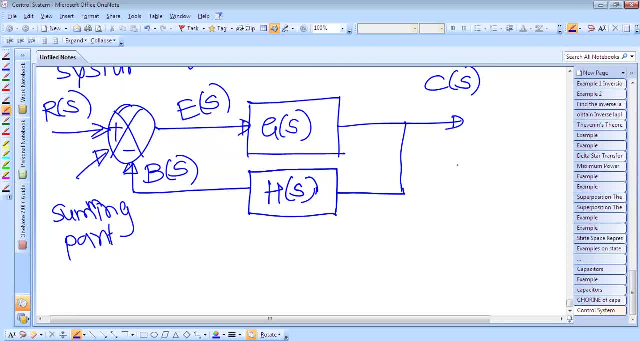 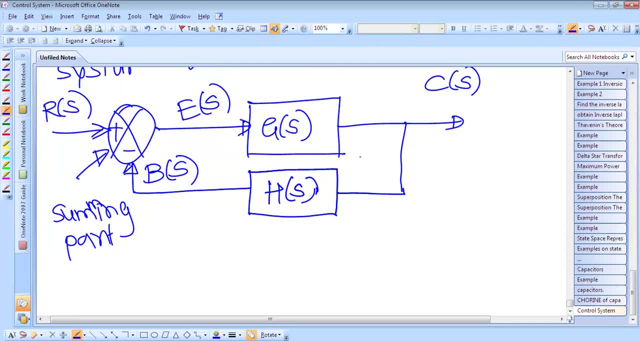 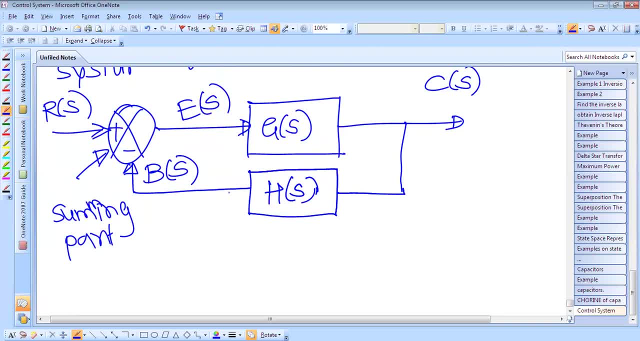 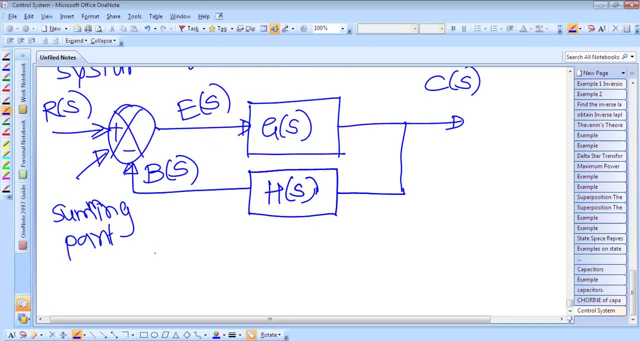 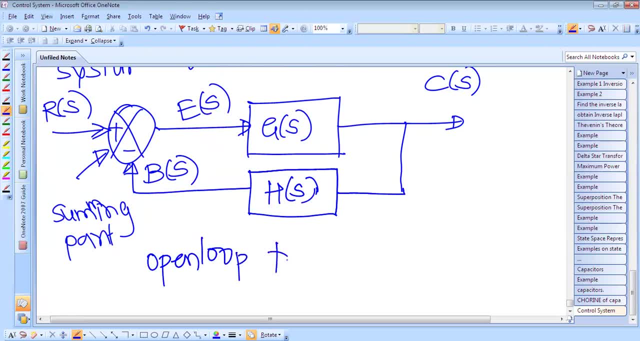 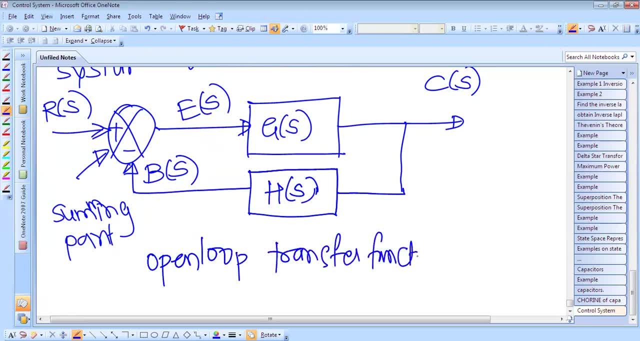 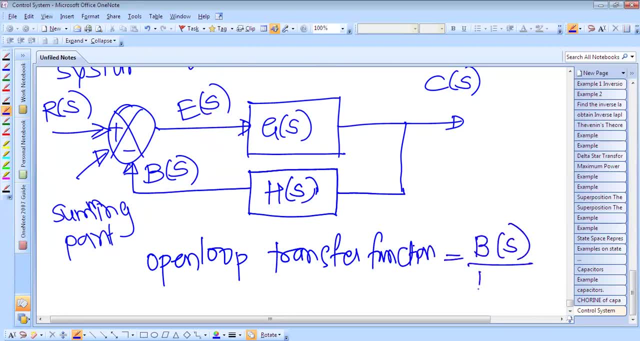 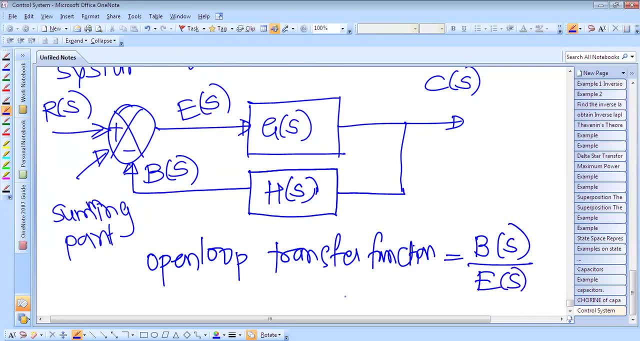 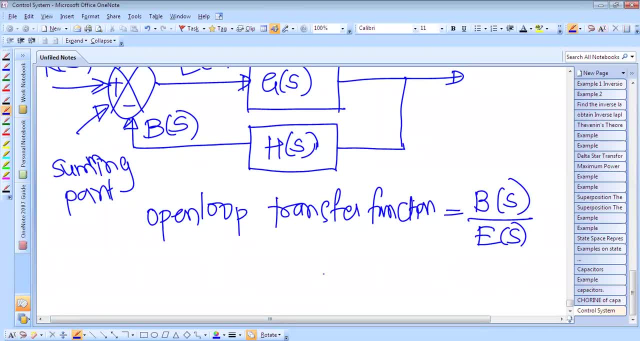 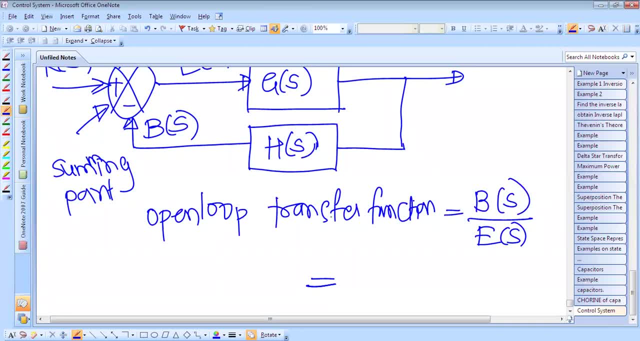 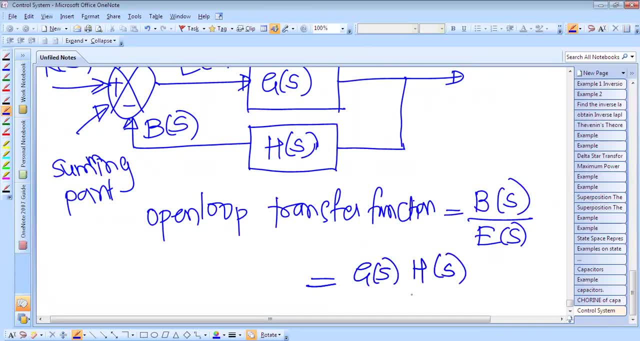 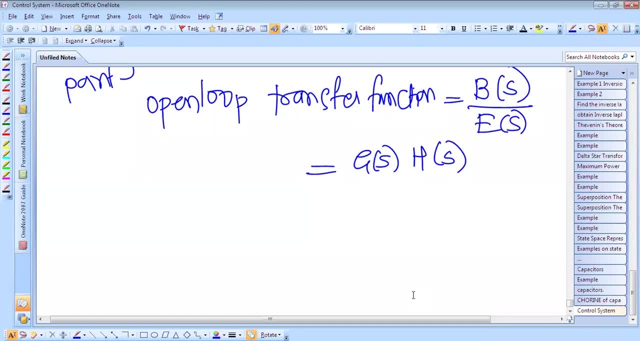 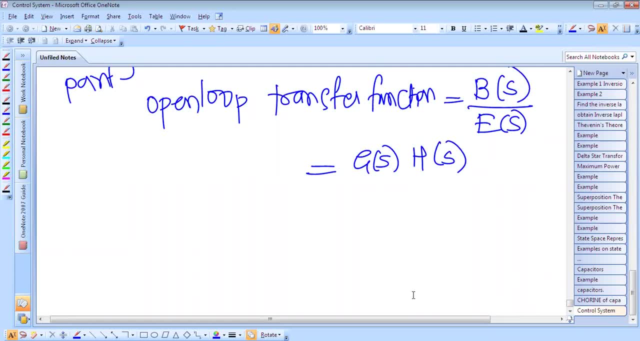 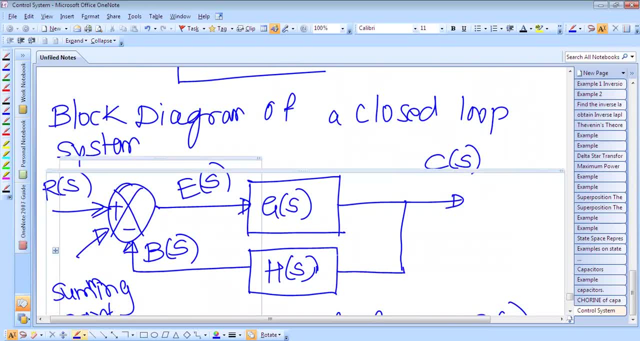 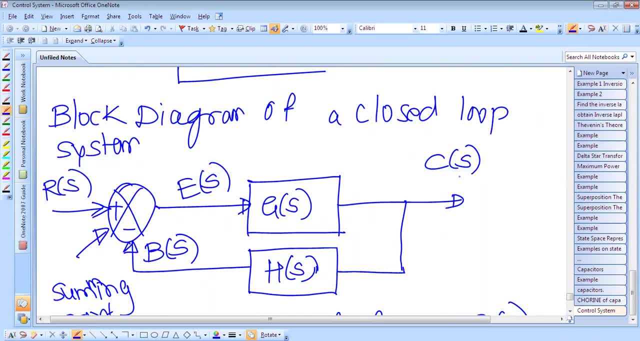 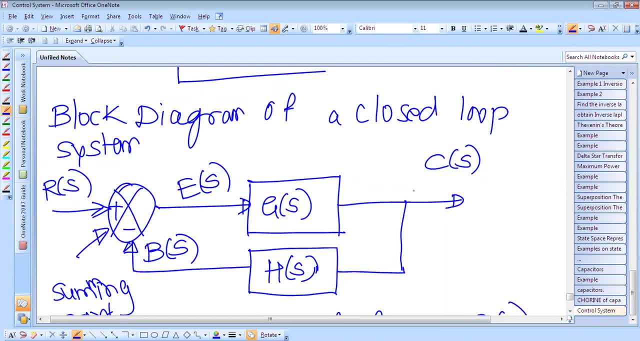 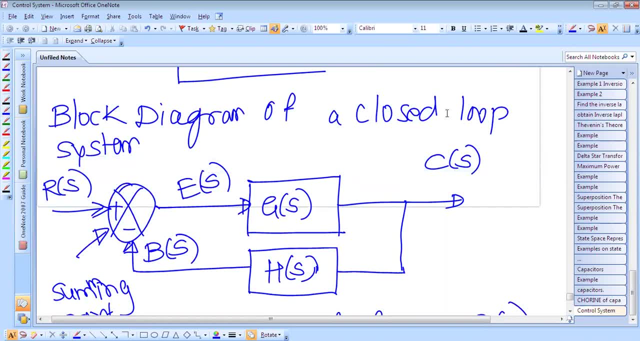 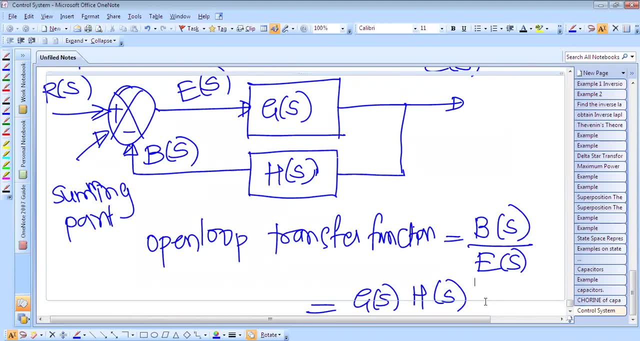 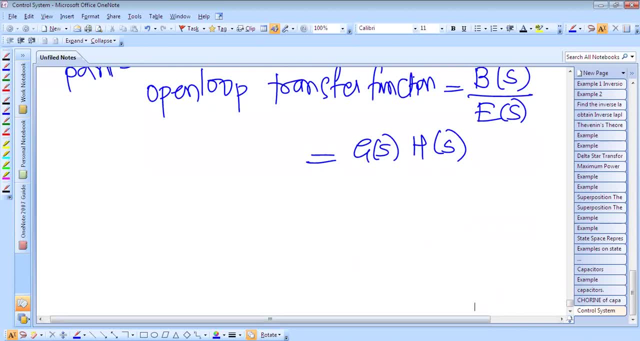 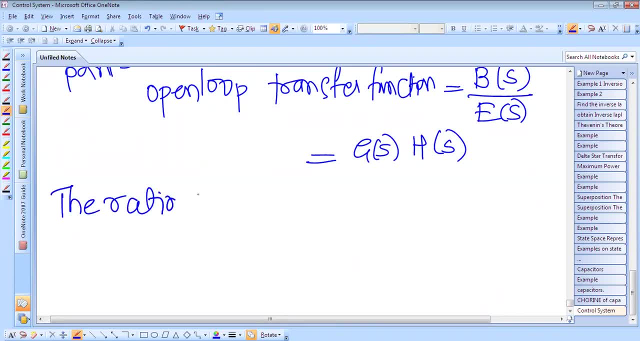 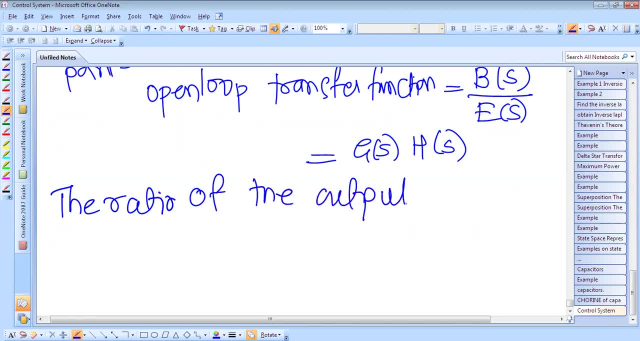 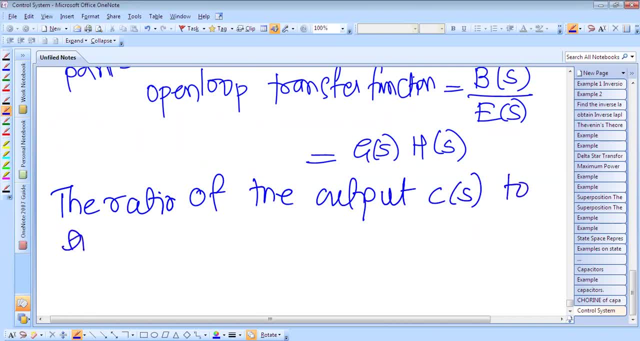 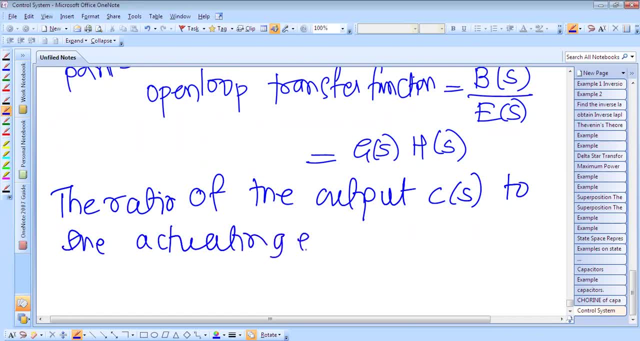 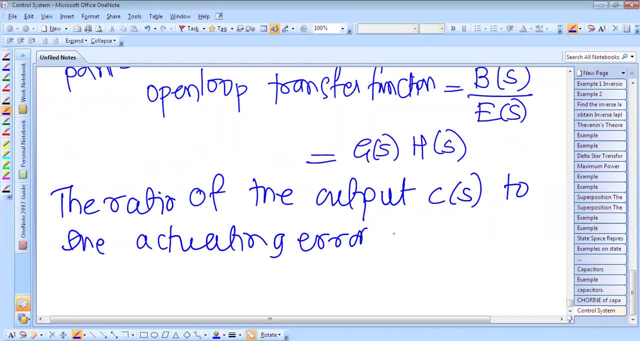 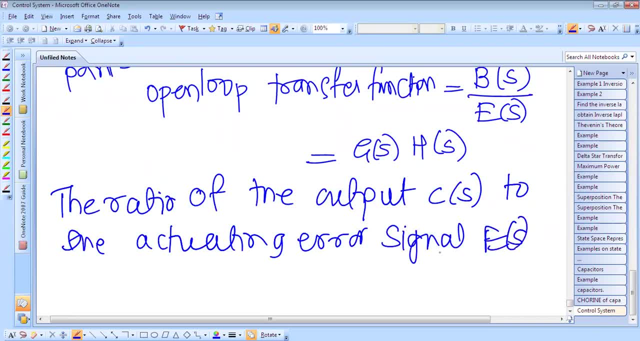 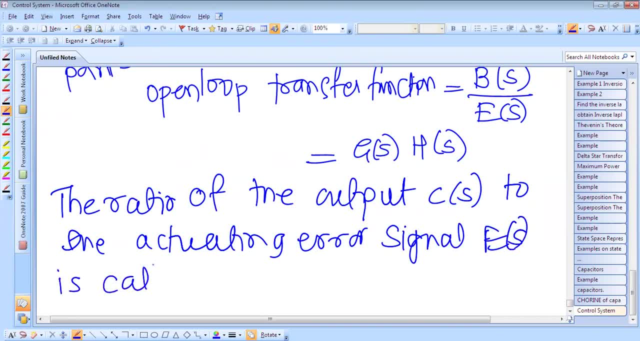 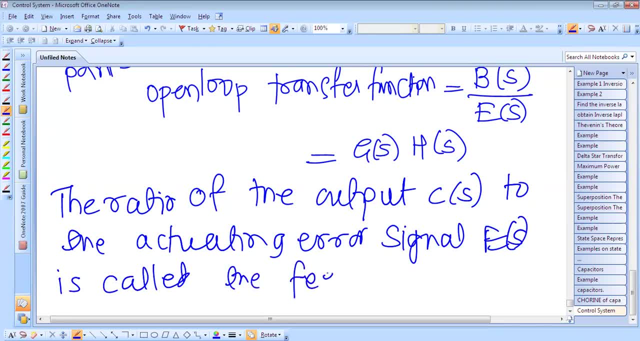 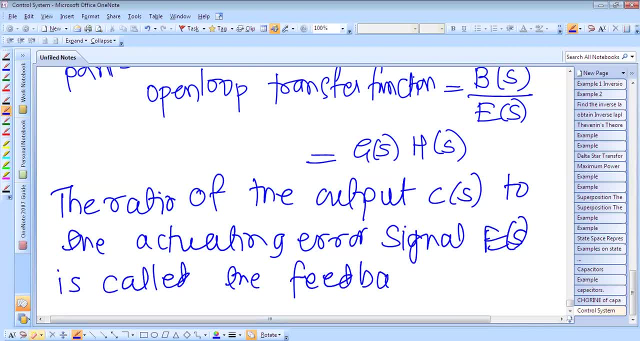 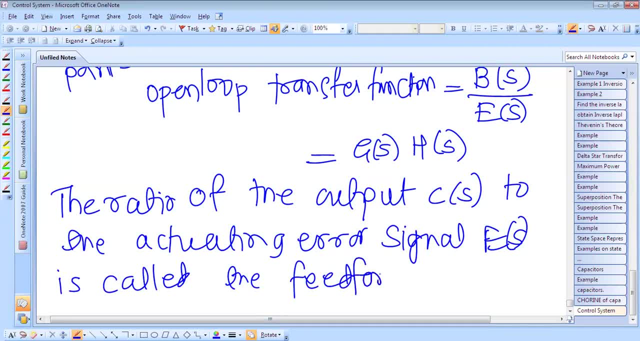 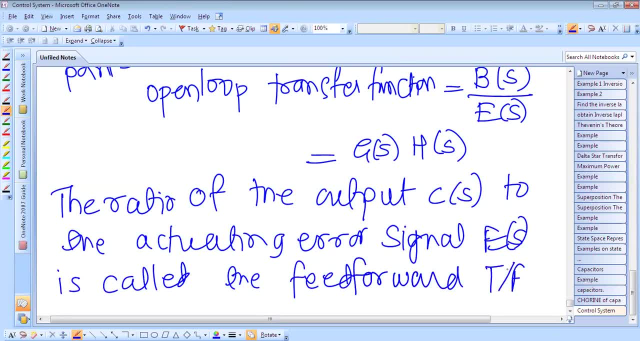 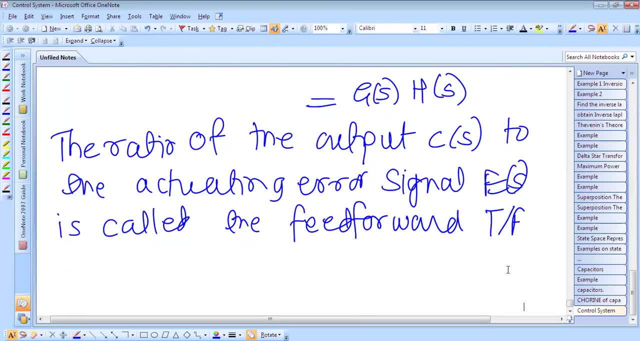 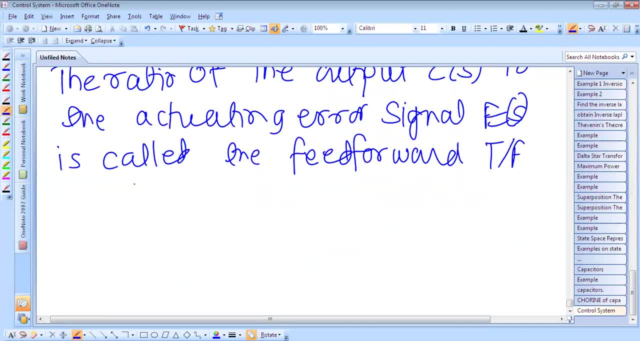 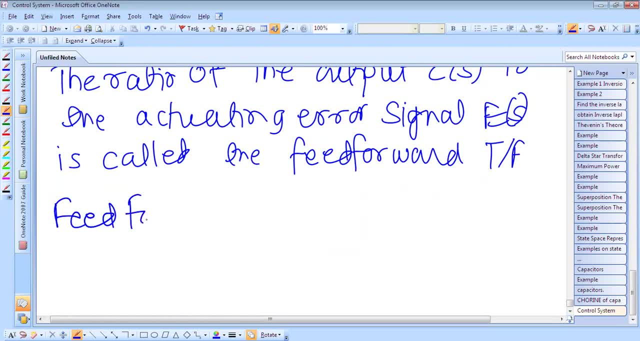 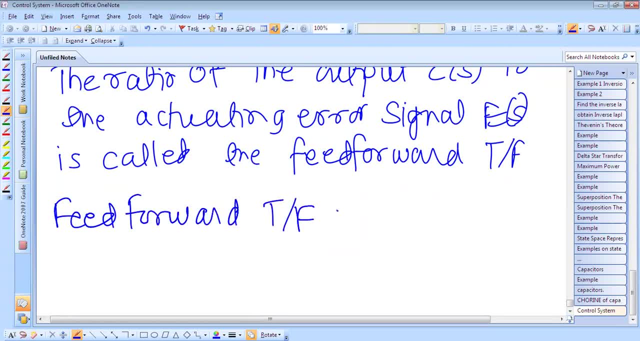 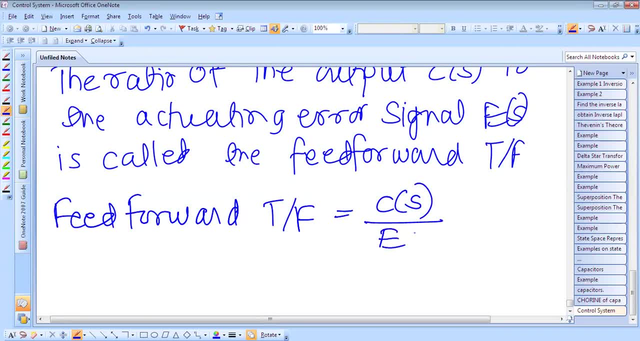 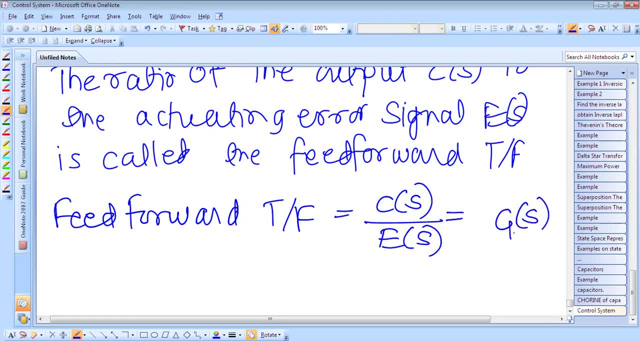 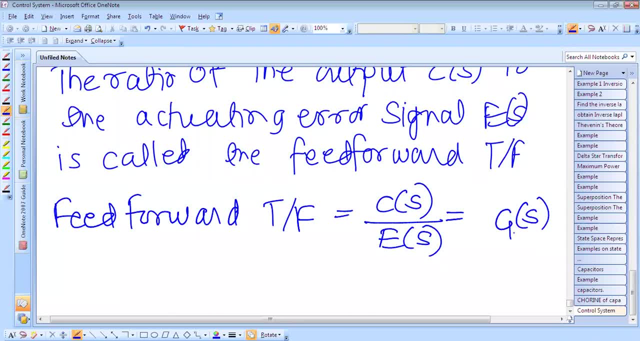 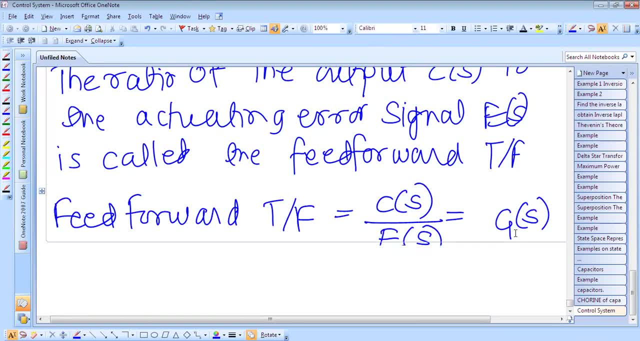 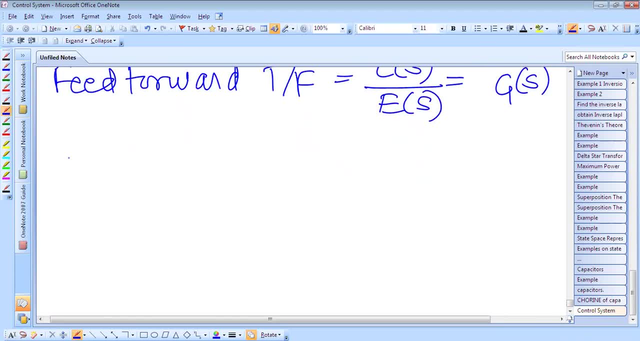 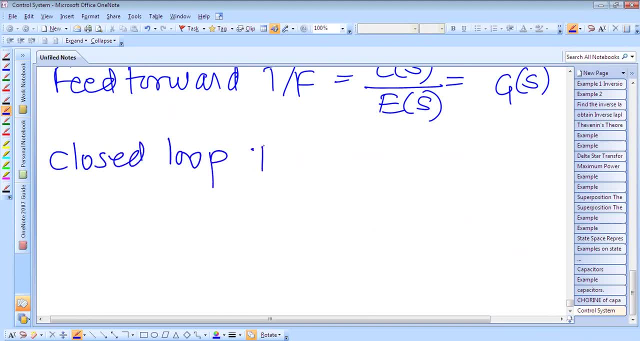 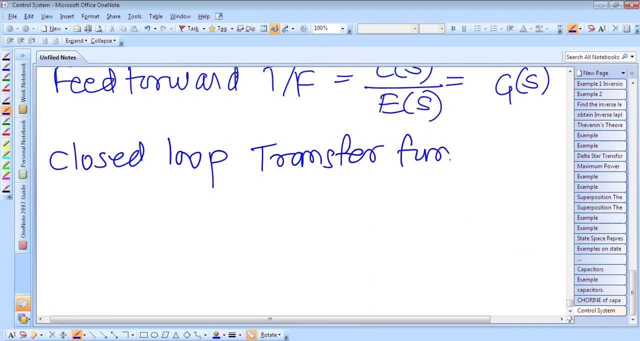 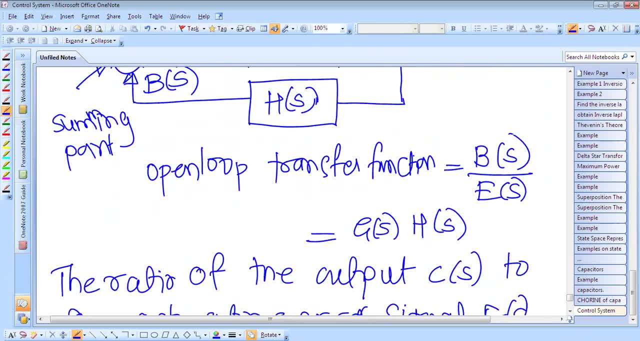 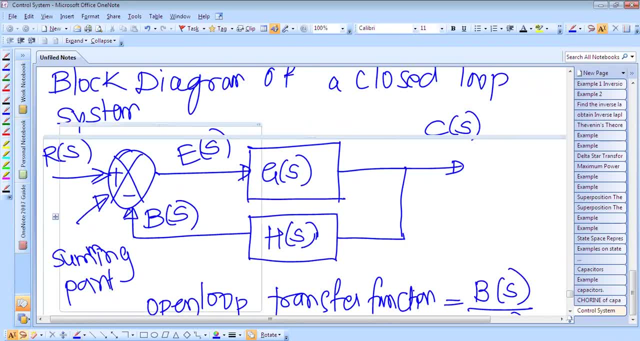 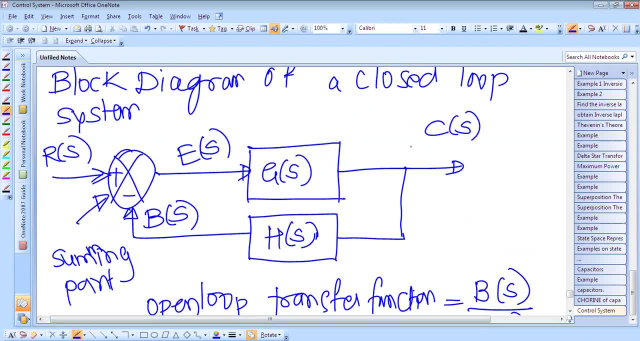 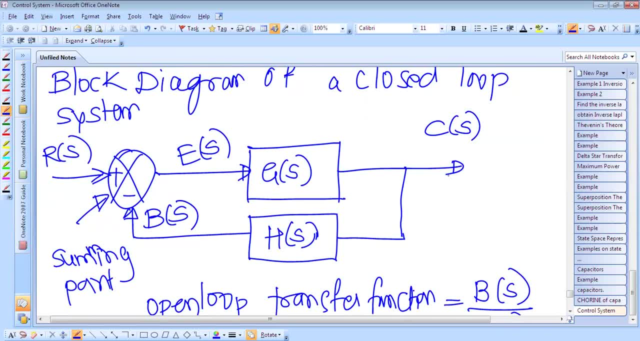 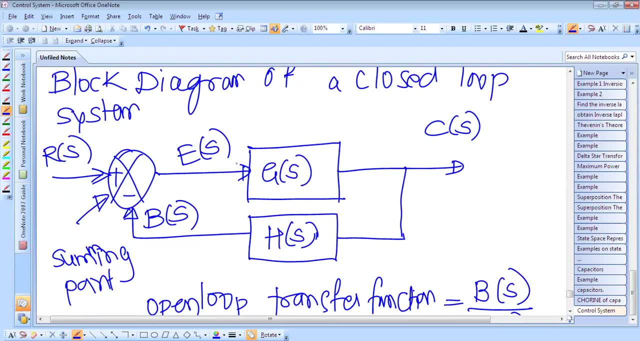 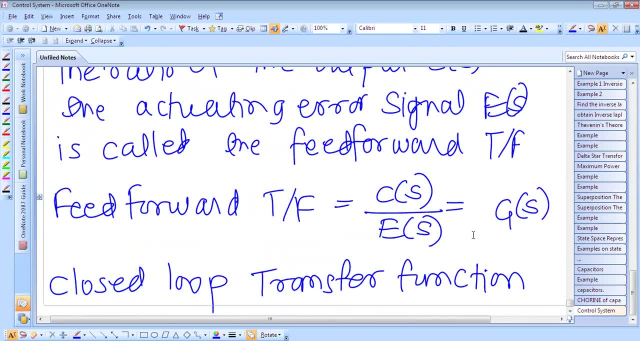 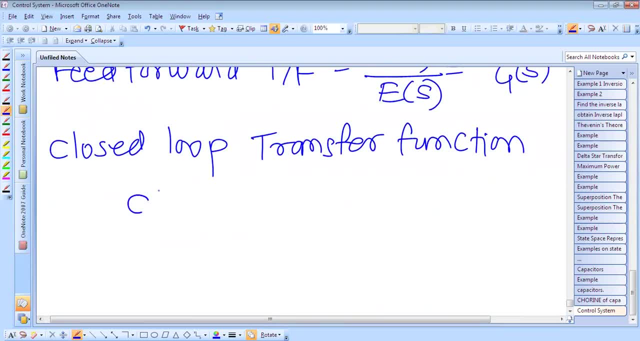 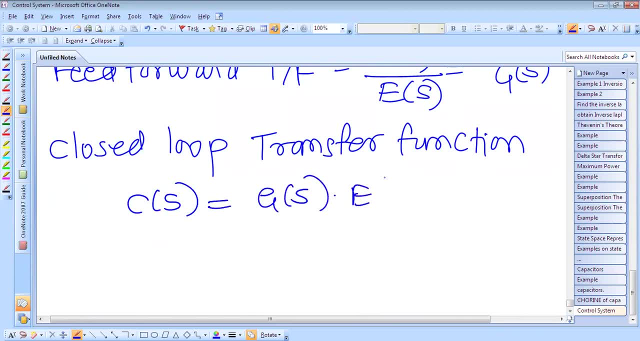 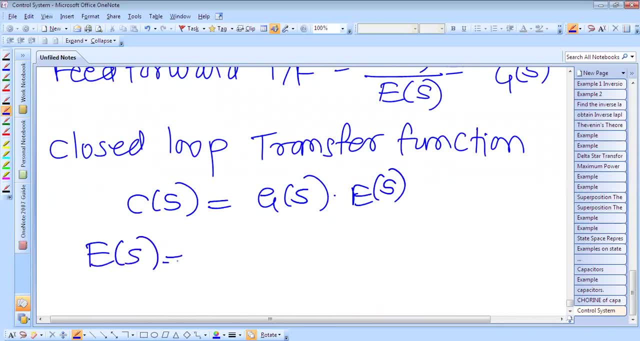 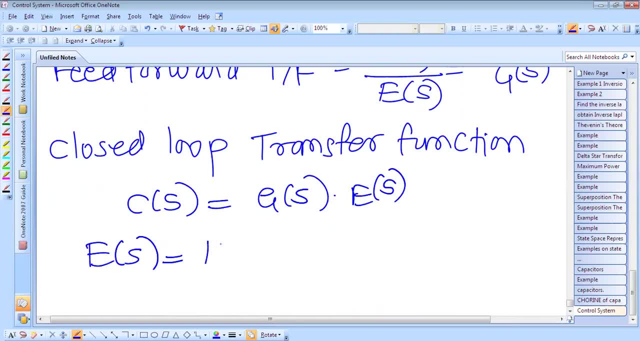 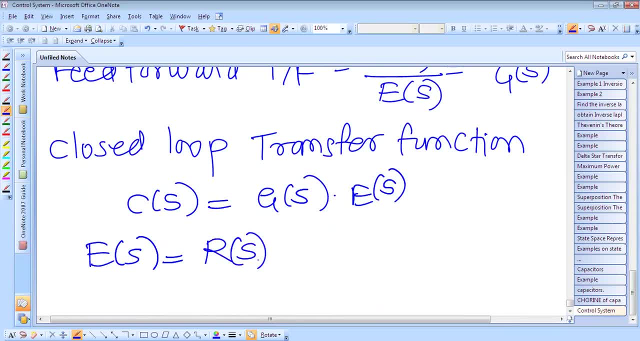 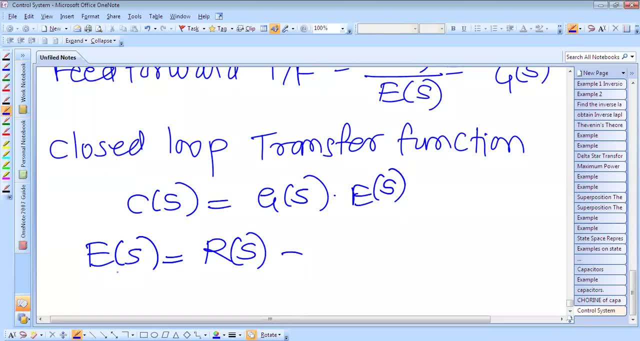 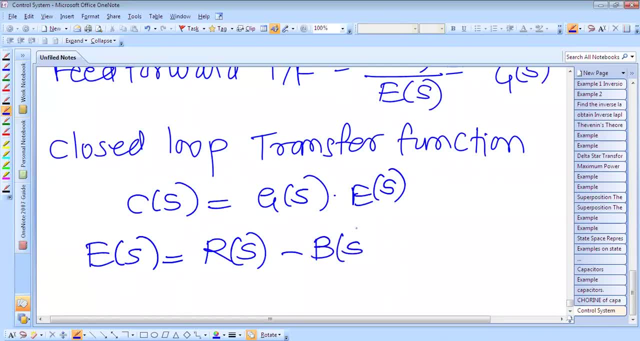 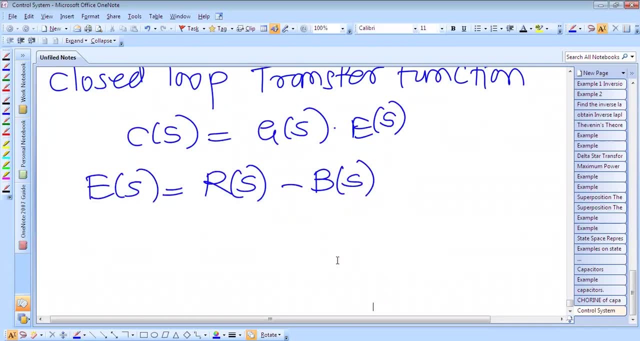 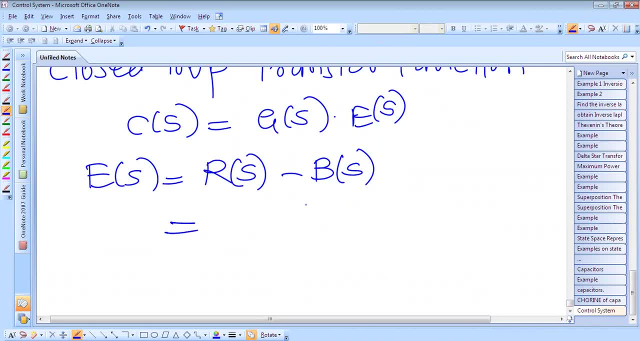 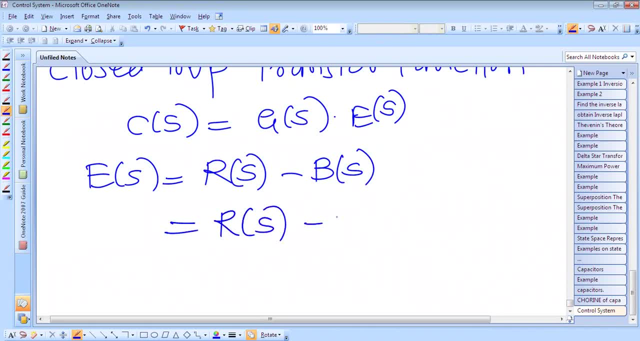 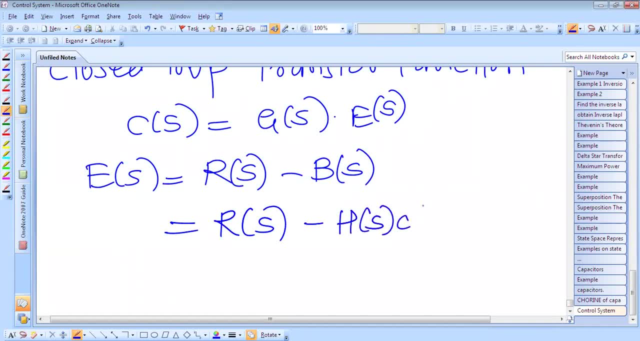 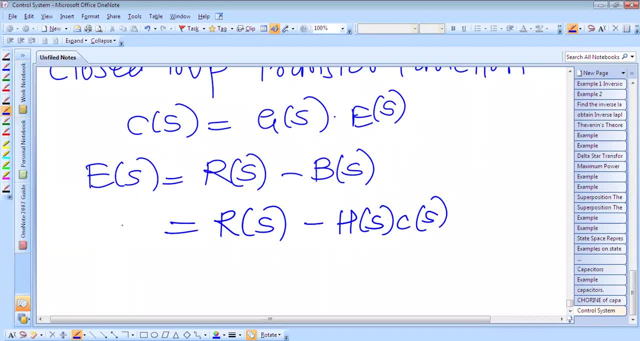 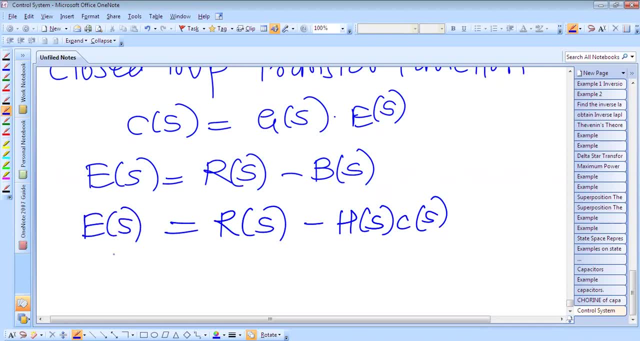 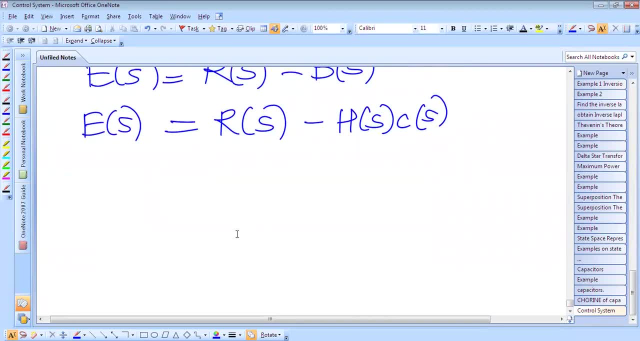 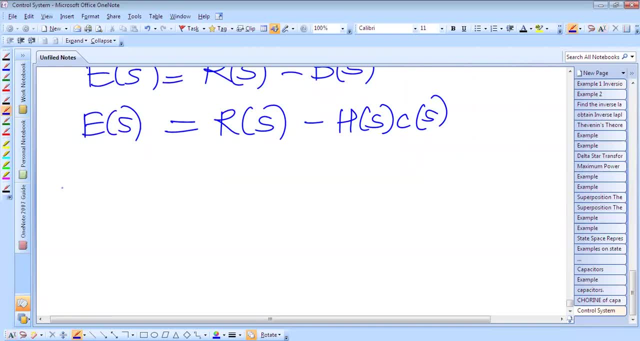 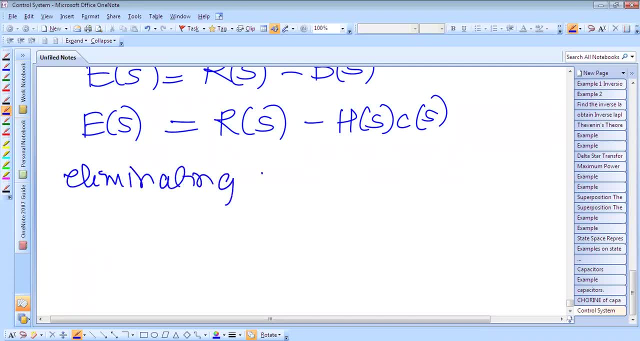 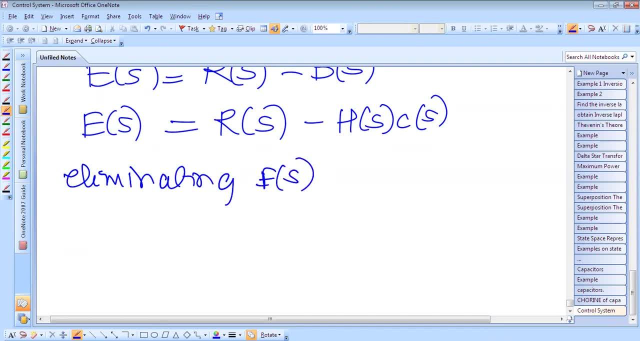 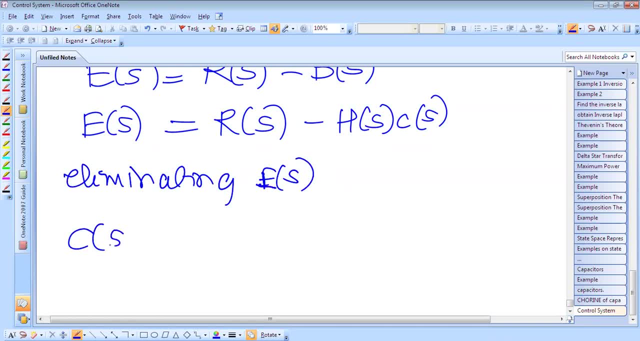 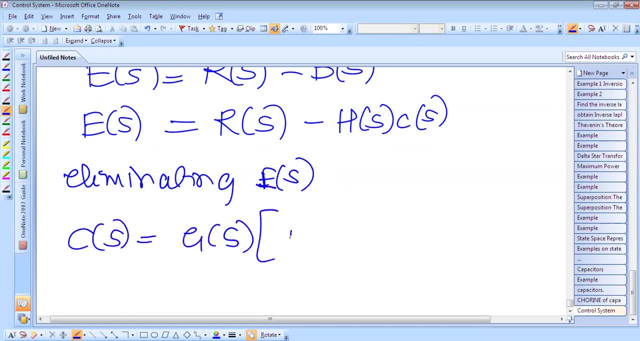 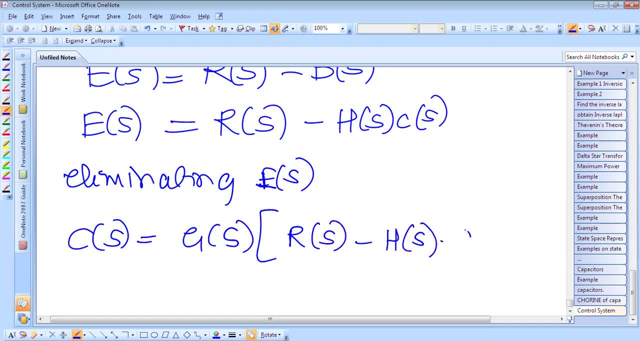 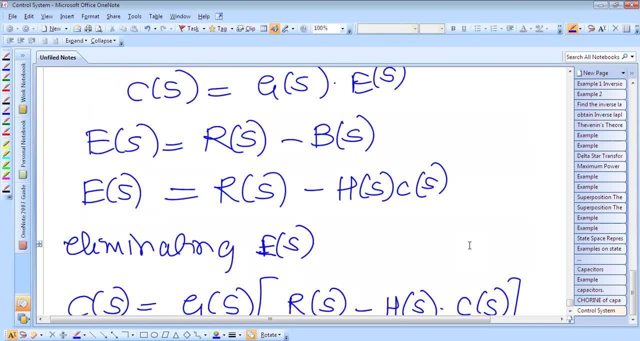 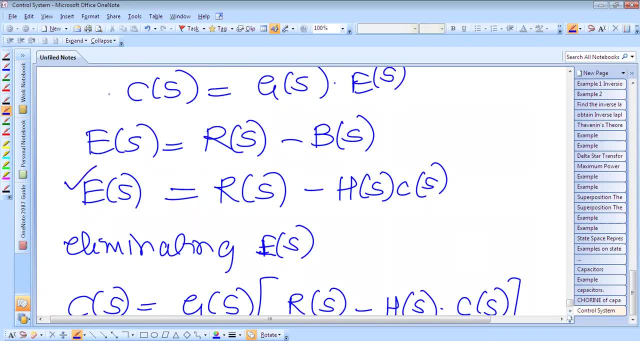 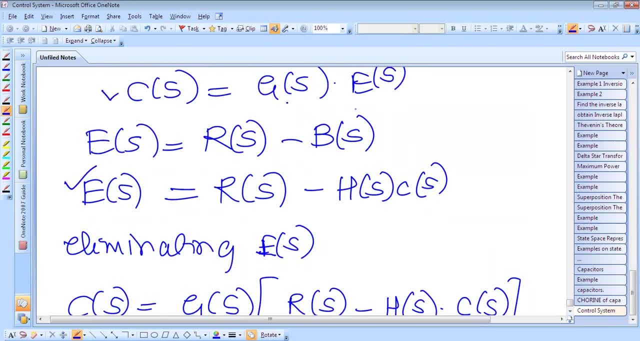 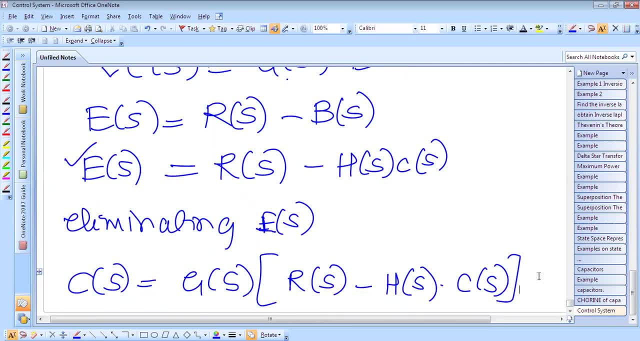 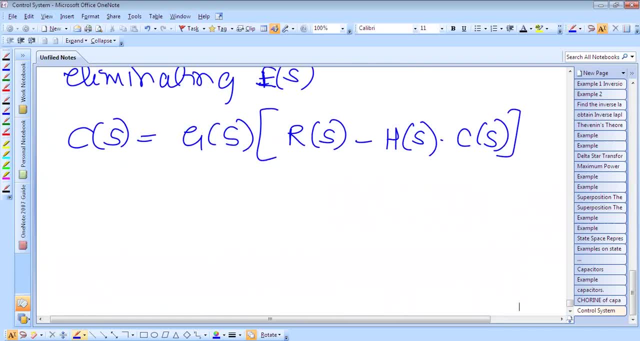 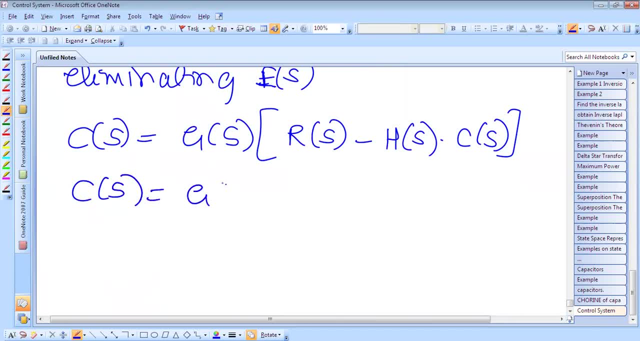 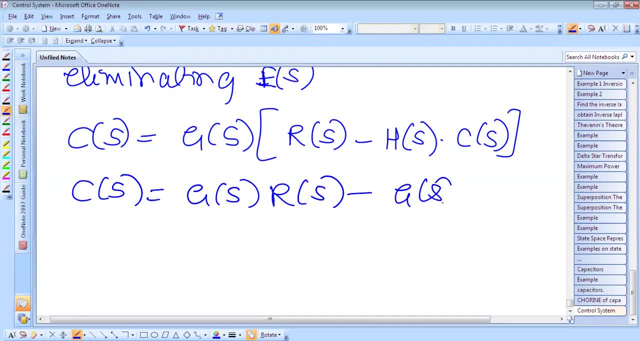 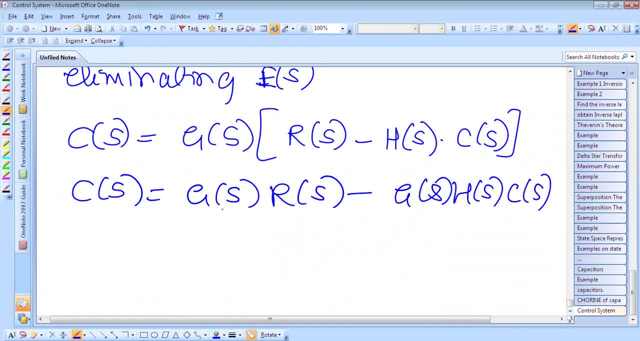 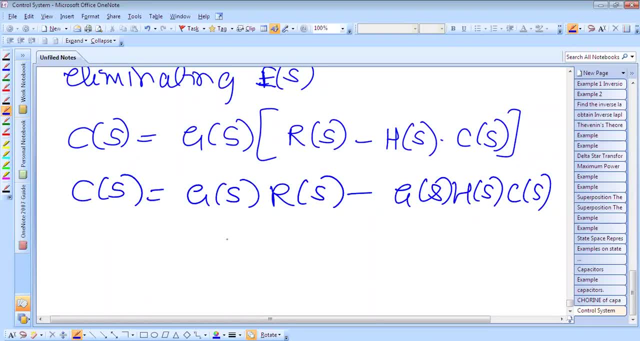 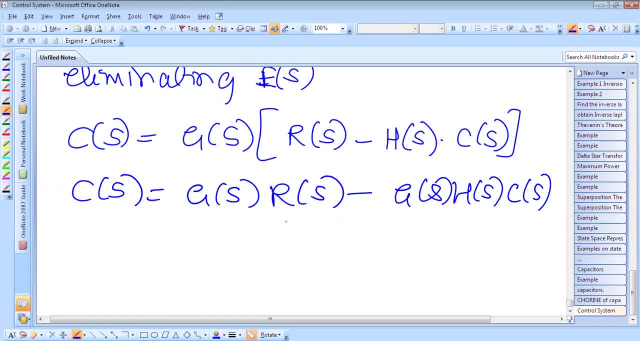 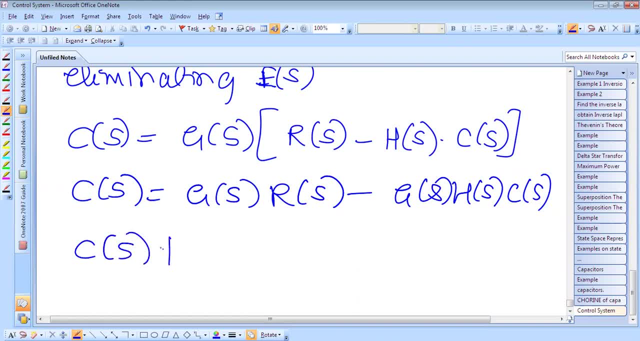 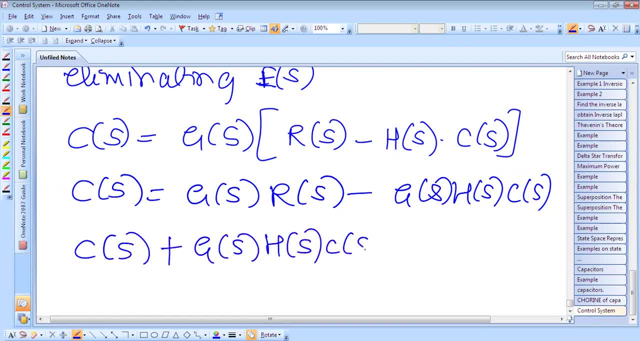 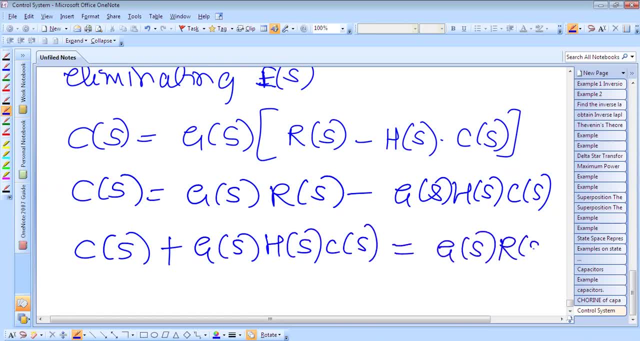 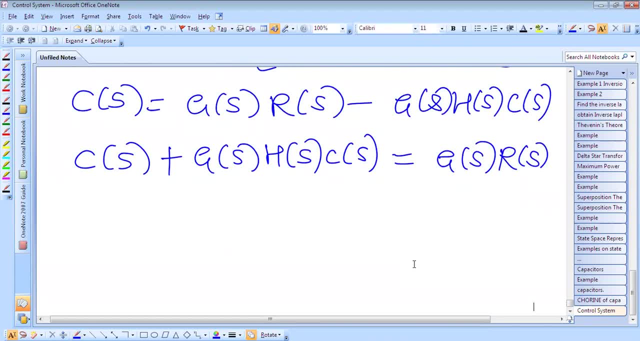 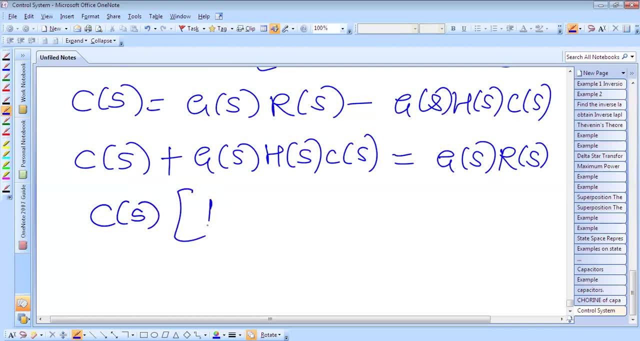 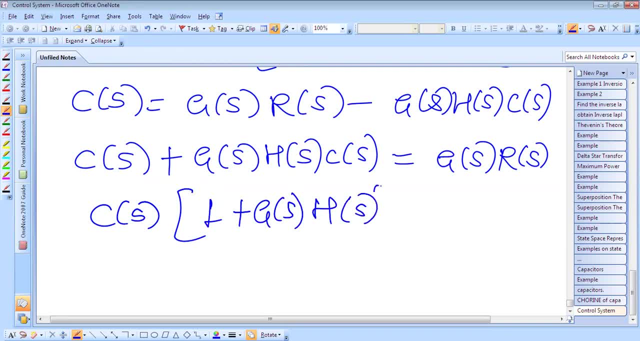 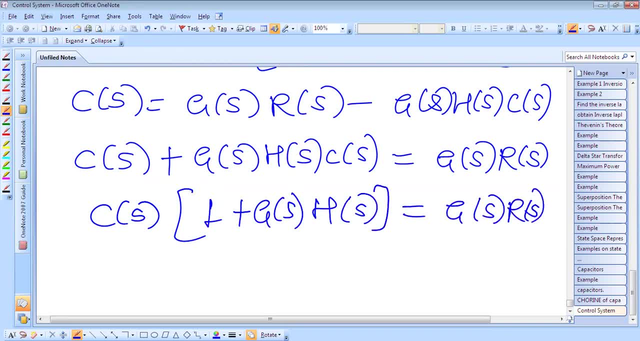 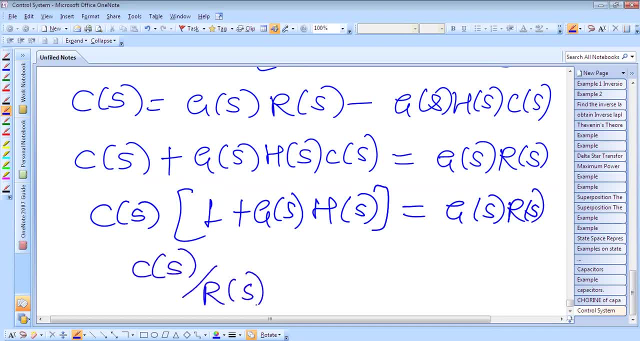 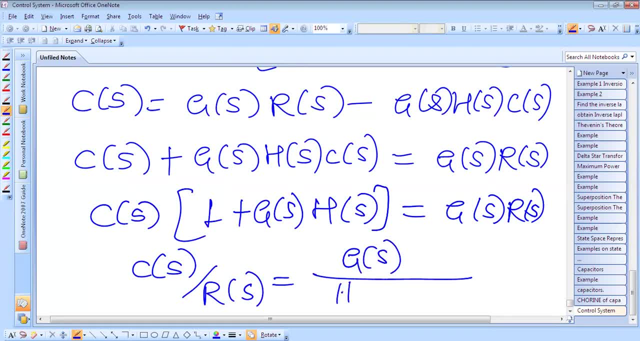 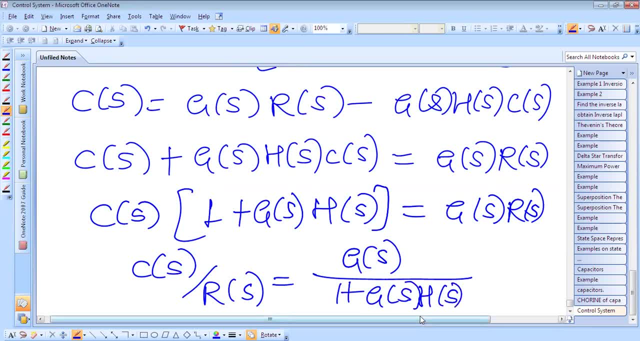 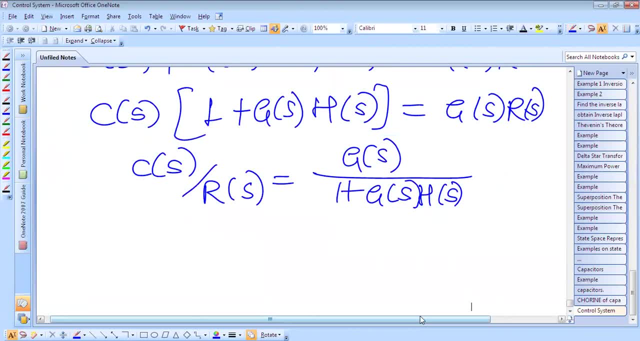 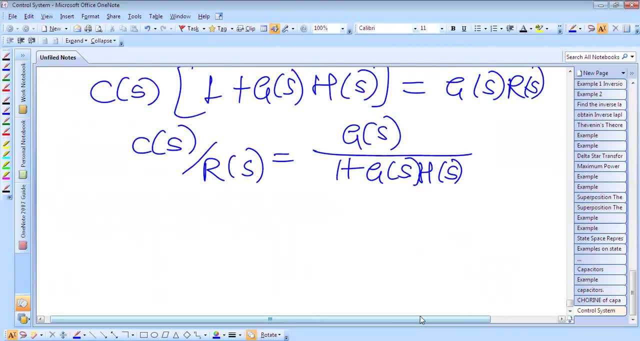 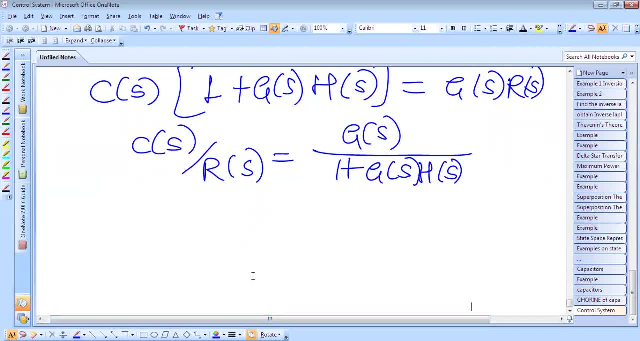 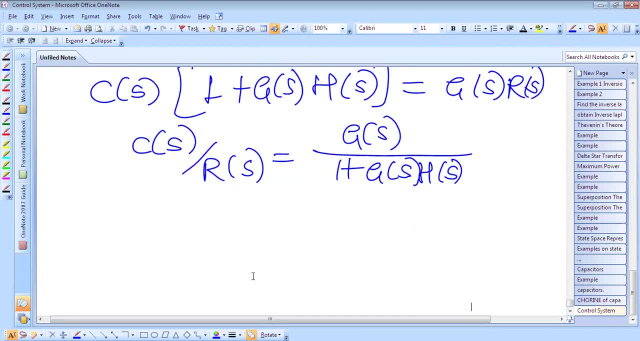 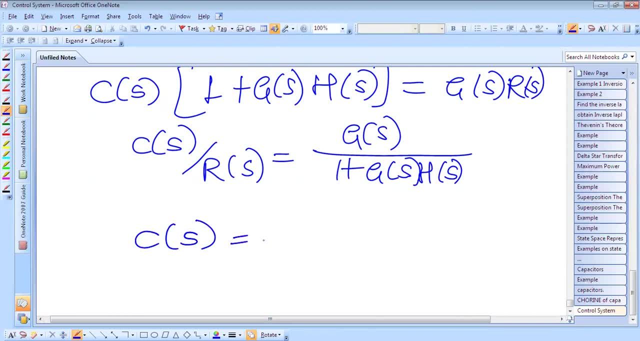 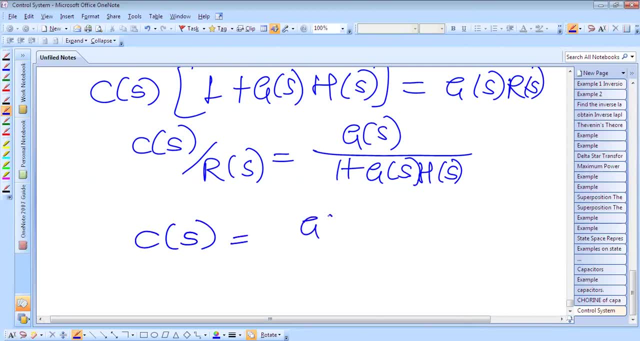 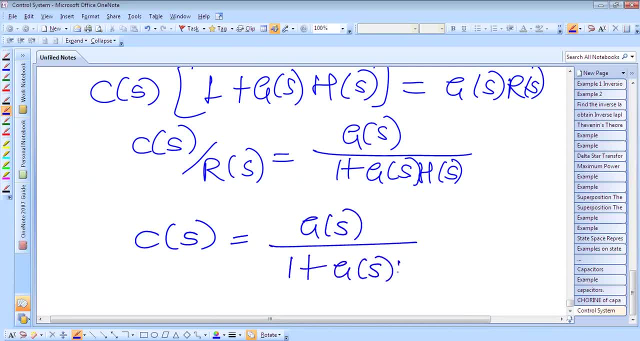 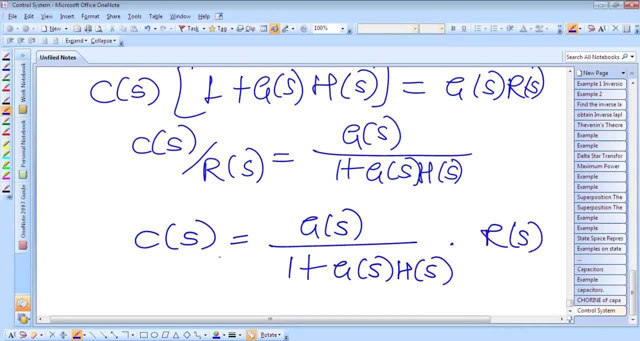 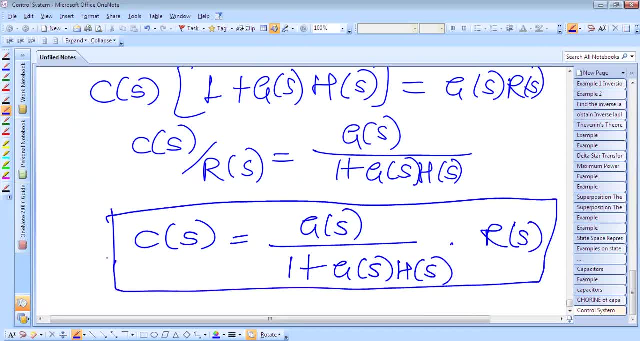 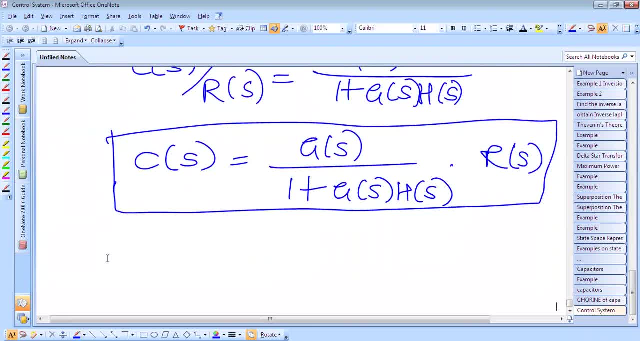 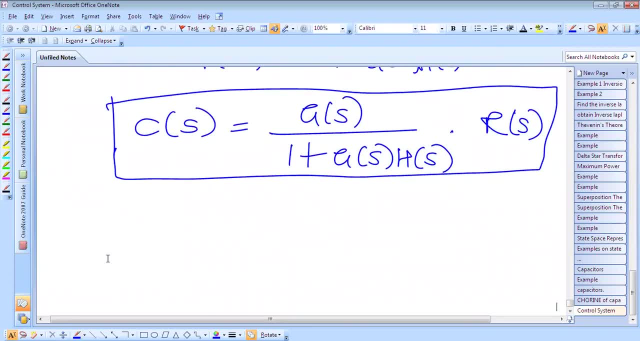 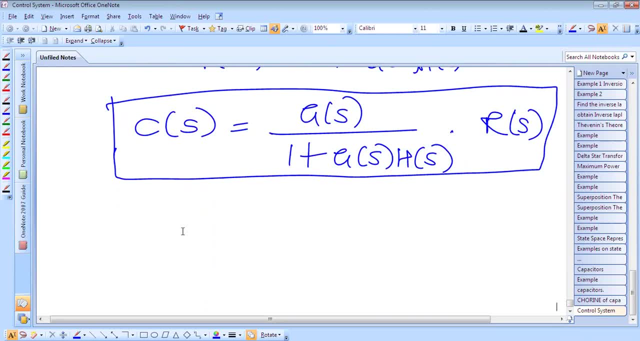 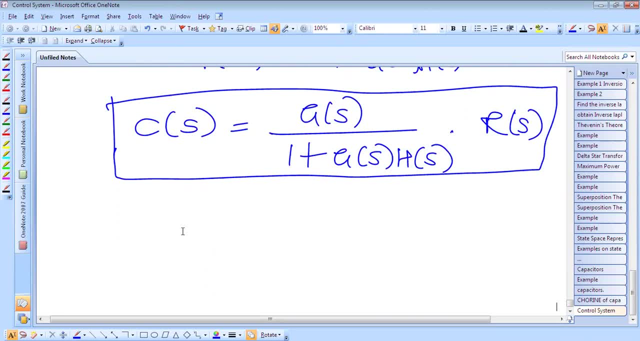 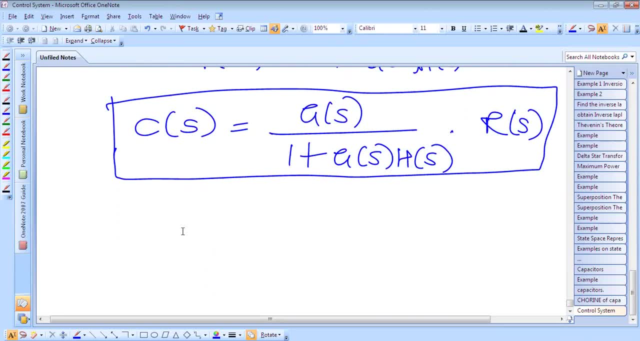 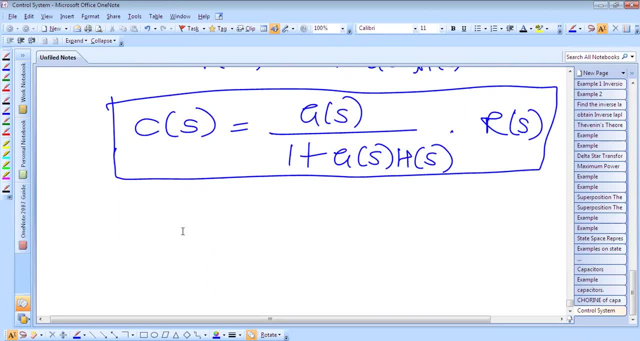 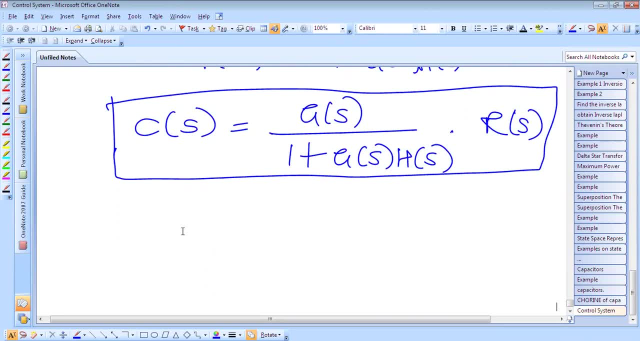 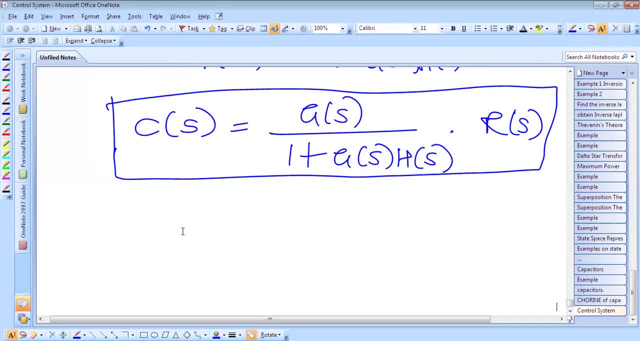 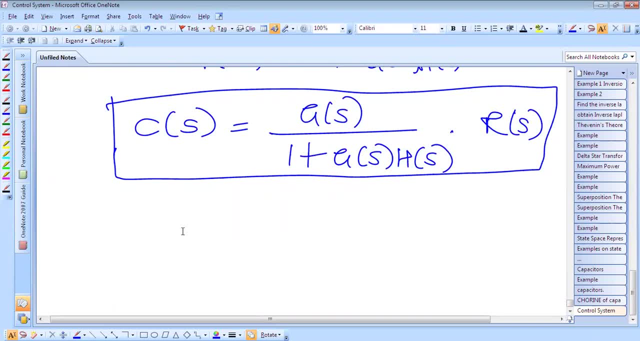 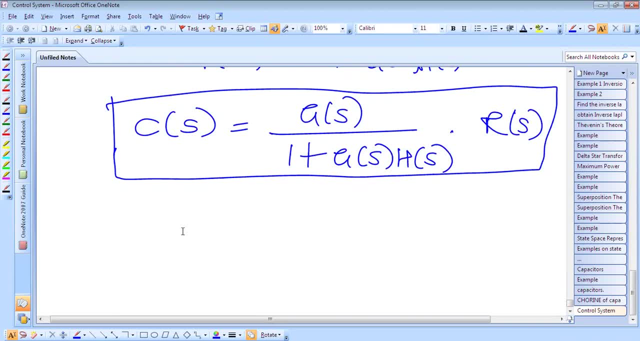 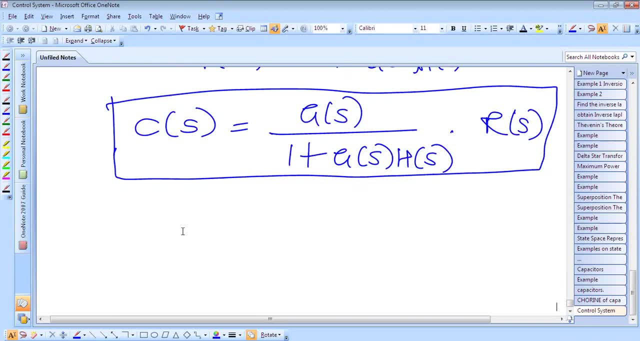 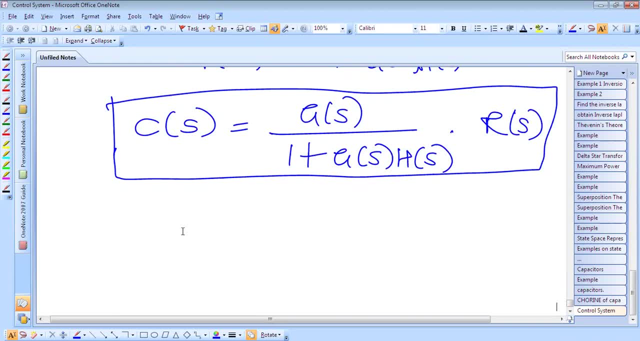 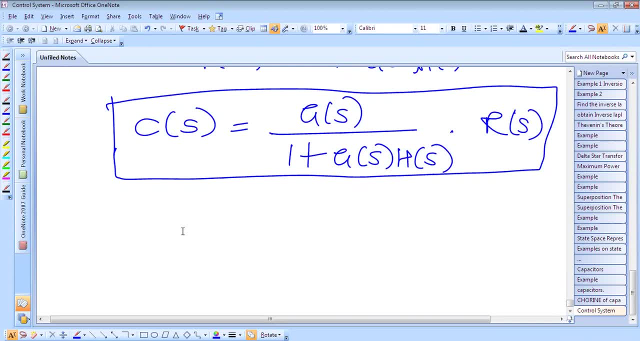 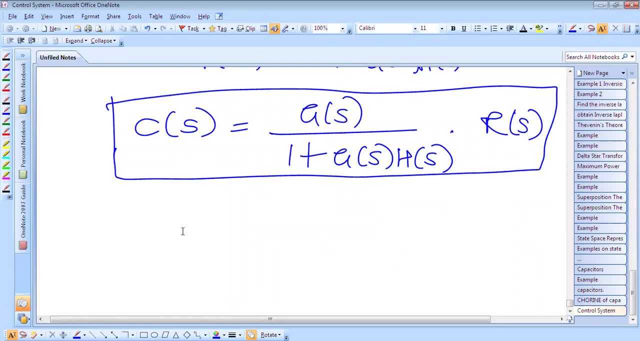 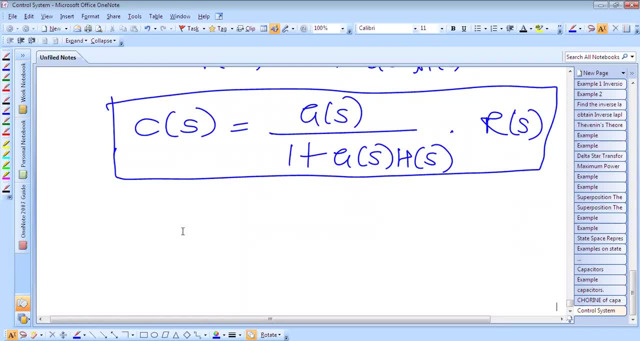 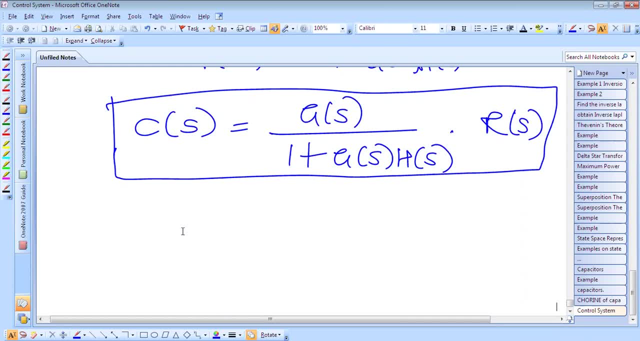 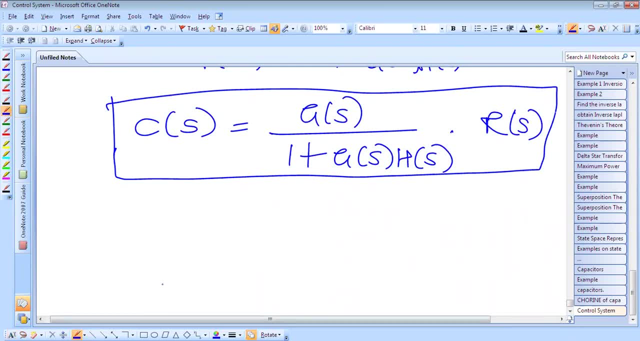 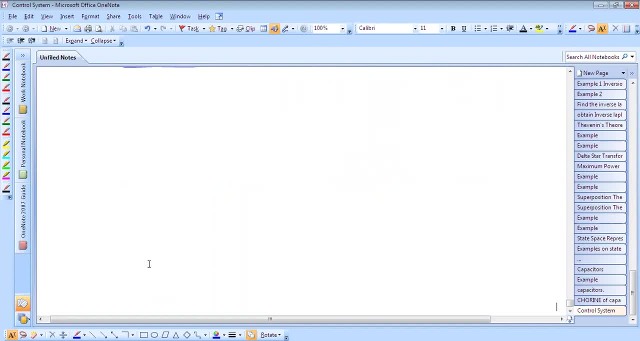 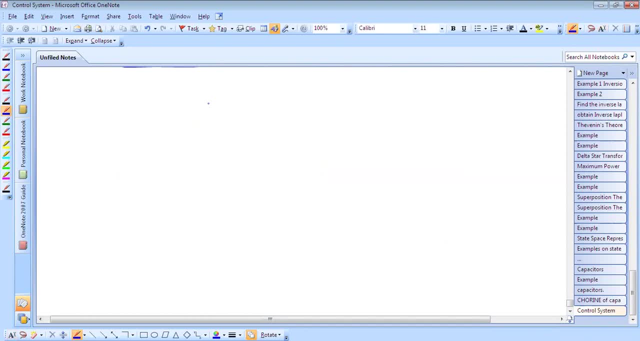 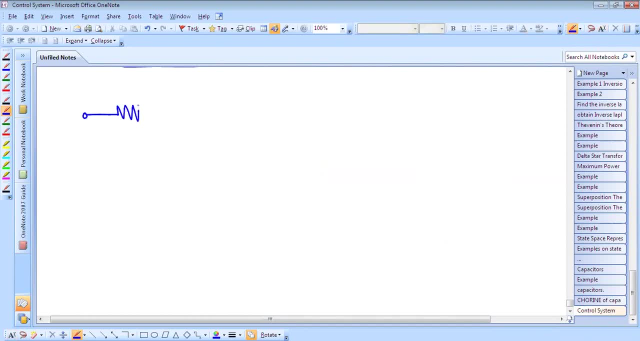 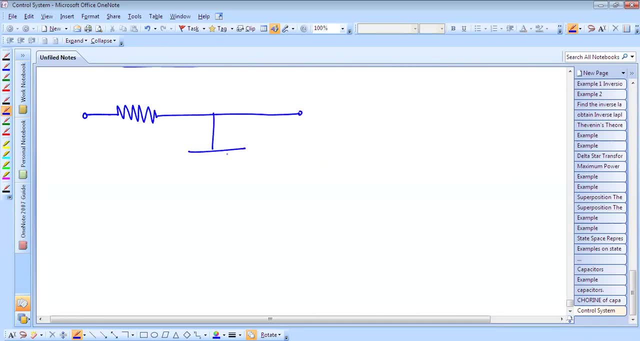 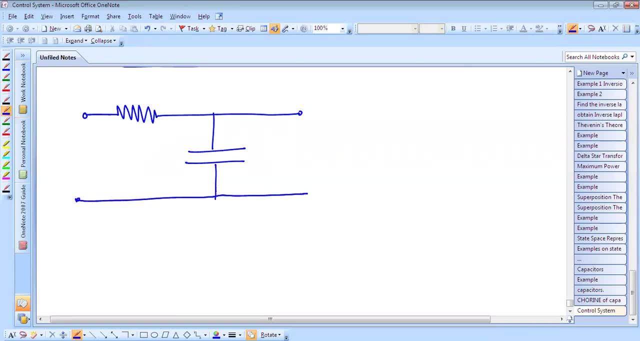 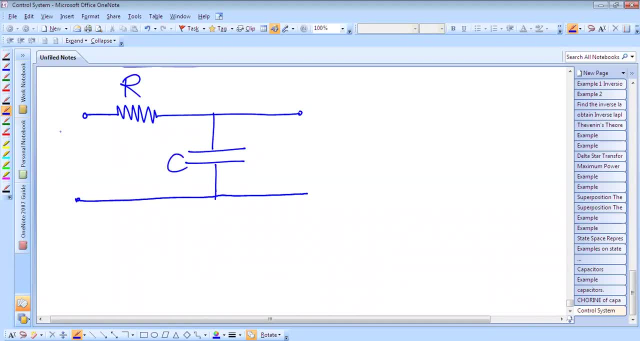 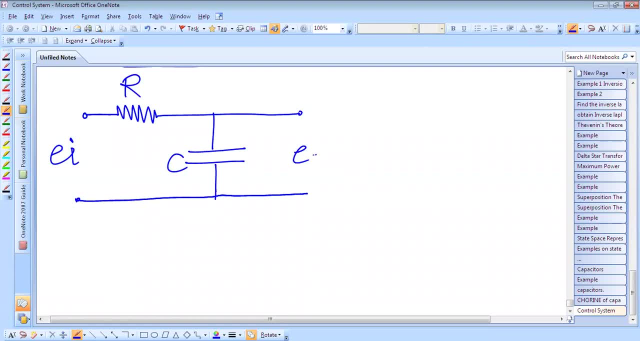 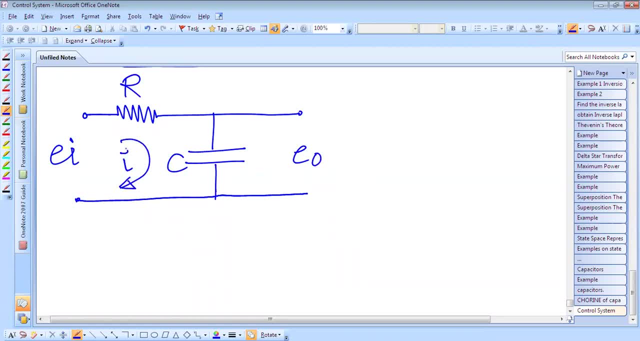 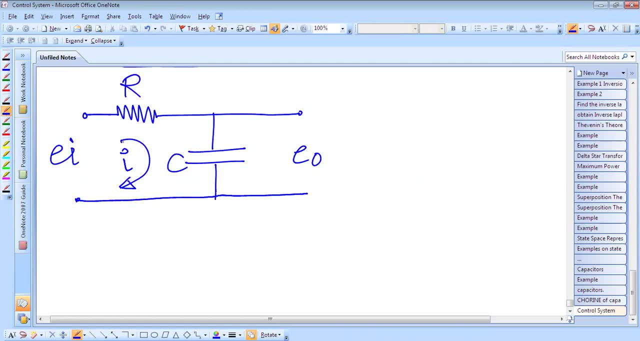 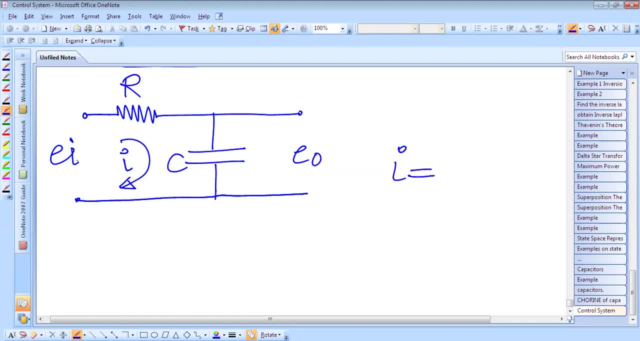 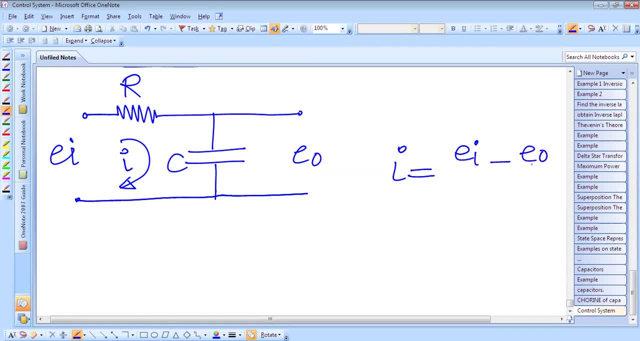 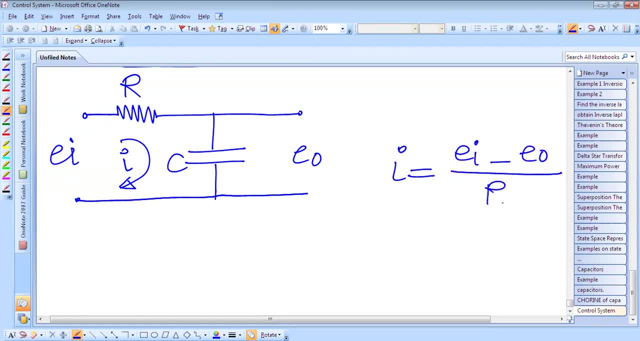 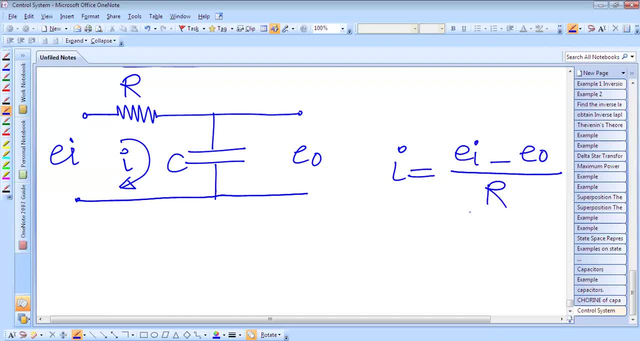 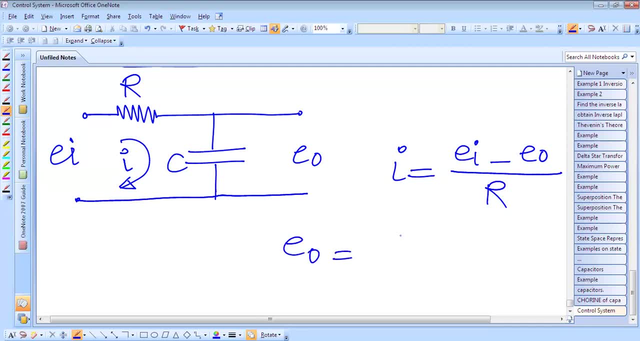 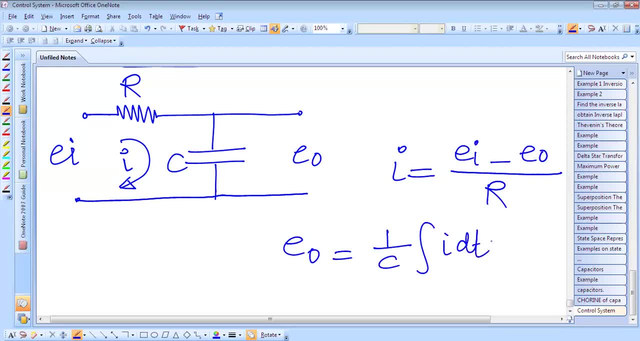 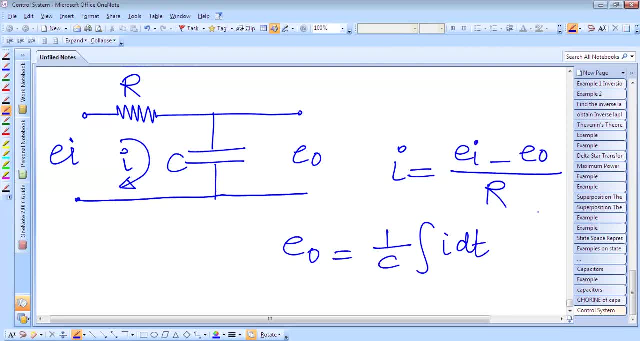 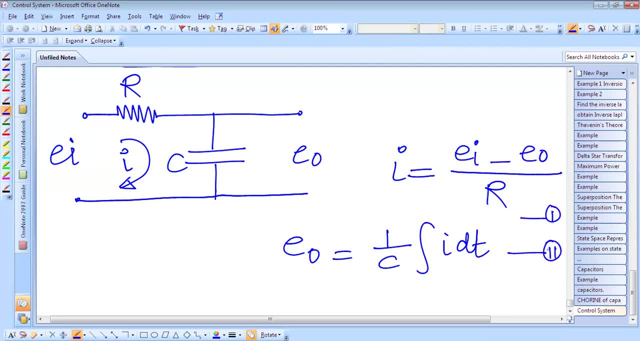 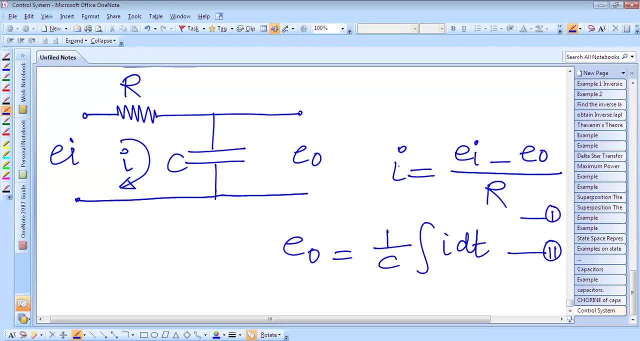 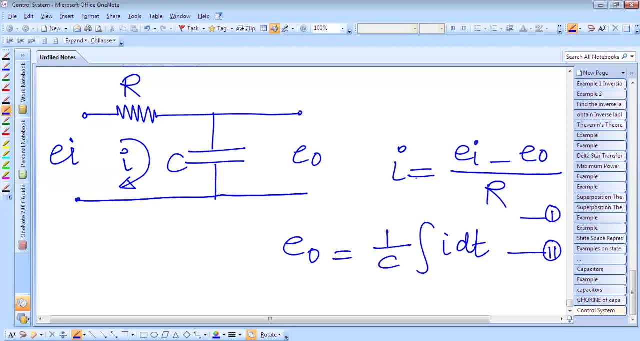 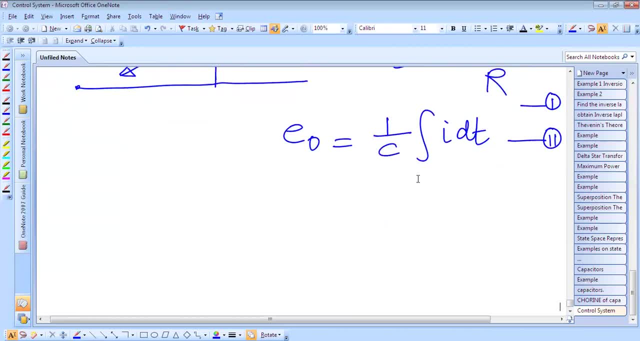 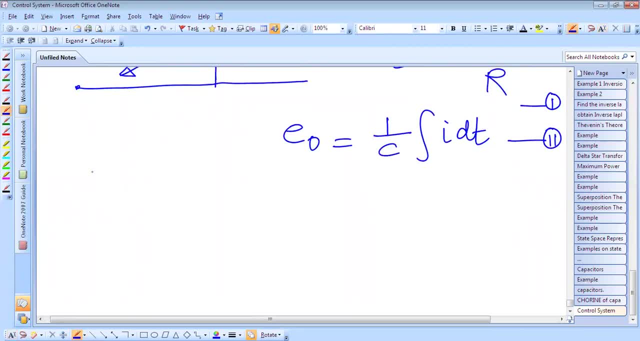 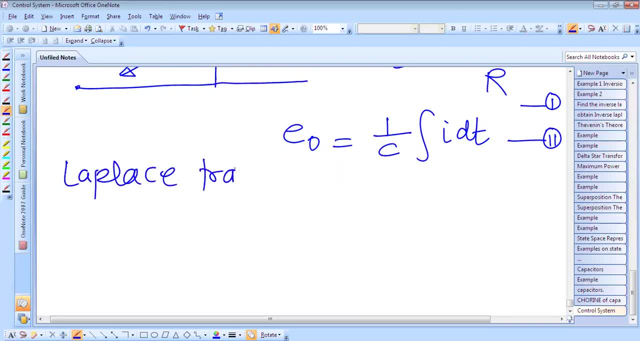 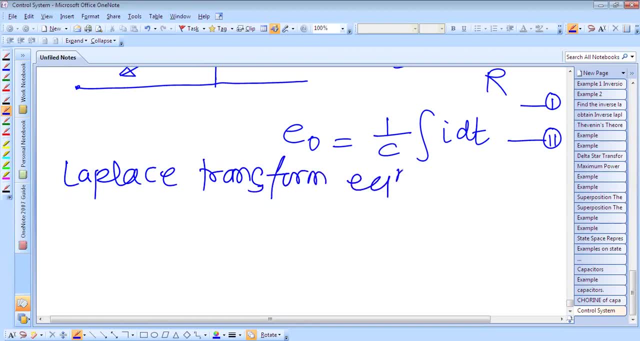 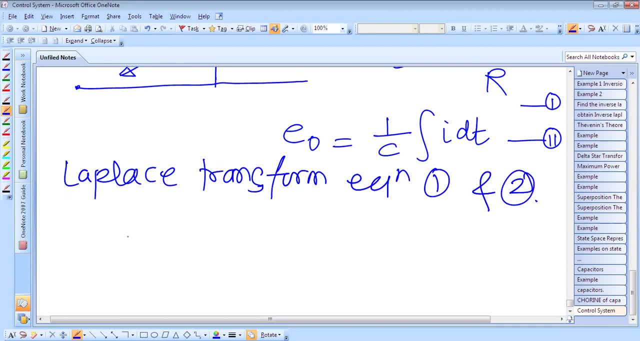 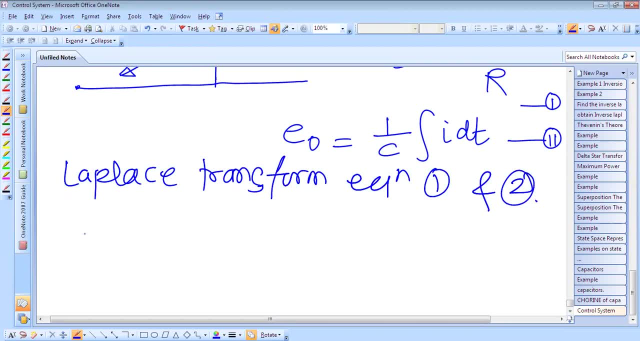 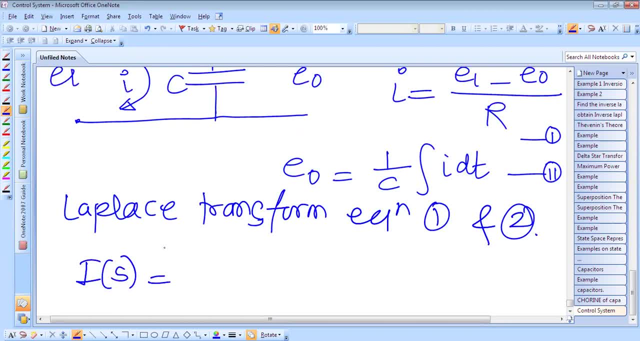 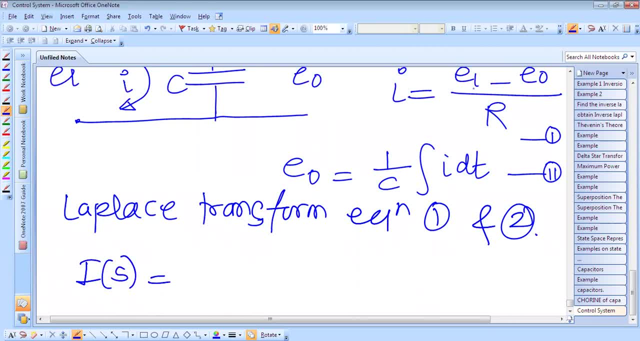 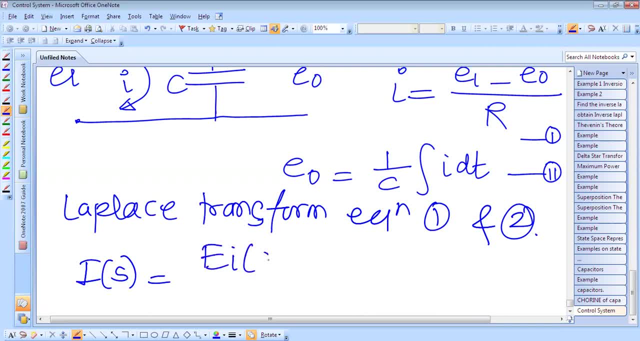 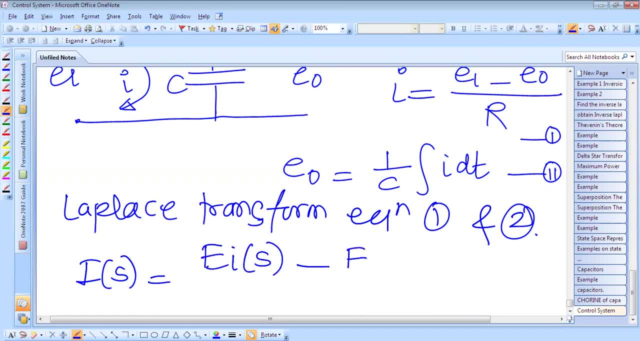 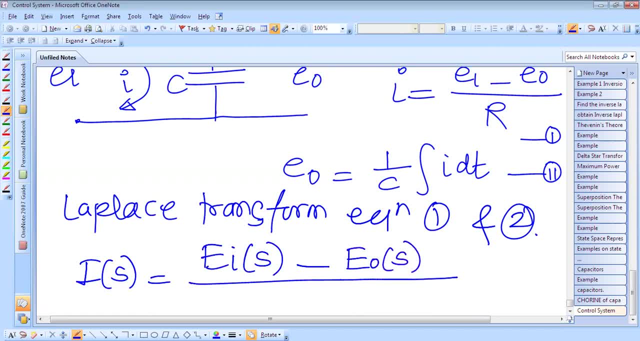 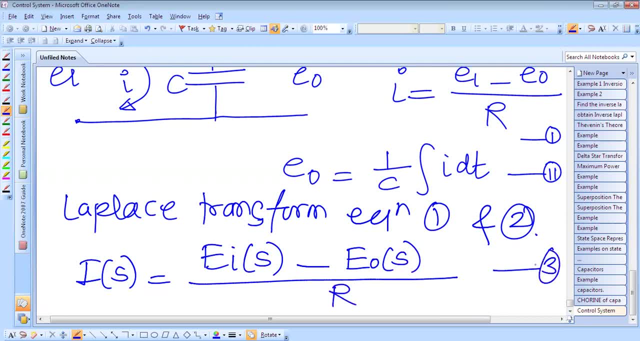 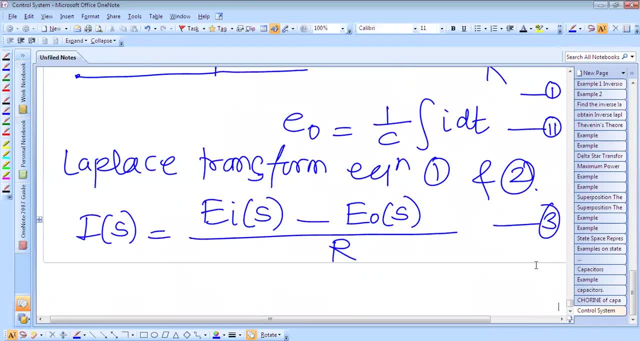 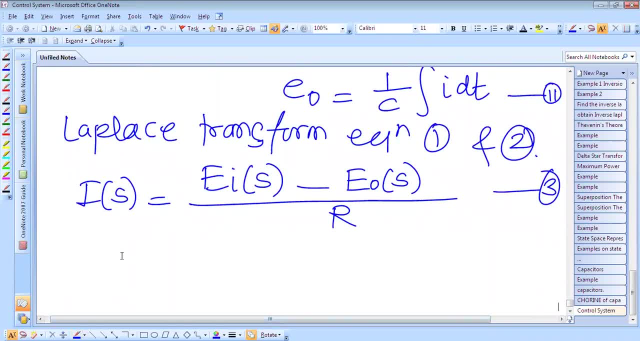 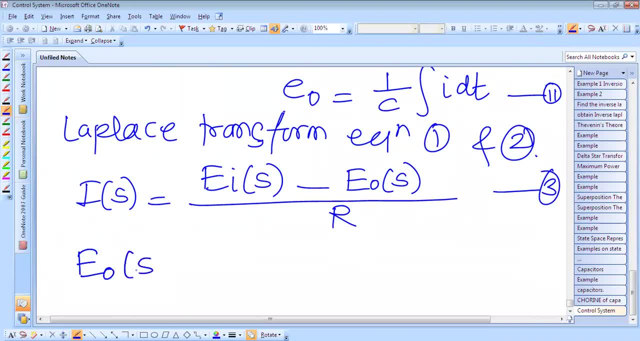 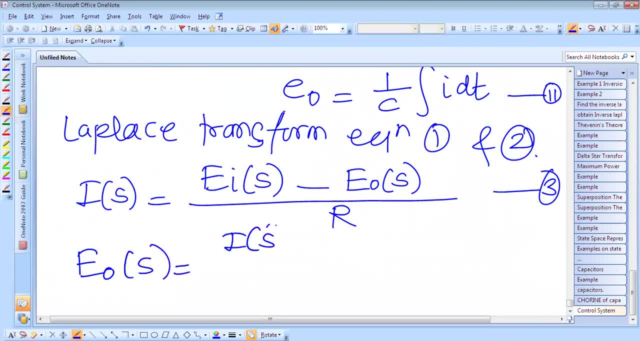 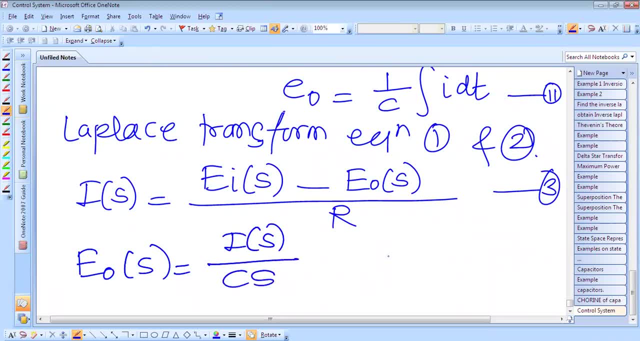 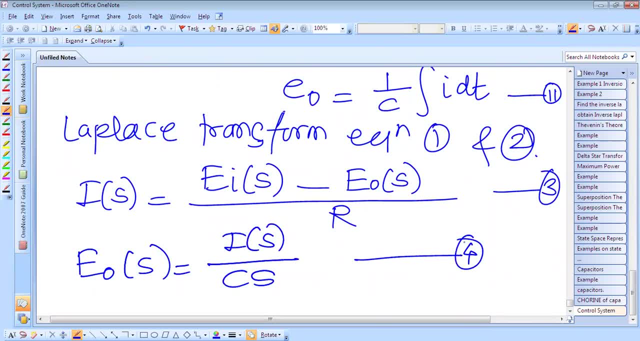 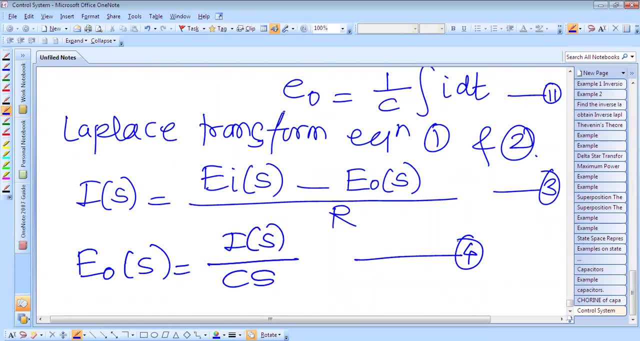 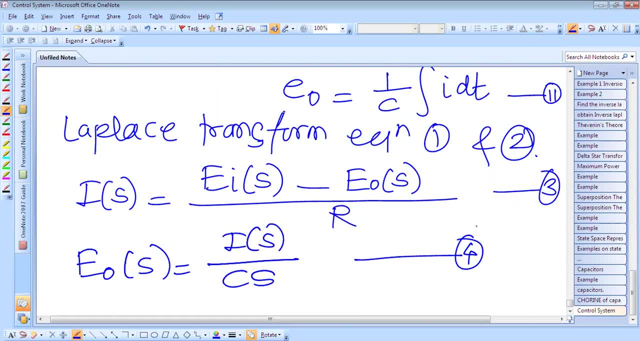 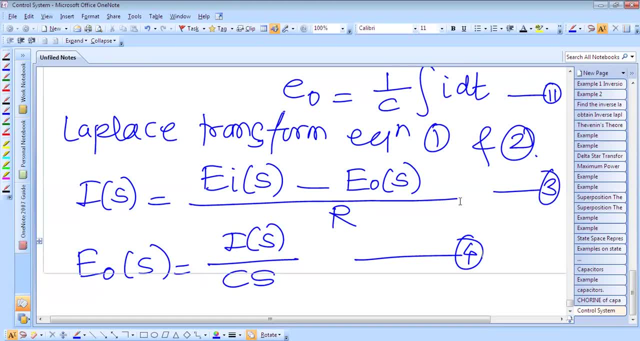 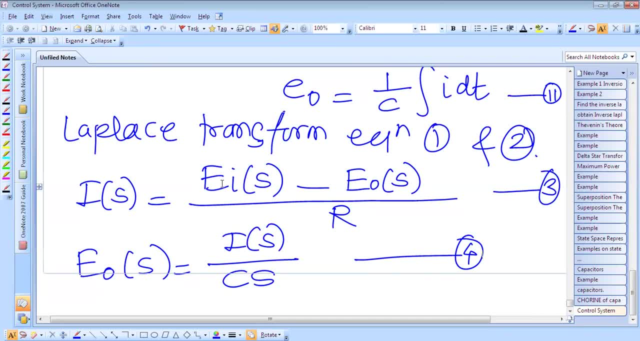 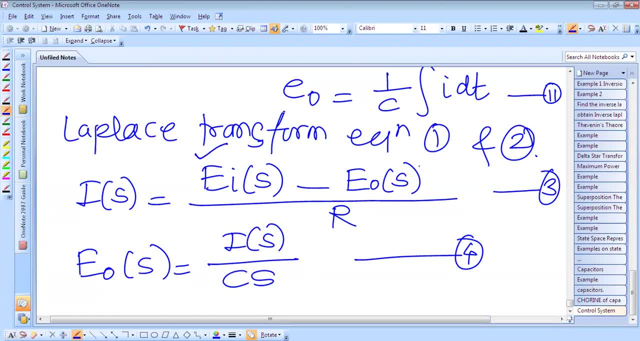 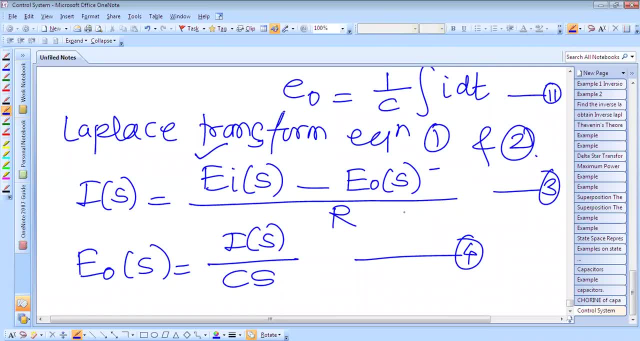 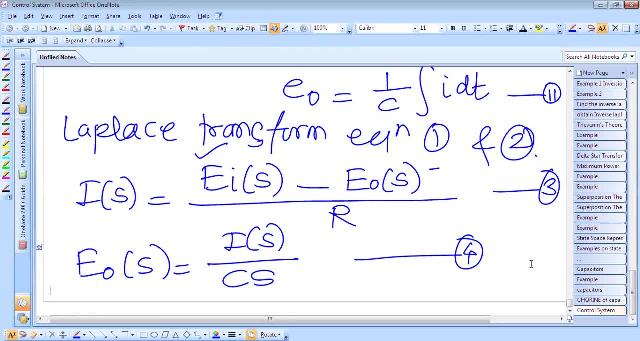